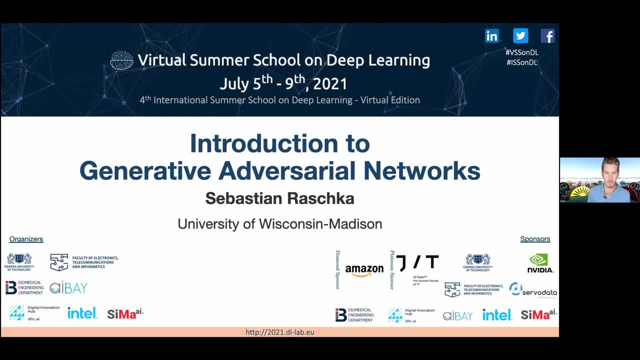 then also, I'm going to talk a little bit about the, let's say the, the, the, the, the, the, the, some code examples, because that's how I personally like to learn: I usually switch back and forth. 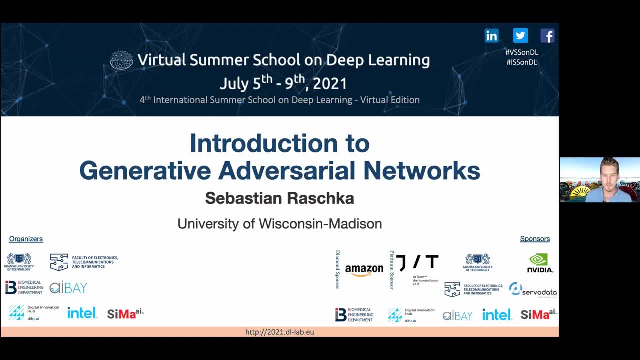 between, like looking at figures and maybe some equations, but then also looking at the code examples, and have like a mix of different- yeah, different- learning resources to help me learn a new topic. So but yes, I use iPad here with my annotations, So if I look down it may look weird. 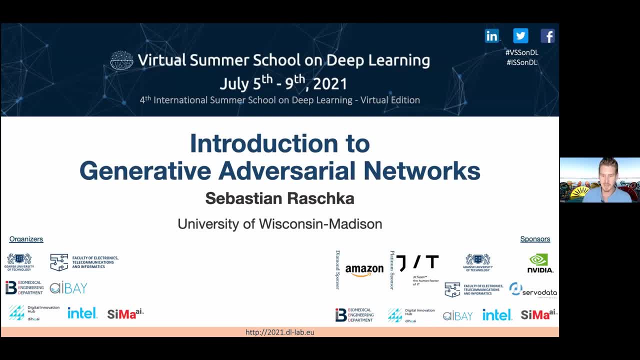 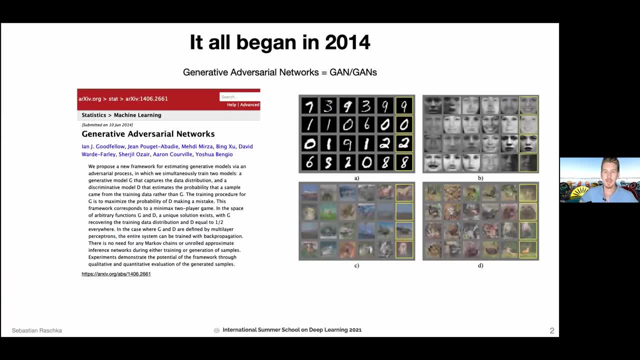 but it's kind of easier to write on this on my desk and then in the air, So I'm just trying to advance to the next slide. Okay, that works. So we will be mainly focused today on the original GAN paper, and then we will also implement a convolutional GAN. So it's called: 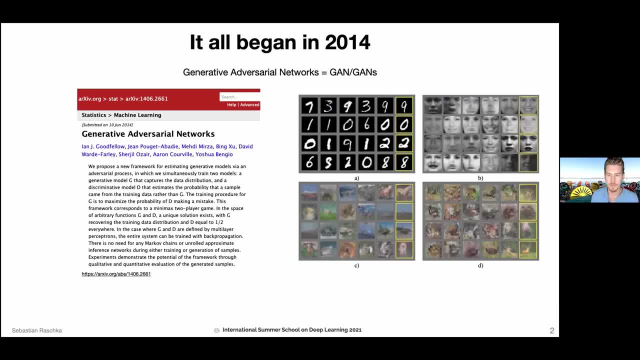 a deep convolutional GAN. It's essentially GAN with convolutional layers for image generation. So the first GAN was presented in 2014 in this seminal paper here by a good fellow and colleagues And this really laid the has laid the groundwork for all the. 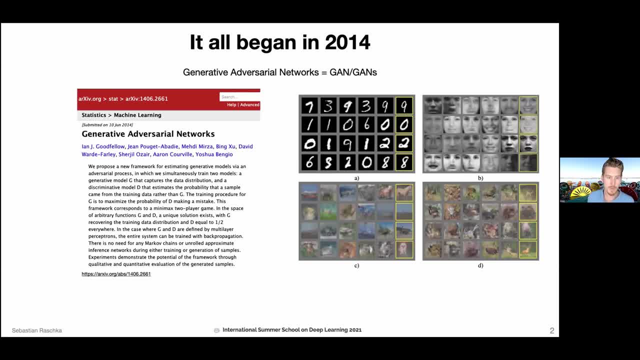 following GAN work. So 2014,. that's almost seven years ago, and a lot of things have happened since then, but still the main fundamental concepts remain the same. So in this paper here, the researchers proposed this GAN. I will talk more about the broader concepts later. 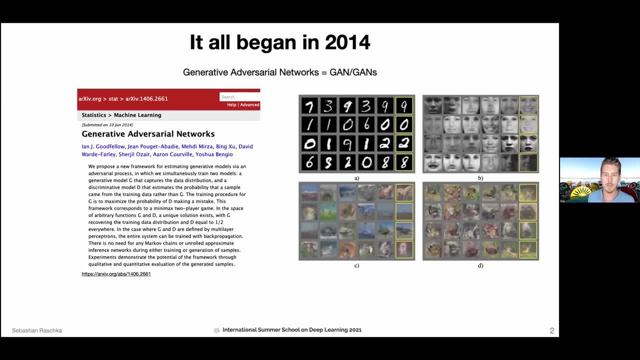 but just to give you an idea of what they did is they generated new images. So before that, deep learning was really focused more on, yeah, classification or regression problems, And this was like a new area where they generated images. So there were some related works with. 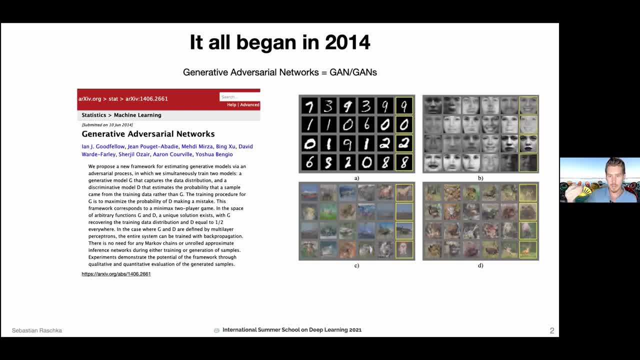 autoencoders and variation autoencoders, And I believe Alfredo will talk more about variation autoencoders tomorrow, which is somewhat related. It's also for generating images, but the generative adversarial networks, they have been really, I would say, groundbreaking in terms of generating. 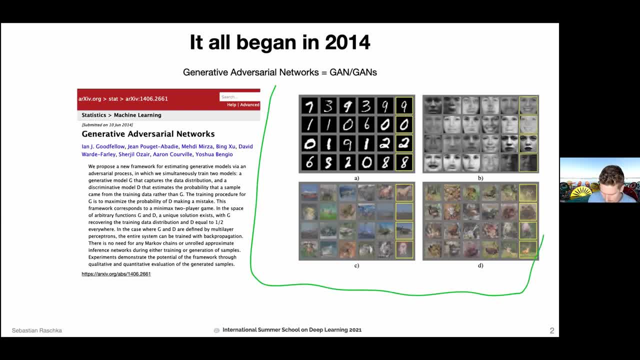 realistic looking images On the right-hand side. here I'm showing you some examples from the paper. They focused only on very- I would say very- simple data sets because at this point it was more like a proof of concept, just demonstrating that what they came up with actually works. 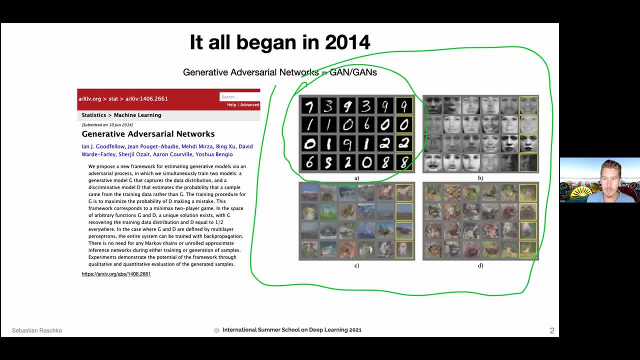 So they, for instance here, generated new handwritten digits from the MNIST data set. I'm pretty sure you've heard of this. It's a data set of handwritten digits And then also here, for example, a face image data set And you can see this is in gray scale and the resolution is. 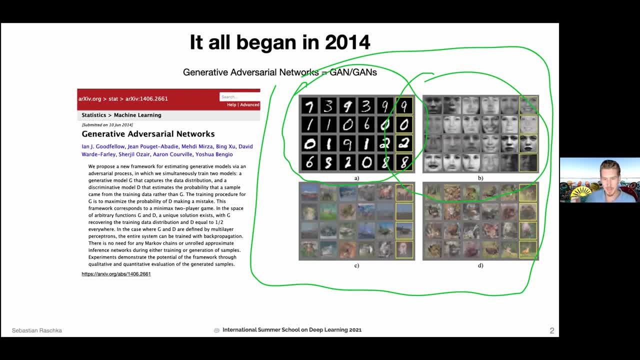 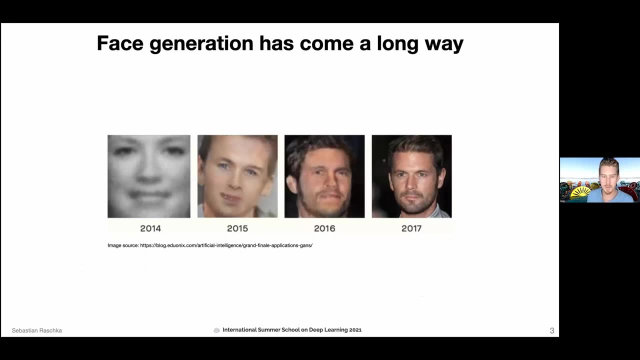 very low, but years have passed after 2014.. And researchers based on these foundations here have been making progress very quickly. So, only a few years later, people then developed these generative adversarial networks with better capabilities of working with higher resolution images. So in 2014,- 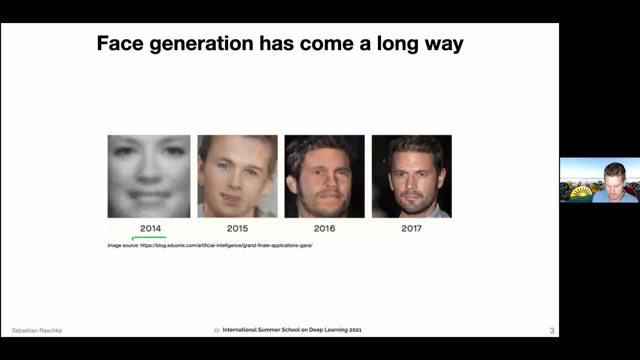 we still had these gray scale low resolution images 2015,. people worked with color images 2016,. the quality of these generated faces became better And this is 2017.. It's also four years ago, but even four years ago, people achieved really impressive results. where here? 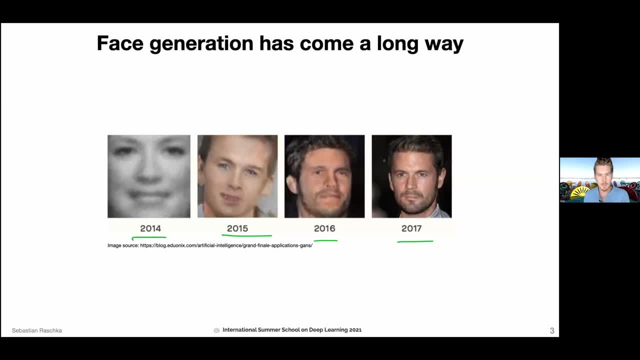 I'm showing you face images of people that don't exist in the real world. So these are all face images that have been imagined or created by this generative adversarial network. So they are images that don't exist, which makes this kind of impressive. So, moving on, of course, 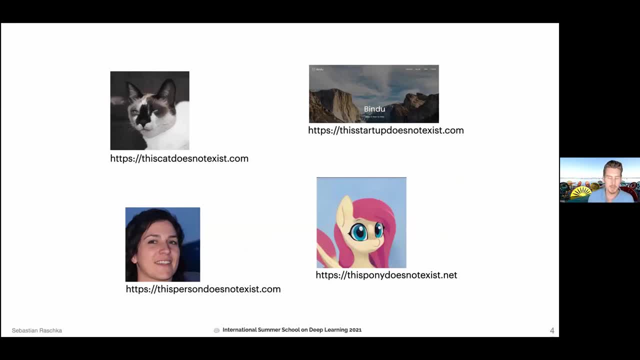 it's not all about face images. That was just one example. People nowadays use GANs for all kinds of things, So there are these fun websites where you can, for example, go to this website. This cat does not exist, And every time you refresh the page, it will create a new cat that does not exist. 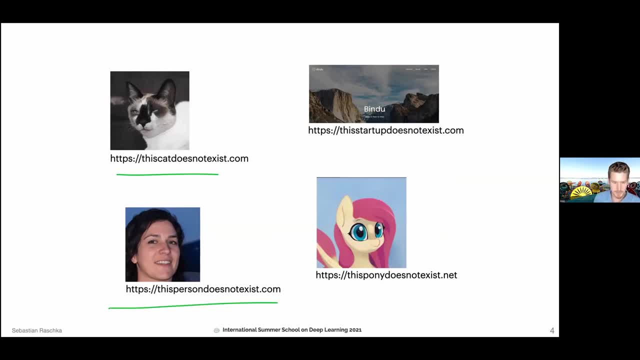 in real life Or this person does not exist- website which is generating these face images And behind the scenes, when you go to these websites, they are all using GANs- generative adversarial networks- to generate these face images And you can see here that the GANs are. 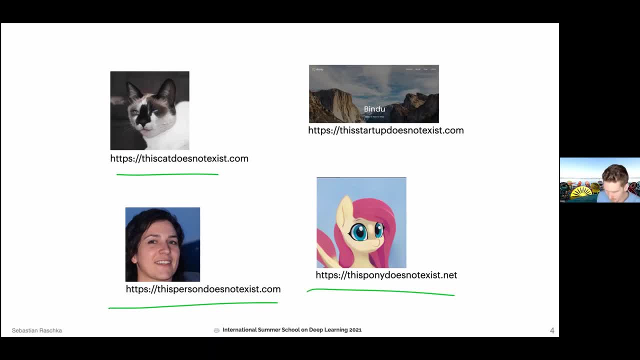 generating these images. Well, if you prefer ponies, there's also a website for ponies. And if you ever think about starting a startup and you are lacking, maybe, the ideas for coming up with a catchy name or logo, there's also a website for this startup that does not exist. 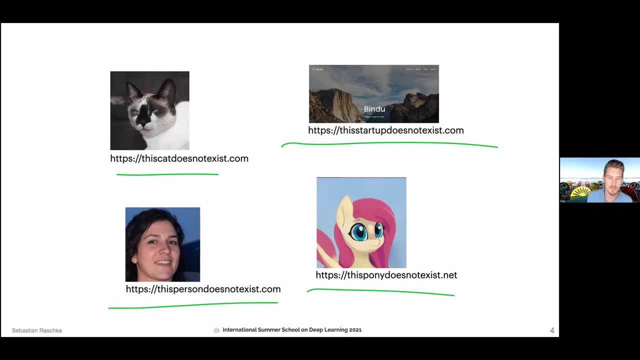 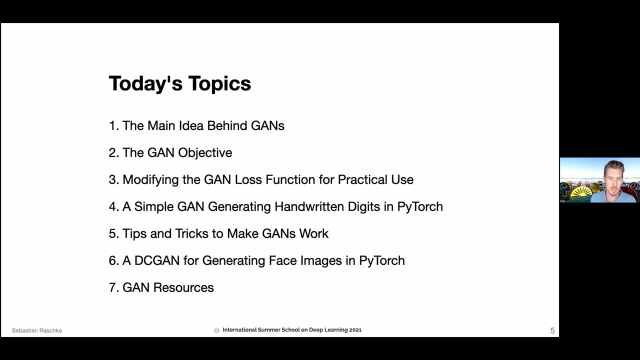 Of course, these are more like joke applications, but now in the real world people use GANs also for many medical applications, So it's a very, very interesting concept. So how we are approaching this lecture today is that today I will start by introducing the 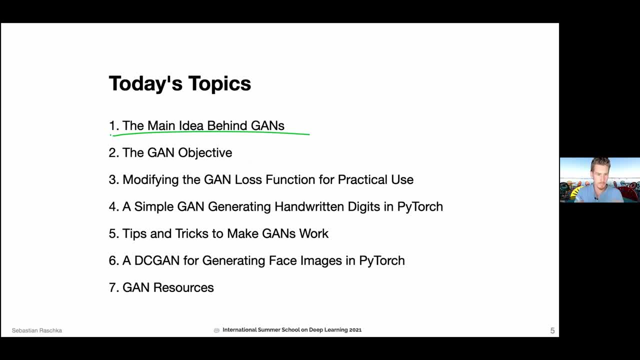 main idea behind GANs. I've just shown you some things that a GAN can do, but I haven't explained how that works yet. So I'm planning to go over the broader concepts, how the GANs work. Then I will talk a little bit about the GAN objective. 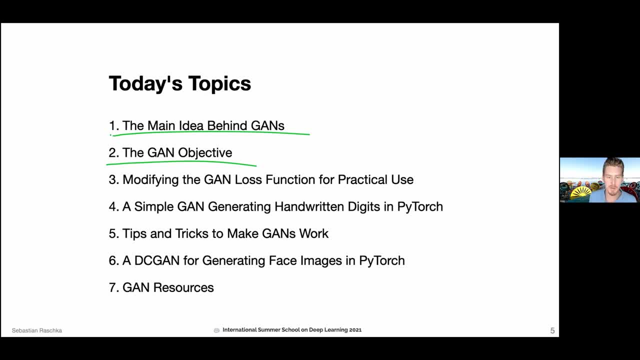 a little bit about the mathematics behind the GAN, but only very briefly, But it's kind of like a fundamental thing that you need to know in order to implement a GAN, So we will talk little bit about that. modify this, then, to make this easier to implement in common frameworks. 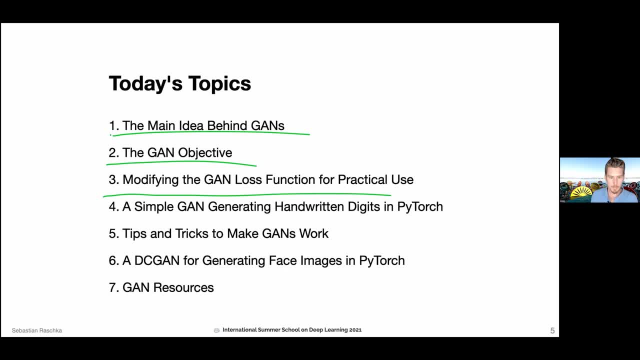 such as tensorflow and pytorch, and then we will implement our first game. so we will implement the fully connected again, again with fully connected layers, like they did in the original paper, and then we will generate handwritten digits and we will be looking at code in pytorch. i will have a 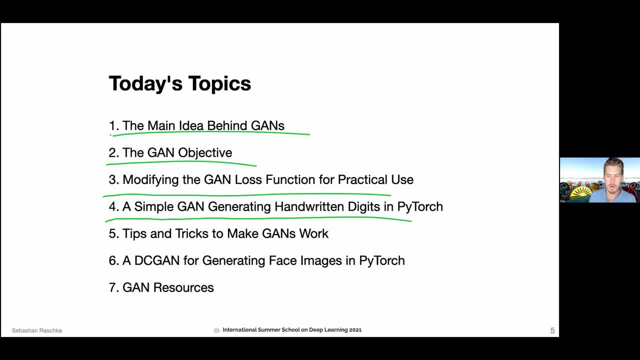 few exercises then for you so that you can also um toy around a little bit with the code. but yeah, of course we only have so much time, so it will be a short, 10-15 minute exercise by you. um, yeah, do some little. um, yeah, looking at the code and playing around with it, and then um, after you've seen the 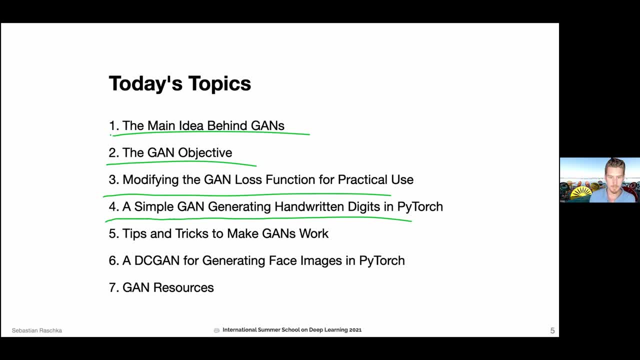 code and you have a feeling of how that looks, uh like when we implement it. i will show you some tips and tricks to make gans work well in practice. so just a few, um yeah, things to consider, and then we are looking at dcgans. so dcgans. 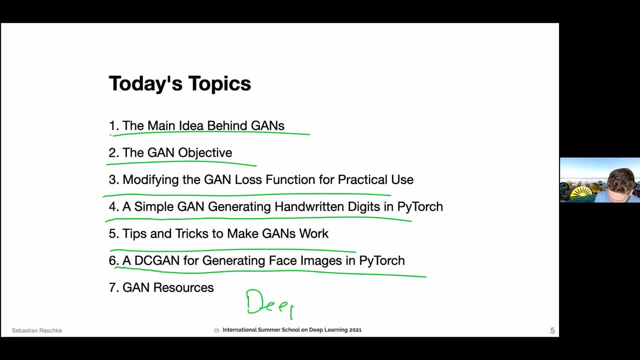 for deep, deep, convolutional again. so it's again with convolutional layers. so here, um above, we only look at the simple case and then we modify the scan to be better at generating images using convolutional layers and we will be then working with face images. i will show you the code examples. but yeah, this is uh something that. 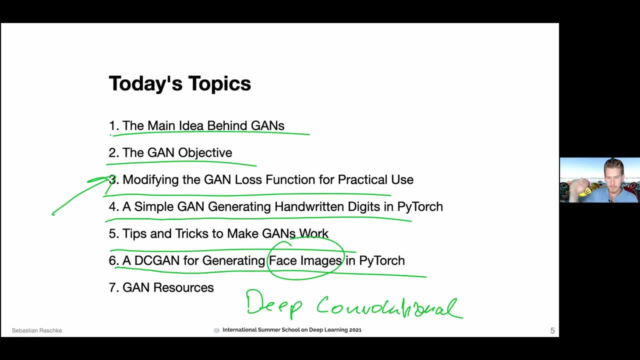 takes a long time to run several hours, so we will only look at the code examples. but, um, if you're interested, i have everything on github and also links that you can then also run this by yourself later and tweak it if you're interested. and then, last but not least, 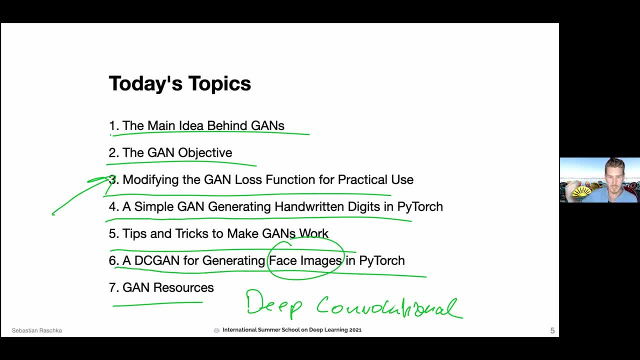 i will show you some um useful resources if you want to catch up with the latest gan literature. there are a few selected resources that you might find helpful, and i will also outline some of the other gans that exist, but of course there are hundreds of different gans. i 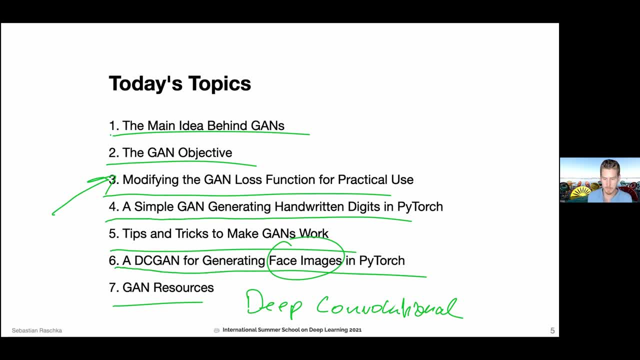 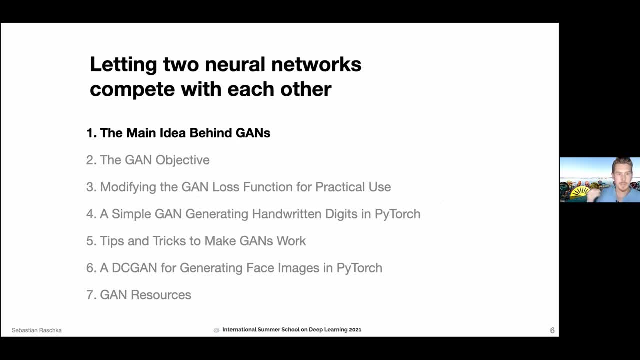 cherry picked, one of some of the most, i would say, fundamental ones. all right, so then, to get started, let's talk about the main idea behind games. so it's essentially about letting two neural networks compete with each other. so we have two networks and they- yeah, they- play this kind of adversarial game where one um one wants to. 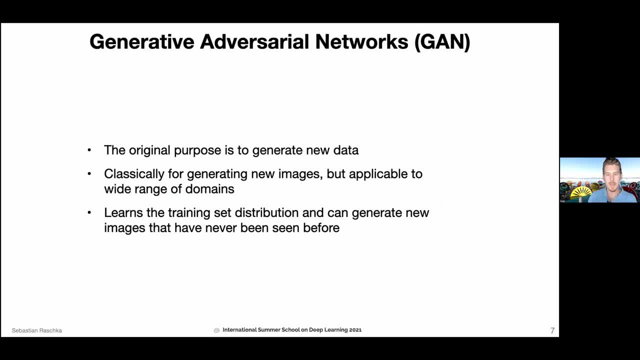 generate new images and the other one has the task of telling a part whether an image is generated or not. so the original purpose, like i mentioned earlier, is to generate new data and classically this was developed for generating new images, but of course it can also be applied to other domains. 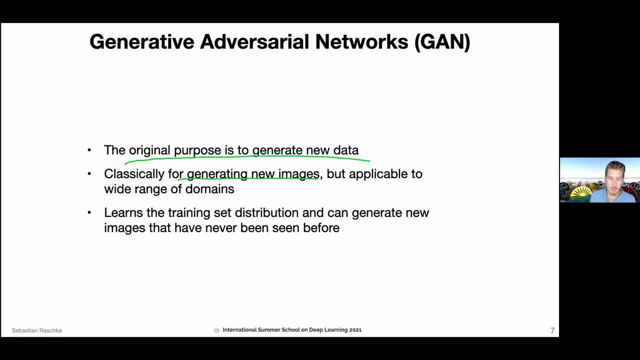 so um, for example, i also, um, like yetzik mentioned, i work on problems related to computational biology and one example there would be, for example, to create new molecules. so we can also develop gans for, let's say, graph structured data to create new molecules, or you can also. 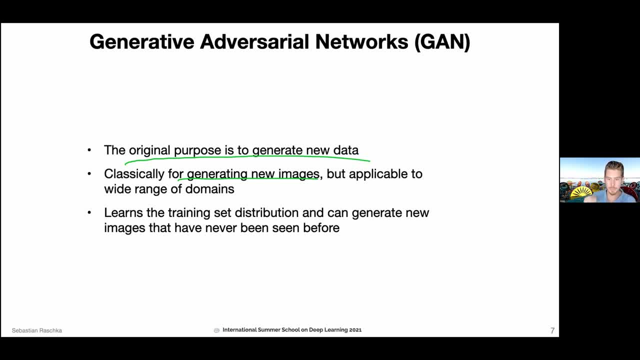 think of more in more general, just generating new types of data. why is that? um the example of images so popular, i would say it's um. one of the reasons might be because it's easy to look at images, so if you generate an image, you don't have to be an expert in whatever data. 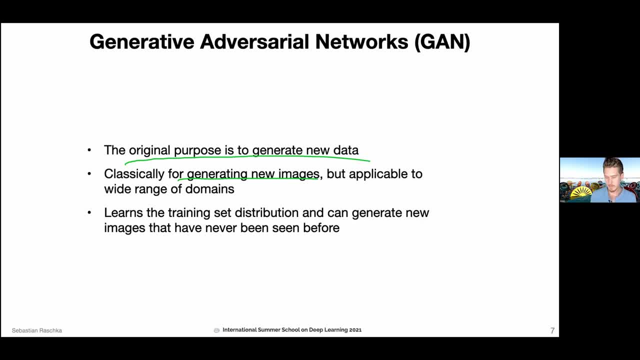 the researcher is working with, you can show it to someone, and this person would be likely able to tell whether this image looks realistic or not. so i think that's one of the reasons why working with images is especially attractive when we are developing new methods, because then it's really easy for everyone to see how good a method is. 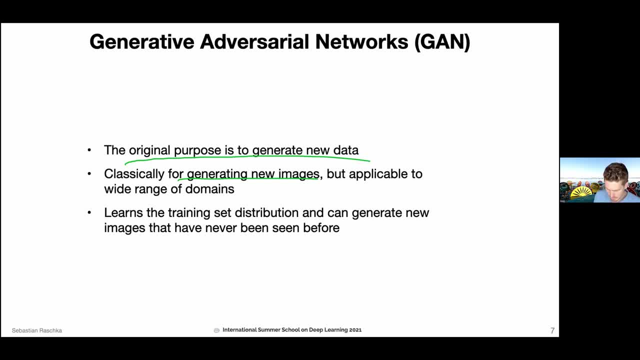 and how does that work? so it's um fundamentally, essentially about learning the dataset distribution, like implicitly learning this distribution of a training set, and then we can sample from this distribution or we can use the distribution to generate new images that have never been seen before, so generating new data. i've recently, for example, also seen applications where 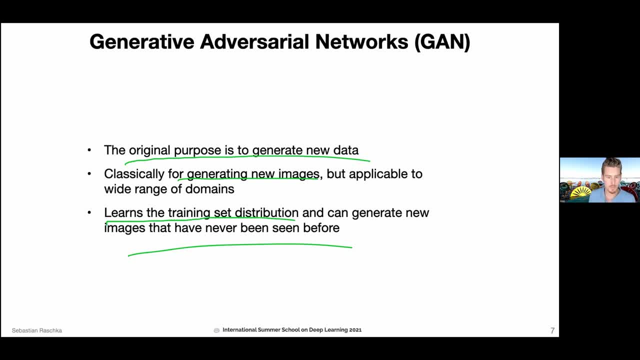 people also do this to augment training sets. so when you have a problem with limited data and you and you want to train a classifier and you only have so few examples, Some people I've seen they use GANs to generate synthetic data. 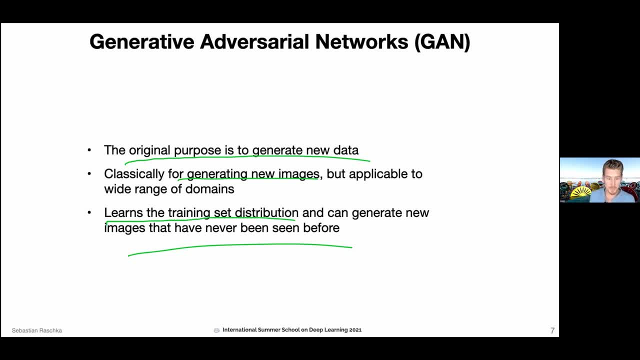 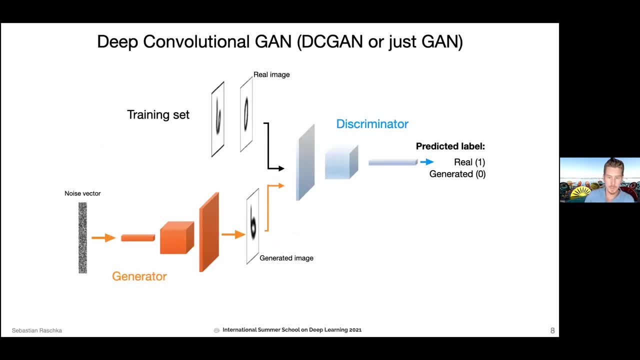 That is also one potential application. But yeah, let's focus more on the broad concept here. learning like this, training, set distribution to generate new data. So here I sketched an outline of a GAN. So- and this is a deep, convolutional GAN- DC GAN. 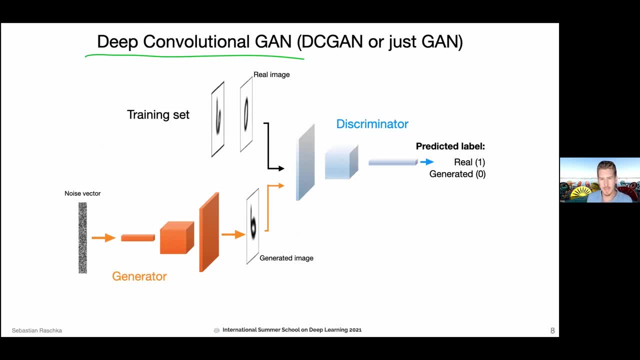 Nowadays, when people talk about GAN, most of the time- I would say 90% of the time- they mean a deep, convolutional GAN. So it's essentially a GAN with convolutional layers, because if you use or work with images, it's helpful. 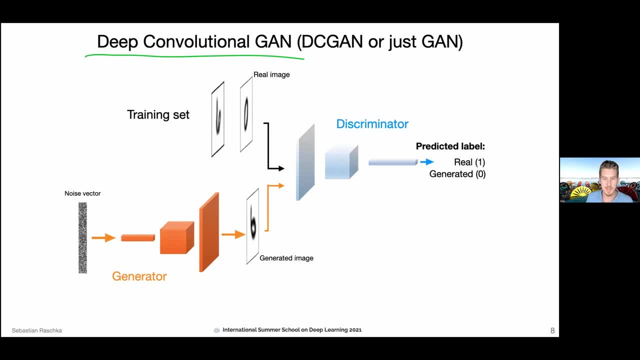 Yeah, as you've learned yesterday in Jacek's lecture, it's useful to work with convolutional layers. So, and this GAN consists of two neural networks. essentially it's a neural network consisting of two sub networks. So we have this discriminator network here. 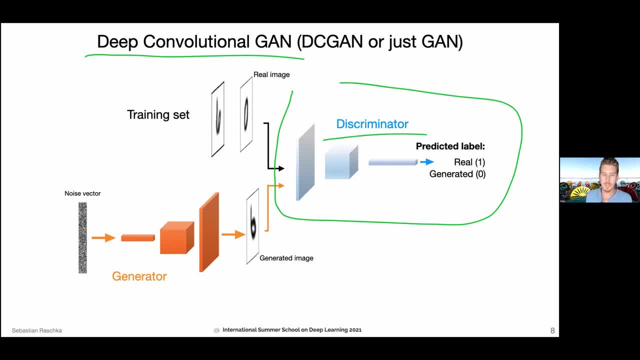 So this is a convolutional GAN and this is a convolutional network, And you can think of this as a convolutional network classifier, a binary classifier. And what is it classifying? So it's classifying whether an image is real or generated. 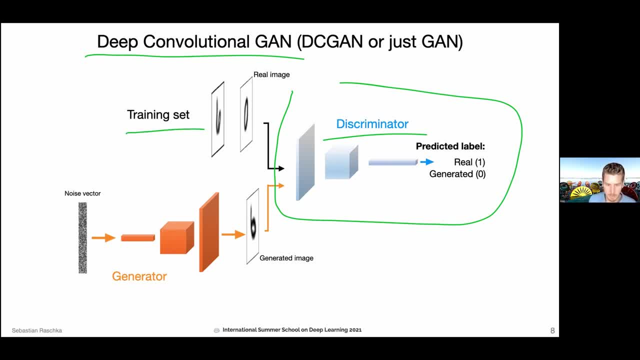 So if you consider here on the left-hand side, the training set, let's say these are my handwritten digits. So here I have a digit six and a zero, just as an example of two possible images, And these are images from a training set. 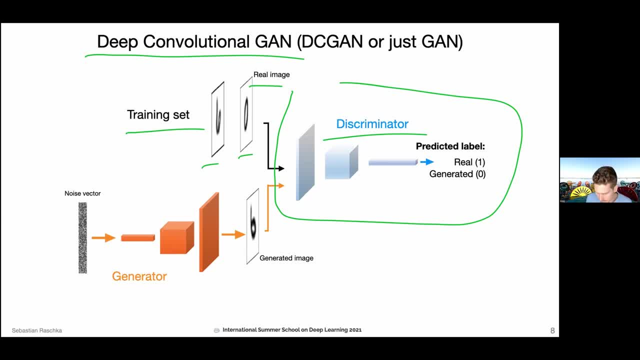 So these are real images And the discriminator, ideally, would predict that they are indeed real. So we have a class table for real images of one. So the class table is one and the discriminator we train it to predict that these are indeed real images. 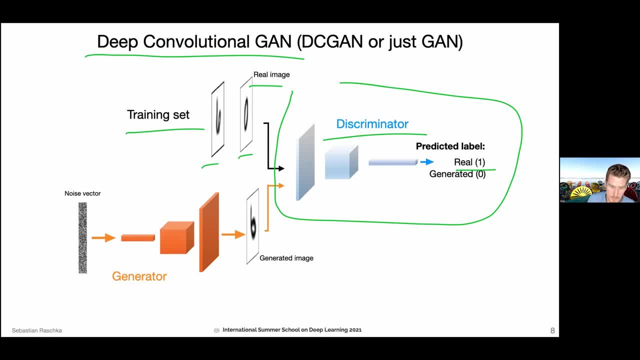 On the other hand then a different type of input. I mean, it's also an image, but the second type of input are these generated images. So the generated image is then created by this second neural network, the generator. So the generator takes in a noise vector. 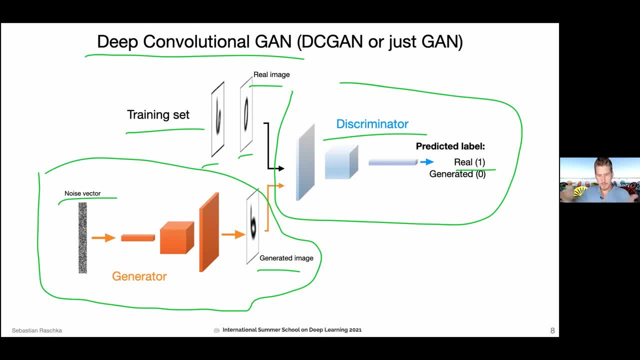 It's a random vector, For example, 100 elements in a vector, a sample from the random uniform or random normal distribution And this then goes through different convolution layers, So a series of convolution layers, And you can see here based on the shapes: 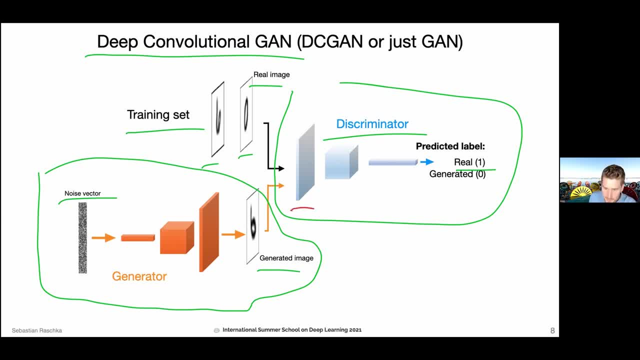 So here on the right-hand side, if we go back to the discriminator, I start with this relatively large feature map and then it becomes smaller and smaller, Or the number of changes channels. So here the width should represent the number of channels and the height and 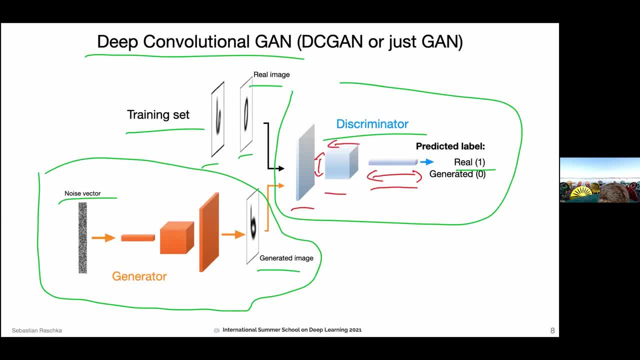 oops, sorry, I jumped too far. The height and width here. these are representing the height and width of the image. So the height and width of the image becomes smaller and smaller and smaller, And the number of channel becomes larger and larger, or longer and longer. 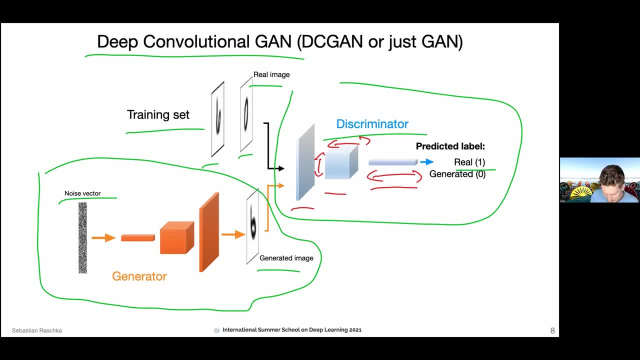 So this is usually the typical setup for convolution network And you can see for the generator. I kind of inverted this. So you start with a lot of channels, So you reshape this vector into, let's say, a one by one, by one hundred channels vector, And then you go backwards. 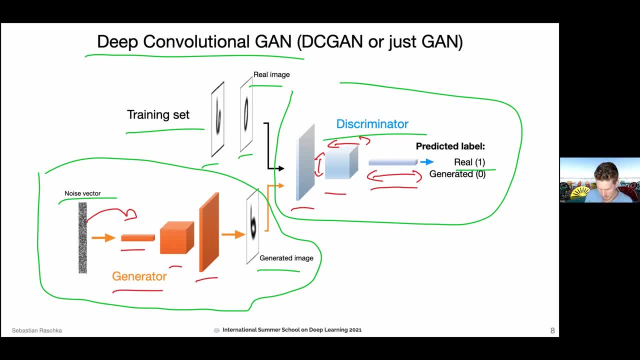 to generate the dimension of the original image. So you end up with a generated image, And then the task of the discriminator is to predict that this is indeed a generated image. So the discriminator is essentially a binary classifier predicting whether an image is real or generated. 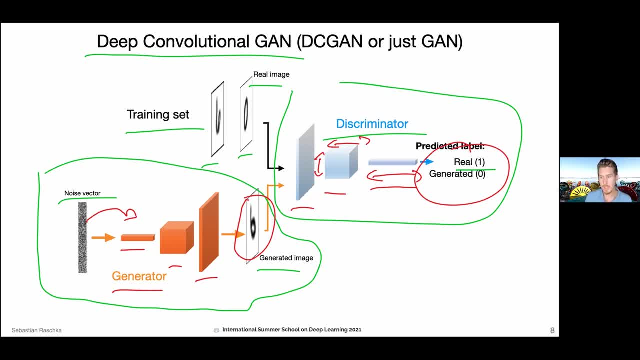 and the discriminator. the task is to become better at distinguishing between the two and the generator that got. the task is to become better at generating these images to fool the discriminator. so there are two kind of adversarial objectives: the generator wants to be better at fooling it and the discriminator- would be well wants to be better at telling those apart. so in 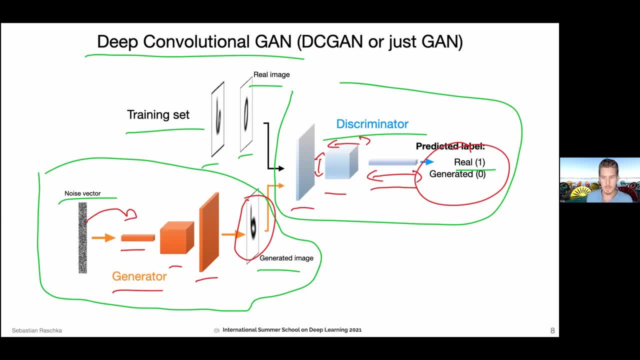 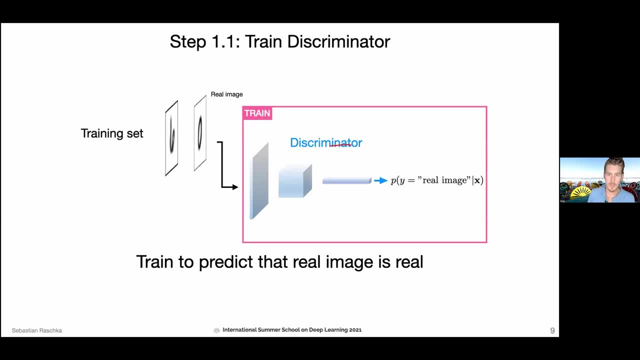 that way. that's why it's called um generative adversarial network. the adversarial comes from the fact that they are competing against each other. okay, so how do we train this network now? so i will, in the next slides, outline the main two steps for doing that. so first step 1.1 would be: 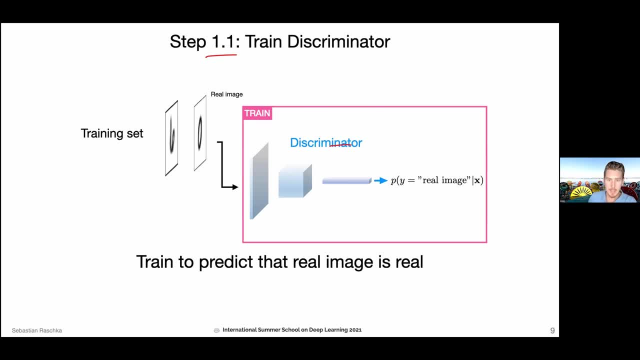 training the discriminator. so how do we do that? yeah, like i mentioned before, we then provide it with um data from the training set and i should say, um, we don't need labels in our data set like labels about what type of data that is. it's kind of like an unsupervised method. i mean the 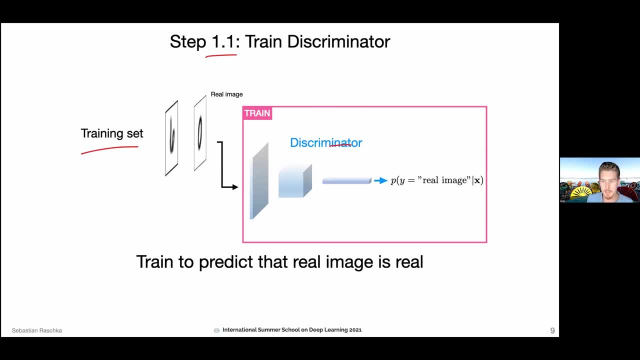 discriminator. you still use class labels, but we provide these classes. we don't have to have class labels or problem in our data set so we can generate these class limits by just saying: everything in our training set is classable 1. these are our real images and we can say all the 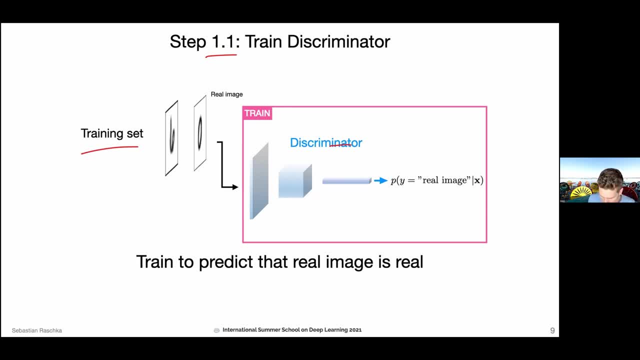 generated images have class label 0.. so and we train it um by maximizing, for instance, the probability that this is a indeed our generated image. so we want to predict class table one and in a binary classification problem, this is essentially the conditional probability that this is a real image given. 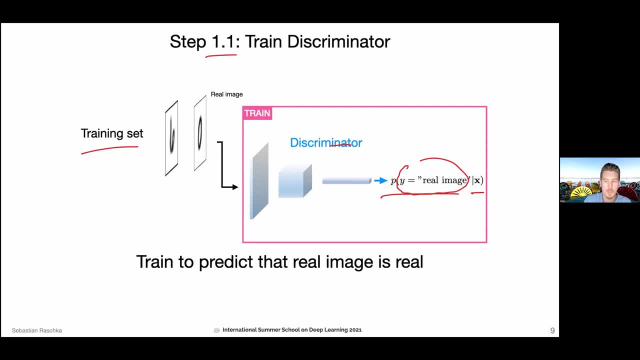 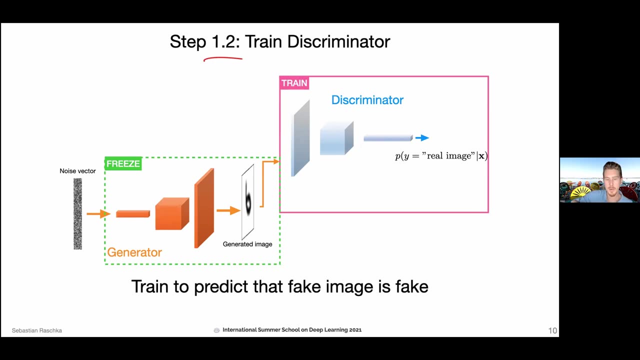 x. x here just means the um features the image itself. so we want to train this discriminator to predict that these real images are indeed real- then in the next step- so this is still step one, but i call it 1.2 because now we try to um train it on the generated 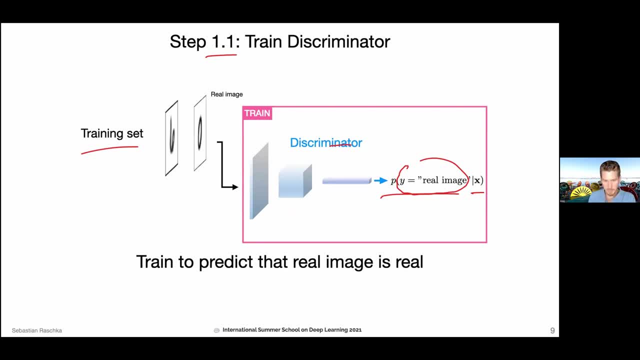 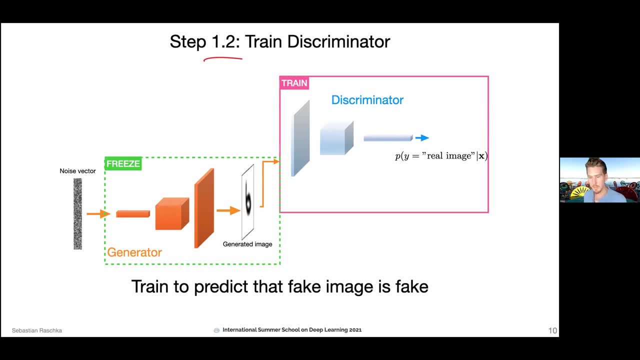 images. so there are two things. one, like i mentioned before, we want to predict that real images are indeed real, and now we want to predict that the fake images or generated images are indeed generated. so here i stay: fake, but with fake i mean um generated, so the same thing. 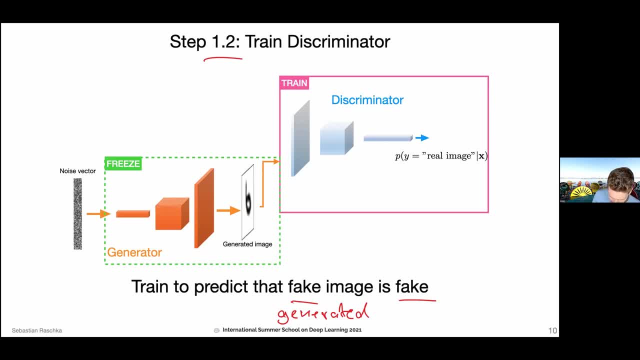 okay, so here um also note. i have two annotations here. one is a freeze and one is train. this is one of the tricky parts when we implement a gan in practice because, uh, when you use, for example, tensorflow or pytorch, there is this automatic differentiation and if things are connected and you call the backward pass or you run the um gradient, 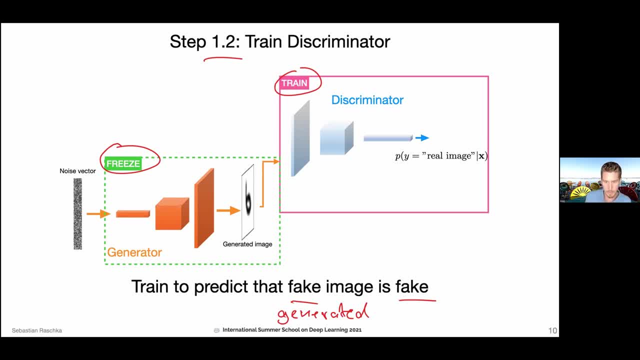 computation. it will compute the gradients for the whole network and then do the updates, and this is not what we want in this step. we don't want to train the generator, we really just want to train the discriminator. so we have to make sure that we keep the weights in the generator as fixed. 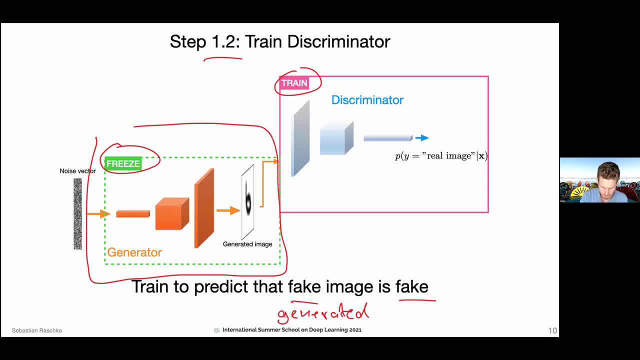 when we update the discriminator at this point and um code is- i will show you later how we do that. it's actually pretty straightforward, but it's like a little gotcha. so if you are having bugs or are not careful, it's easy to make this mistake- that all the weights are updated and 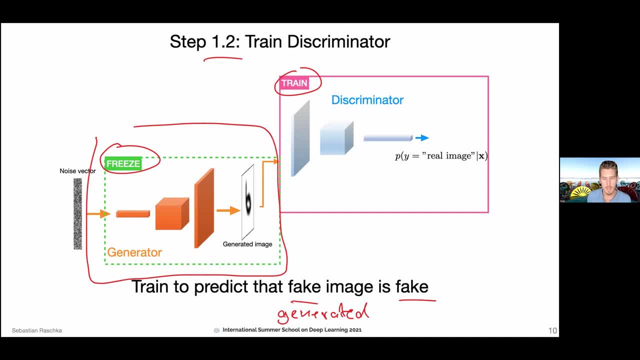 then you get weird results and it's sometimes hard to tell where it's coming from. so that's one thing to keep in mind. if things are a little bit funky, it's always good to double check that you are indeed keeping the weights of the generator fixed when you are updating the discriminator. 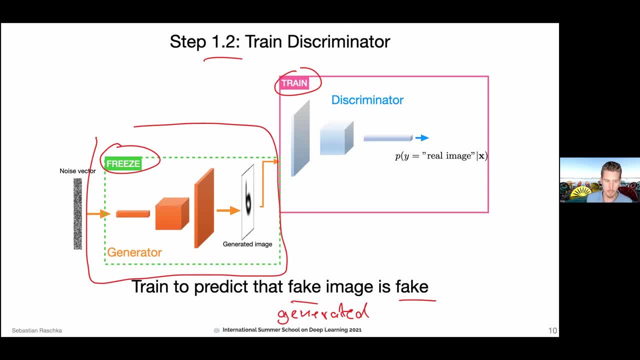 and again. this will become more clear later when we look at the code example. so here now, what we are doing is: um, we're keeping these weights for the generator fixed and only update the discriminator weights, and again, the goal here is that it outputs a zero class of the. 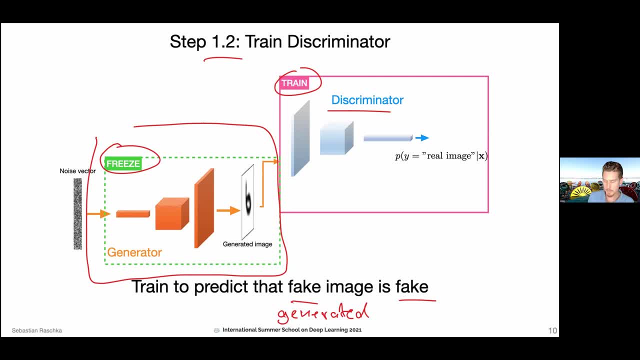 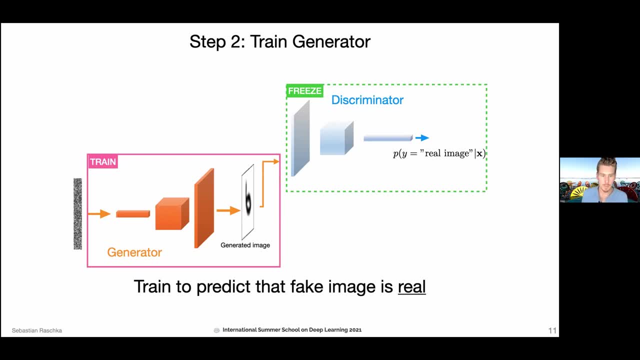 zero for these generated images. so these, um step 1.1 and step 1.2, were the discriminator training steps, and now step two would be training the generator. here we do um the opposite. we are now fixing the discriminator and are only training the generator here. so the generator. 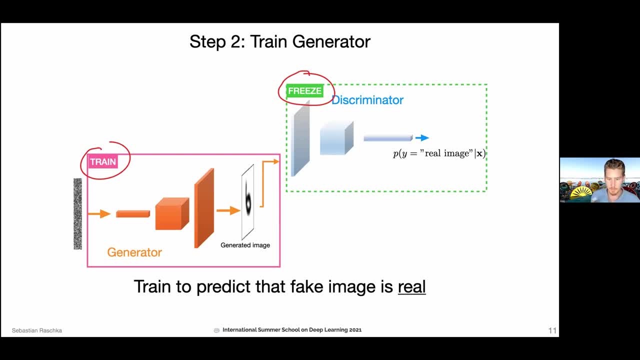 now the goal is to learn to fool the discriminator. so what we want is now that the discriminator thinks that these generated or fake images are real images. well, why do we want to do that? um, yeah, so we, we want to generate. also, we want to generate realistic images. 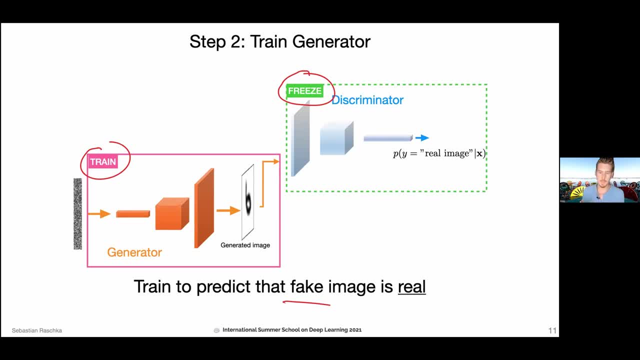 and you can think of the discriminator as a critic. you can think of it as maybe a human like me or you, and we are looking at this image and we are saying that it doesn't look quite right And if we say, okay, this is not right, then the generator will get. 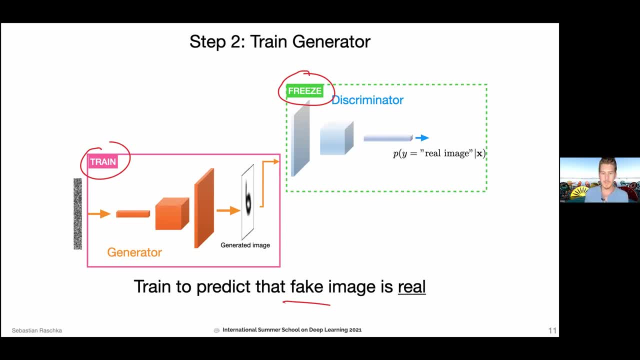 a penalty and it will next time try harder to generate a better image, essentially. So we want to make the discriminator better, to also push the generator to become better. So, yeah, this is, like the, the main, the main outline of how a GAN works. So it's essentially 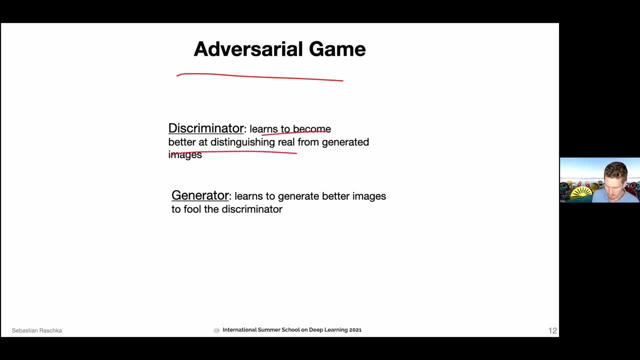 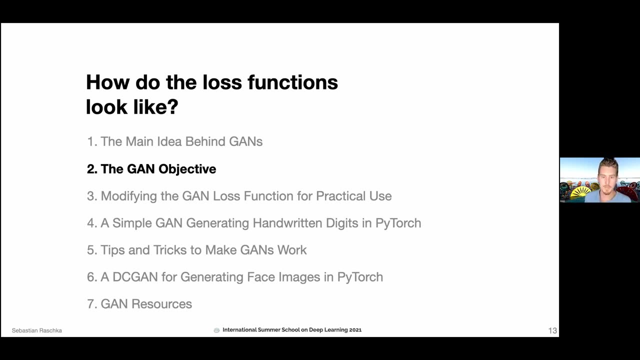 this adversarial game that the discriminator learns to become better at distinguishing real from generated images and the generator learns to generate better images to fool this discriminator. Okay, So this was the main idea behind GANs. So these two sub networks playing this adversarial game with each other. And then the next slides. I will go over some. 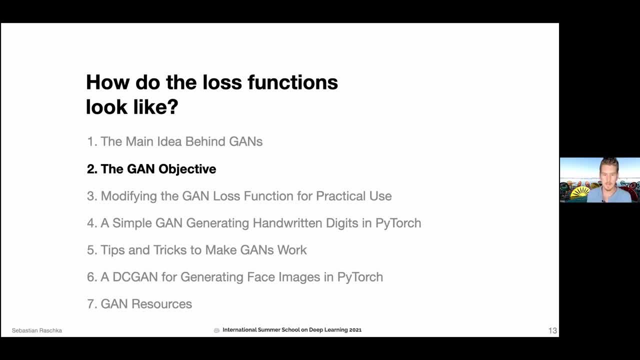 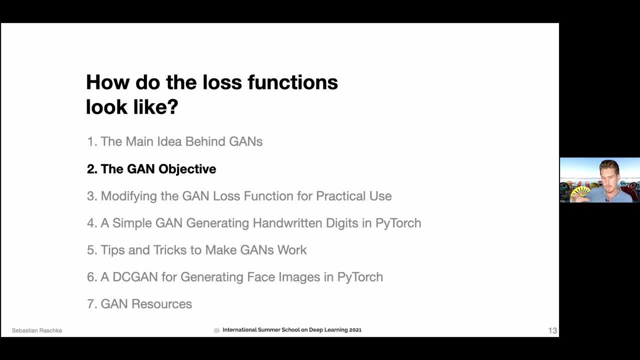 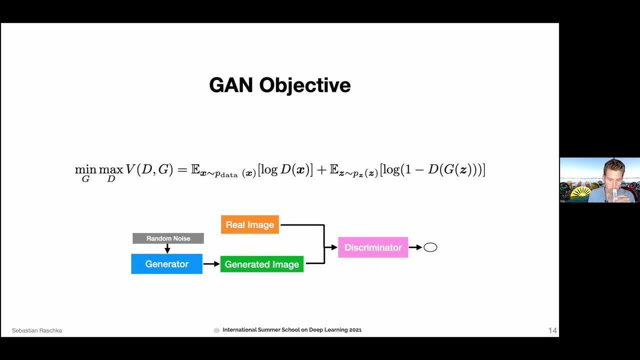 the brief overview that we kind of need in order to express this training objective in code later on. So I have taken, so I've taken this equation from the original paper. So this is the objective, again objective, and here at the bottom this is just a summary of what I've just shown. 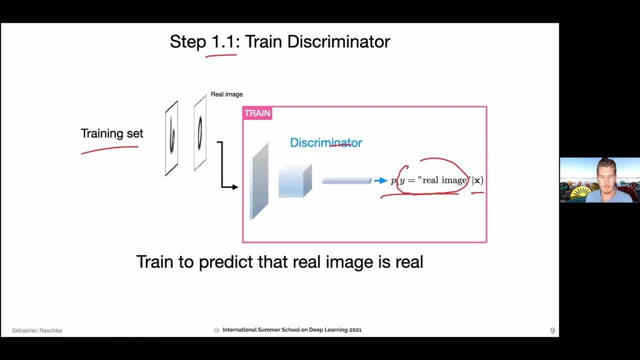 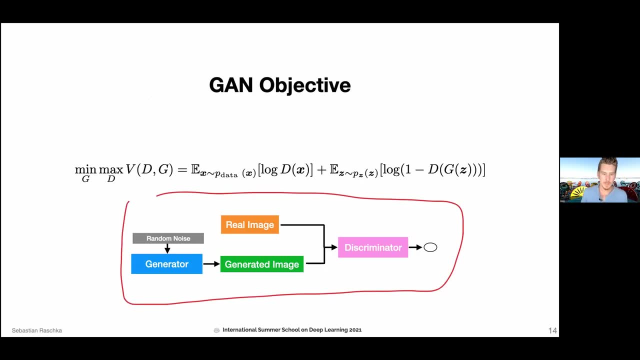 you by go back to the slide I added. I showed you it like this and I just summarized it for reference here at the bottom again for you. So it's again the same setup. The generator here receives a noise vector. It becomes the generated images through the generator. 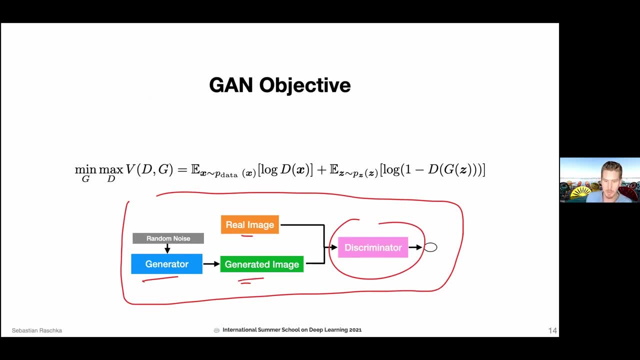 and the discriminator has to tell apart real versus generated images. And for that, in order to train the setup, yeah, we need an objective, something that we can optimize in PyTorch or TensorFlow, And here this is taken from the original paper. 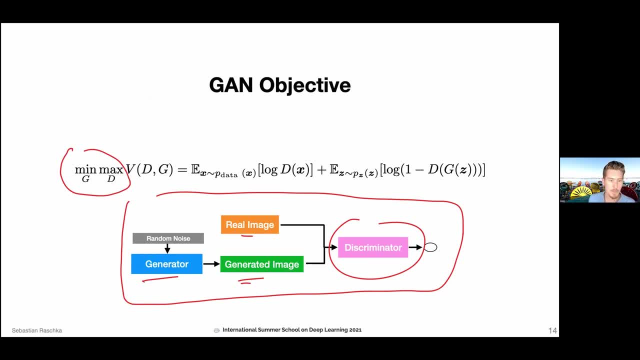 It's expressed as a min-max game, So we want to minimize something while we want to maximize something else. So it's like this kind of trade-off that we have here. So I will, in the next couple of slides, also look at a simplified version of that. 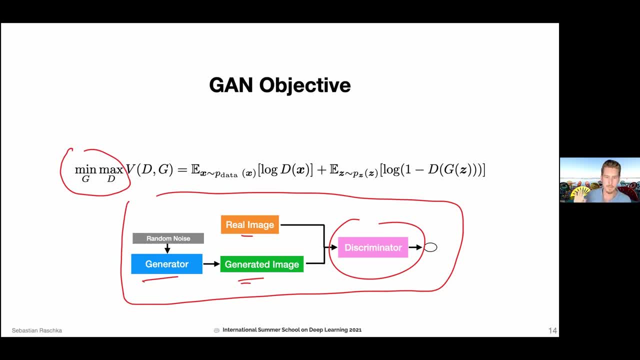 but because I think this is like one of the most fundamental things about GANs- you will probably encounter this in textbooks and GAN papers- I thought it might be useful to show it to you, But yeah, I can imagine it looks quite daunting. 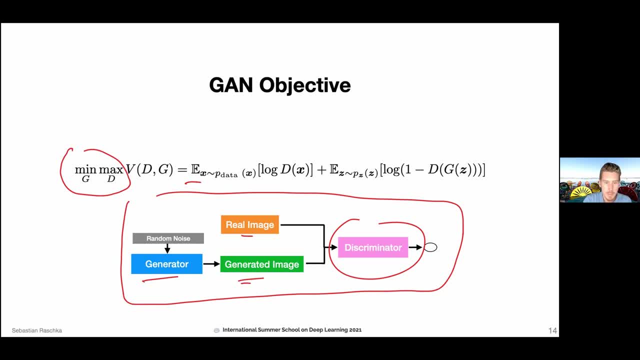 So if you don't know what this E here is, this stands for the empirical risk, essentially. So it's like one thing in deep learning papers to write something in a more general sense versus the practical one. So here we are, assuming we are talking. 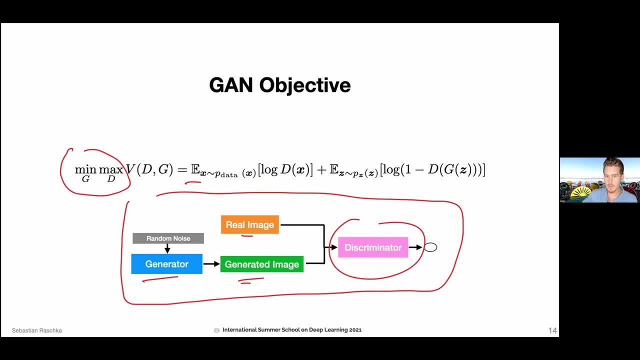 about the whole distribution of the data that the training set comes from. So here the X would be like the data distribution, So random variable distributed according to whatever distribution generated our training set. But of course in practice we never really have the whole distribution of the training. 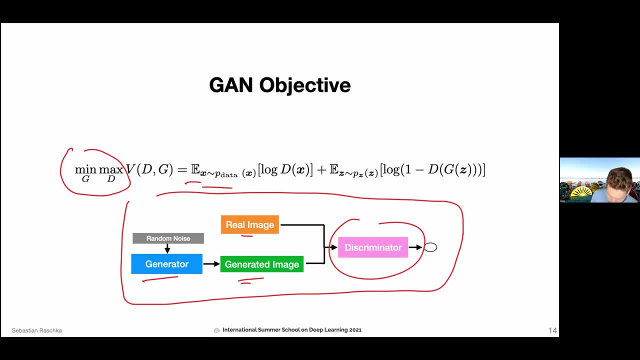 data right. So in practice we only have a training set. So this E in practice would more like become a sum over something. So in practice we would have, let's say, 1 over n, sum over, let's say: i equals 1 over n. 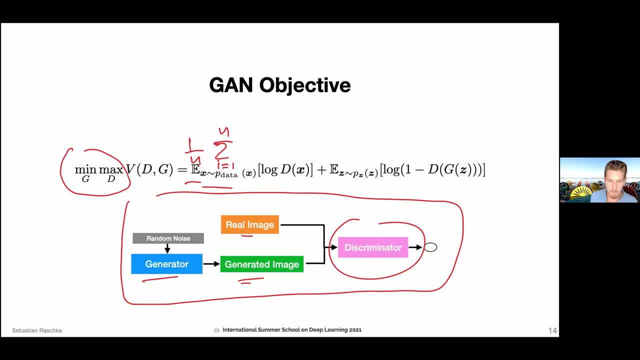 So it's more like a discrete version. We would be summing, We would be summing over something, instead of having a continuous version of that. But yeah, this E symbol here. you can really think of it as encapsulating all the data. 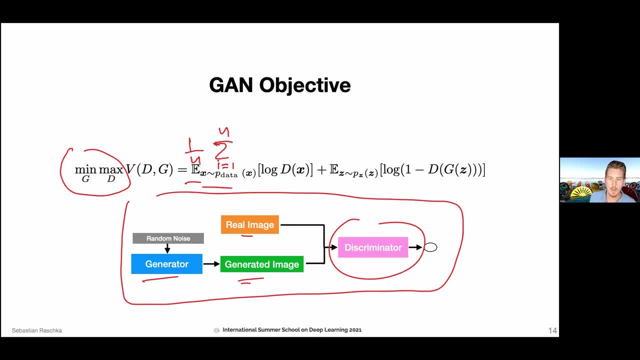 that could be sampled from the distribution? Yeah, and there are two. So, focusing on this objective, there are two things going on here. We can think of the plus sign here as our center point, So this would be something on the left side. 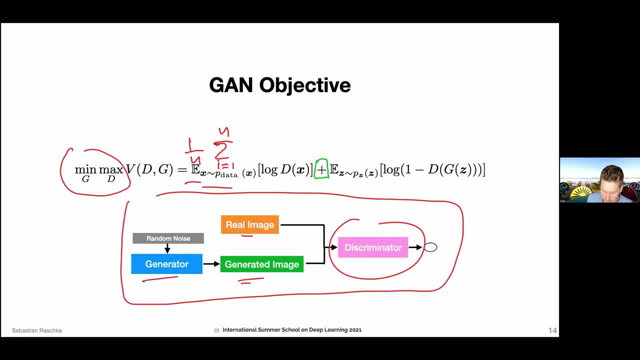 and on the right side of this plus symbol. So we are combining two things. And on the left-hand side, if we look at this here, we can see that there is only the discriminator involved. So we have this dx here And the dx- the d, stands for the discriminator. 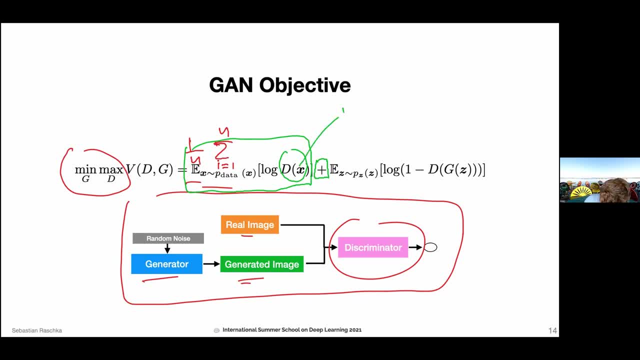 And x is just the data, the image data. So let's say: this is our image here. d is our discriminator. Oops, yeah, somehow it's always skipping forward, Sorry, This is our discriminator. And So what we want to do is we want to maximize this. 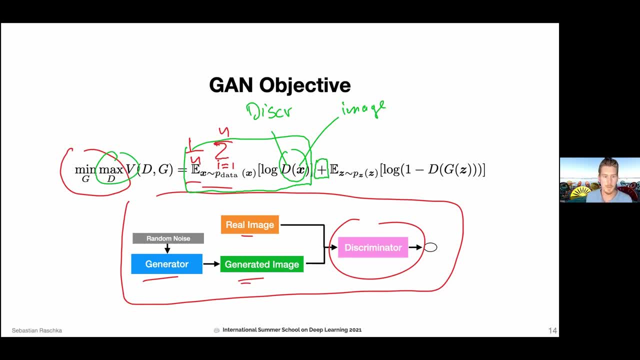 So this is the maximization part. We want to maximize things with respect to the discriminator weights, We want to maximize the term with respect to the discriminator- And I will go through this more slowly later. But if we have the discriminator, if it's a classifier and we use, let's say, 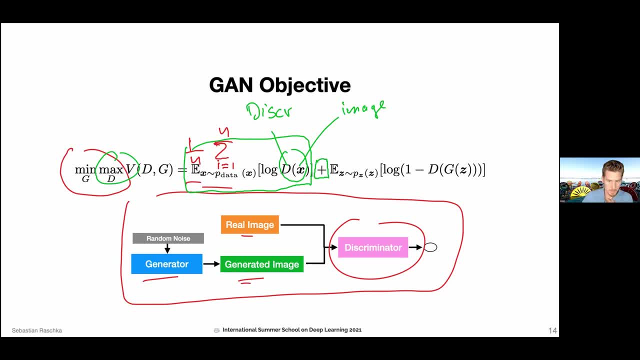 sigma activation as the last output layer or as the last layer in the network. we have squares in the range between, say, 0 and 1, so where that stands for the probability that this is a real image, And yeah, so if we look at this, so the log of 0. 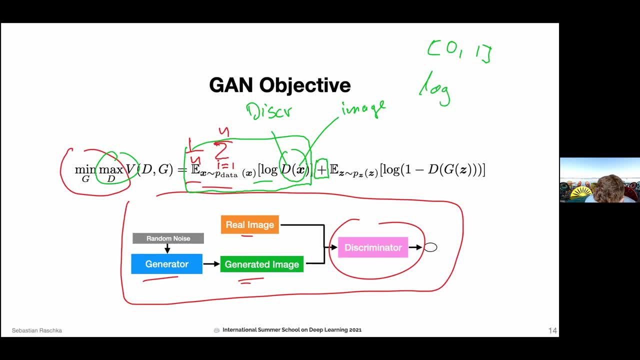 would be if we take the log here, the log of 0 would be minus infinity, So this would be very bad And the log of 1 would be 0. So in this case we would maximize this whole left hand side. if the discriminator indeed 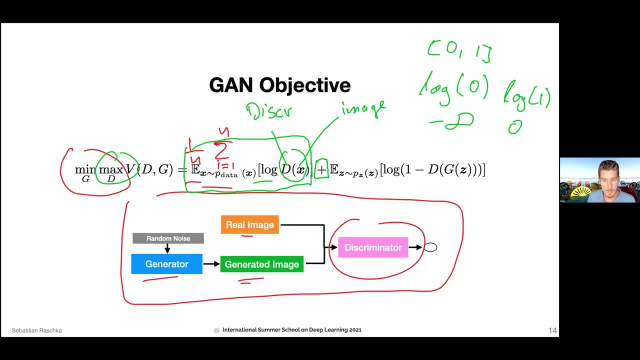 outputs a 1, the score of 1.. That would be the ideal case, because otherwise it would be infinitely low minus infinity here. So we want to maximize this part. So it's just to a little bit understand what's going on here. 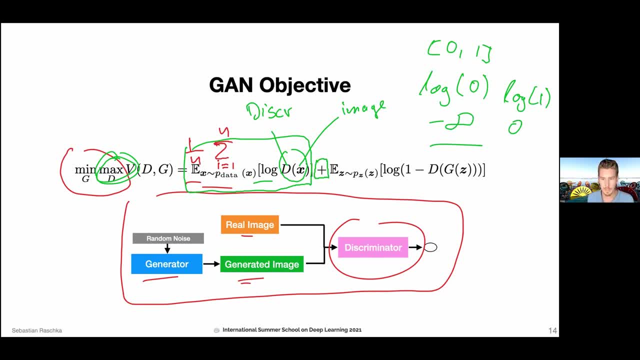 And then we can use that in code to train our GAN. So this is only the left hand part. On the right hand part, we also have a D here, So there's another D And we also want to maximize this right hand side. 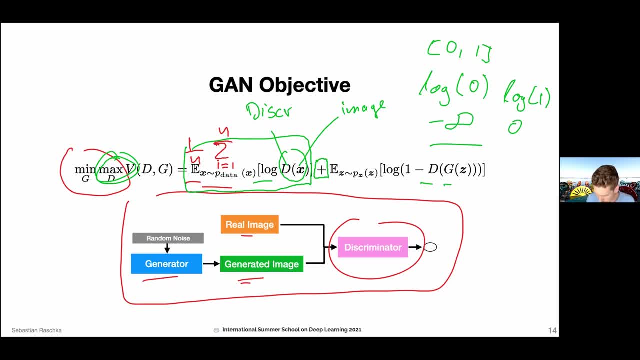 So this right hand side here involves a G and a Z. So the Z here would be the noise vector And the G here is our generator. And now we still- I mean the D- D is our discriminator. still It still outputs something between 0 and 1,. 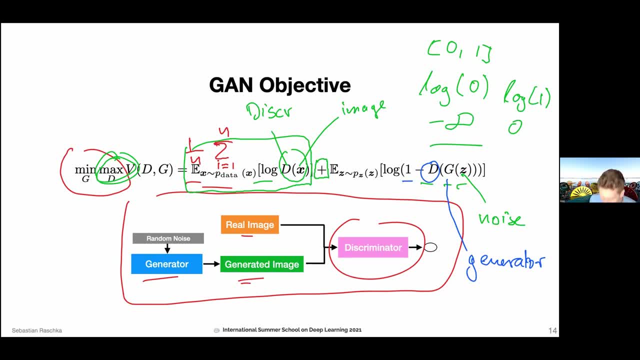 the probability score. But now we have this 1 minus here in front, So it's kind of flipping Right. So if we have 1 minus 1, it becomes 0. And if we have 1 minus 0, it's becoming 1.. 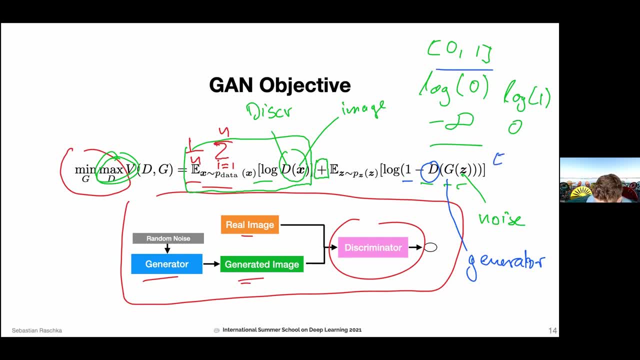 So it's kind of like the output instead of 0, 1 would be now 1, 0. And then if we have the log, the log of 1 is 0. And the log 0, running out of space would be minus infinity. 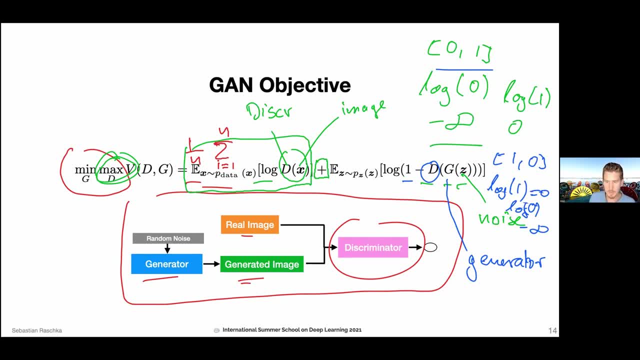 So in this way it's kind of reversed. So because we want to detect that this is a fake image. So here the score is maximized if we output 0, essentially So because we have the 1,- sorry, we have the minus in front. 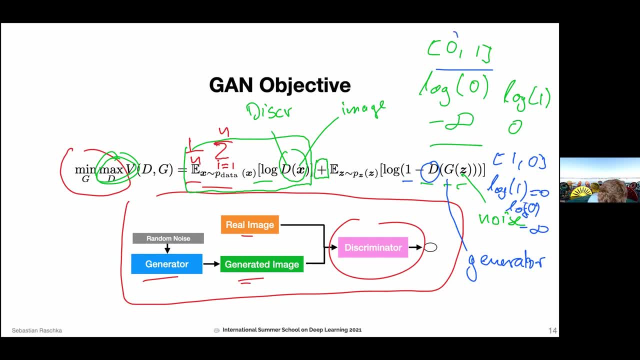 So if we output 0, it becomes this 1. And then this becomes the maximum score. So it's kind of like the opposite of the left hand side, where we also want to maximize, And this is maximized if the discriminator predicts. 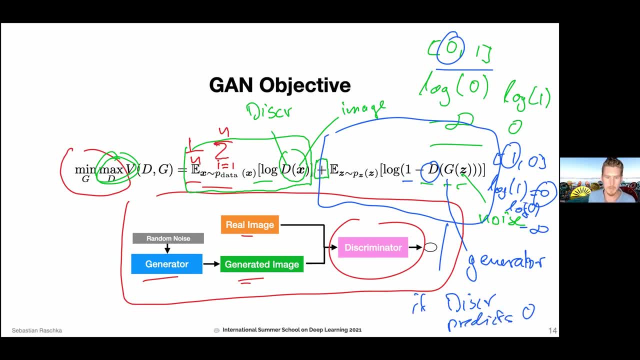 0. So it's kind of the other way around, And so we were only focusing here on the discriminator part. But then we have also this objective: minimizing this for the generator. So we could do the same thing now for the generator, And if we look at the left side, here there is no g involved. 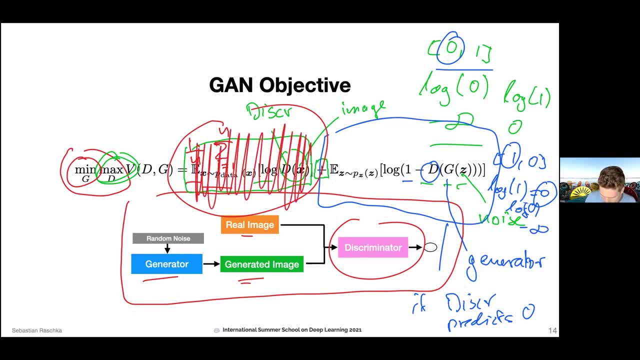 So we can actually ignore this whole left hand side, only focusing on the right hand side. And when is this minimized? This is essentially minimized when- OK, when the discriminator predicts a 1, because the 1,, we have the 1 minus 1.. 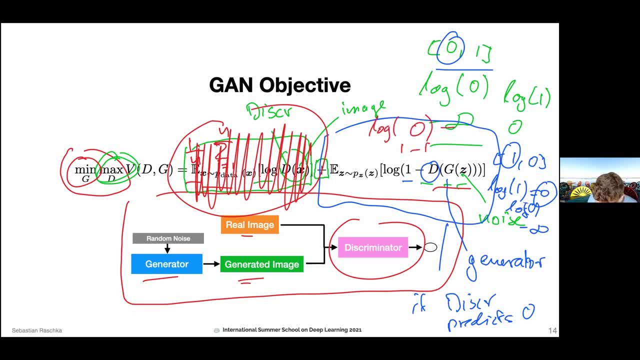 This becomes 0. And then log of 0 becomes minus infinity, And this would be then minimized when the discriminator outputs a 1 for this score, because that's like fooling the discriminator, forcing it to predict the wrong label. So this is essentially how the scan objective works. 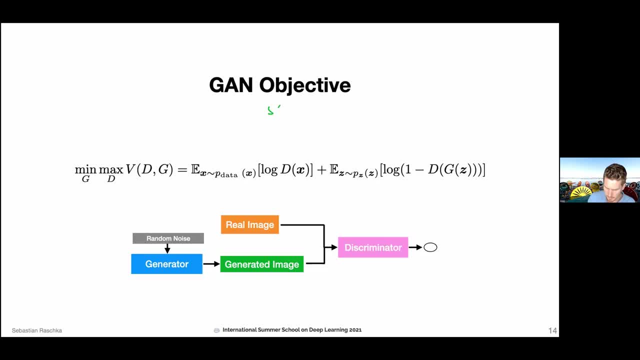 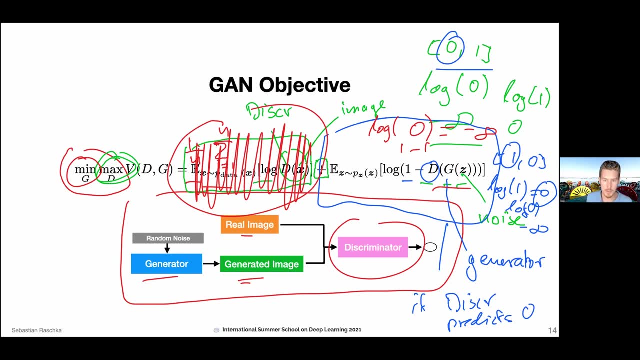 And this is how the scan objective works, And this is essentially how the scan objective works. And this is essentially how the scan objective works In practice. if you have worked with TensorFlow or PyTorch before, there is something we have available called stochastic gradient descent. 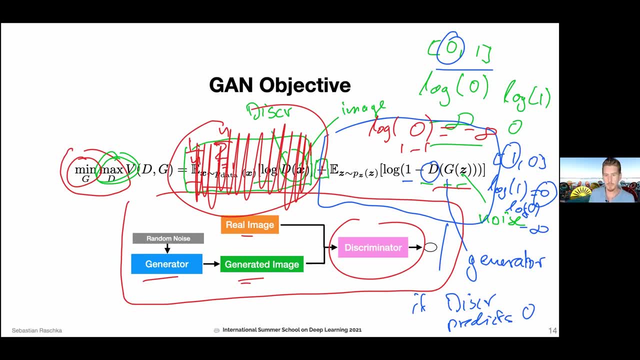 It's for minimizing loss functions. We could just flip it around and maximize something We'll call that then gradiates ascent. so gradient ascent instead of descent. But why not just simplifying it so that we can use stochastic gradient descent all the way? 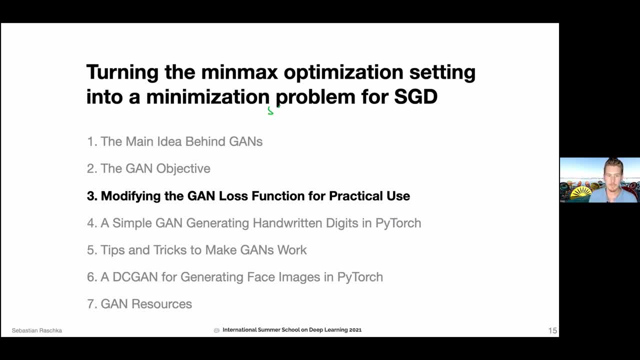 fast rubber faudra 6. So here I have what I just talked about, just so that we can use the stochastic gradient descent all the way. If we apply stochastic gradient descent here, the model won't stop. ask to sample. if the mass is least, then we are próprily no go. 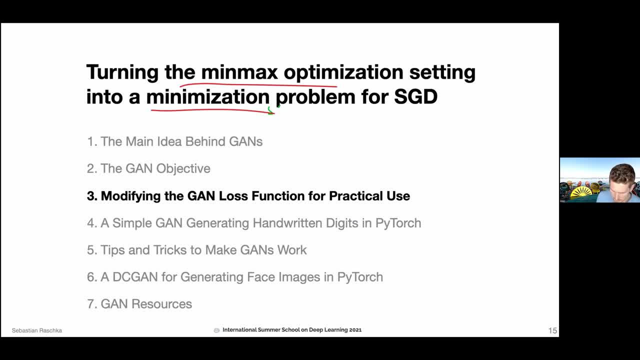 simplified it as a minimization problem. So instead of doing this min-max optimization, we are turning this into just a minimization problem. We can just do that by changing the sign, And I will show you in a few slides how that looks like, And I can imagine if you first. 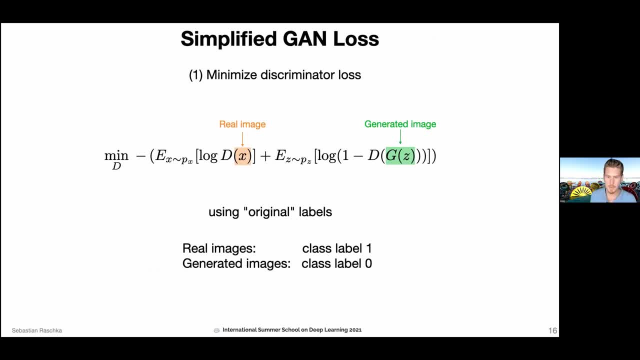 see this. it's kind of like pretty complicated. It's pretty quick, maybe also because we only have so much time here, But I will share the slides with you so you can also walk through this step by step later. So if things are not clear- And I'm also, of course, happy to answer- 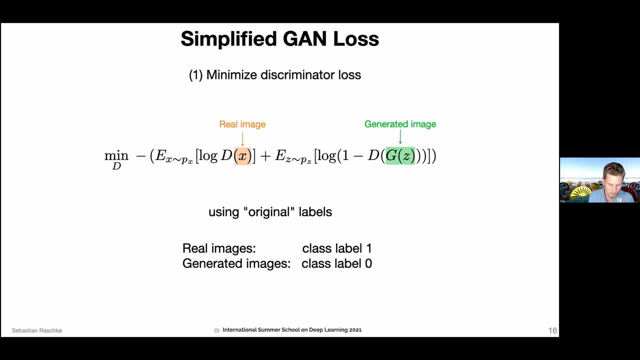 questions about that. So in the next couple of slides, before we go to the code examples, I will do a quick run through these equations again. So we have the task of minimizing this granite atmosphere. I talk about this in terms of what I've done before for the real images. 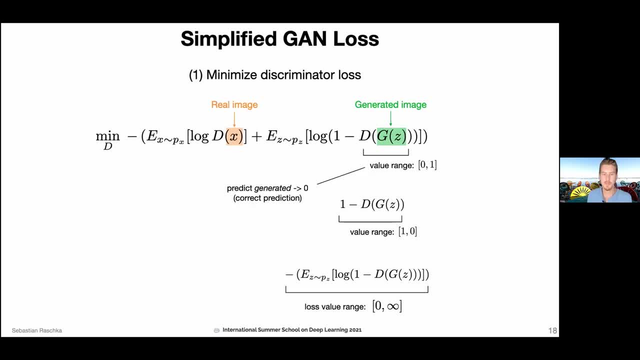 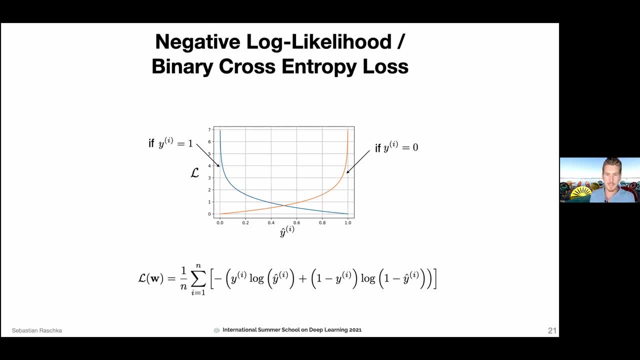 then for the generated images. So I will go back, I'll just show you what's going on, what's lying ahead, And then we will look at the generator loss And I will then explain how we implement that using tools we already have. 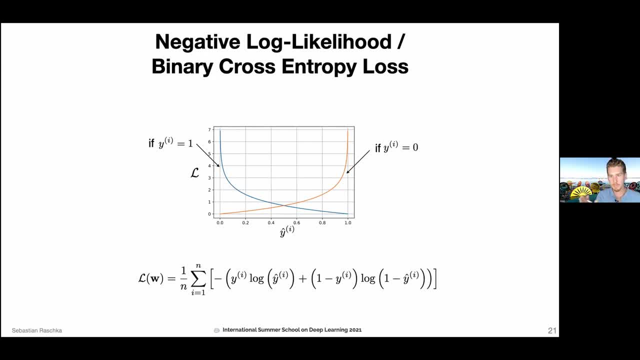 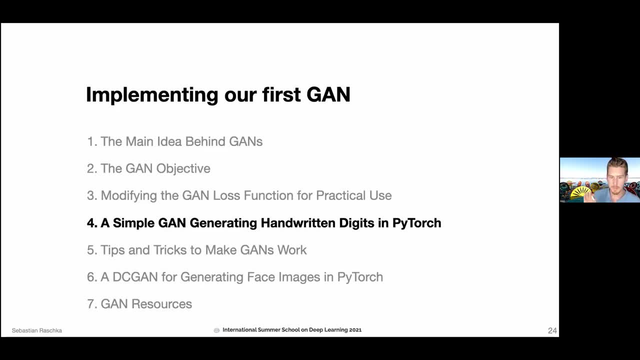 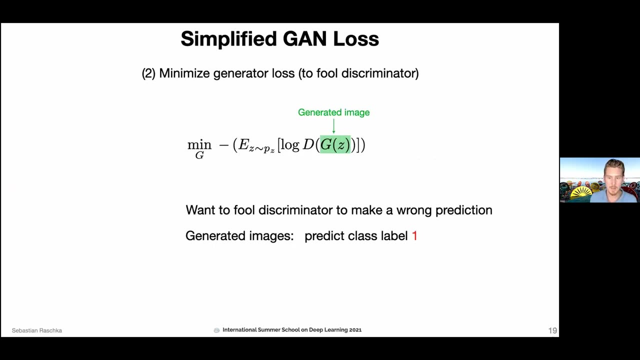 available in TensorFlow and PyTorch, namely the negative log likelihood, or also called binary cross entropy loss, And then after that, we will implement or look at the code implementation based on these concepts for generating digits. So, going back, walking through this now a little bit more slowly. So we are now first focusing on minimizing the 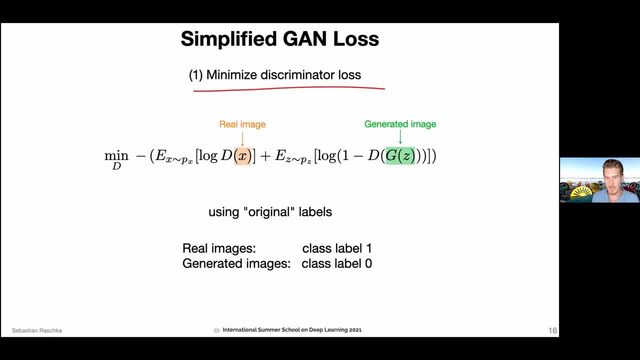 discriminator loss, And instead of using the GAN objective that I showed you before with this min max, we are only now looking at the discriminator, which we turned into a minimization problem here just by adding this minus sign here in front. But yeah, the concept remains the same, So we 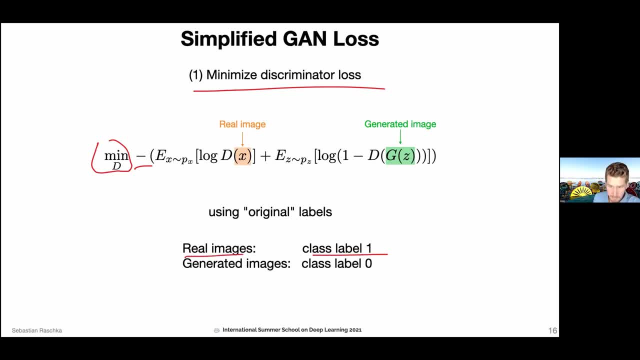 are assuming that for the real images we have the class label 1.. And for the generated images we have the class label 0. So we want this discriminator to output a 1 here And we want this discriminator to output a 0 here. ideally, That means that it correctly predicts real images as real. 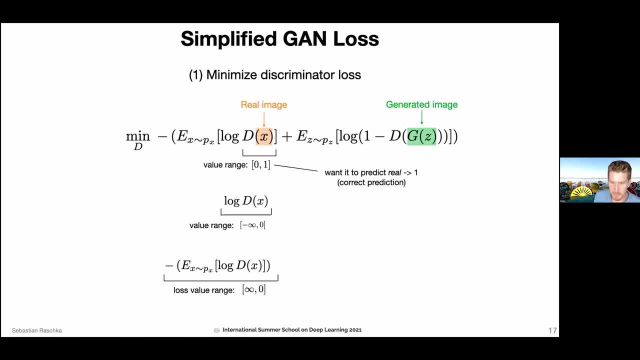 and generated images as generated. OK, so, like I mentioned before, the value range that we can get from the discriminator is some value between 0 and 1.. This is usually because we use a logistic sigmoid function like in a regular classifier. 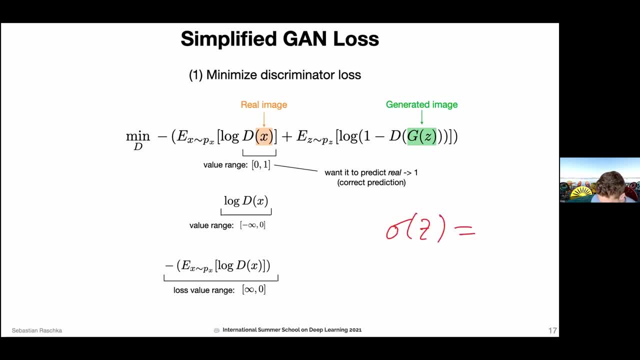 So the logistic sigmoid function would be something. if I don't make a mistake, it should look like this, where here Z would be the logits when you compute the inputs to a layer like the weighted sum. So if we have some weights- i and some inputs, usually the inputs. 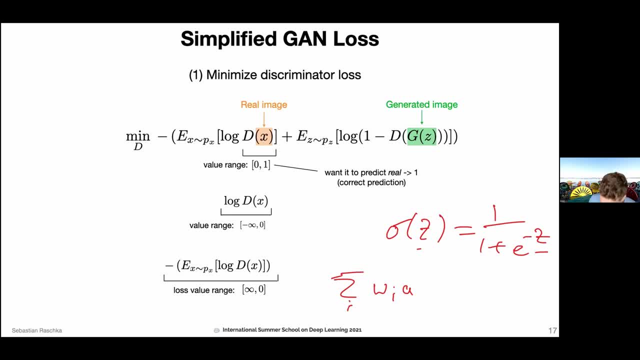 we can denote them as a, because they are the activations from the previous layer plus some bias unit. If we call that a Z, then if we put the Z through this logistic sigmoid, the output range would be between 0 and 1, where 1 here would correspond to a high probability that this is a real image. 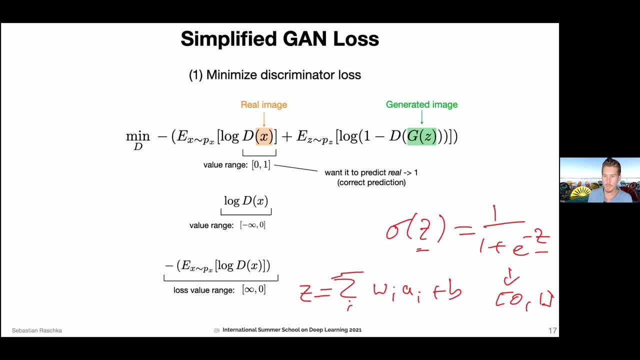 and a 0 would correspond to a low probability that this is a real image. I don't have a slide on this, unfortunately, but if I would just briefly sketch how the sigmoid looks like, So if we would plot this logistic sigmoid values here. 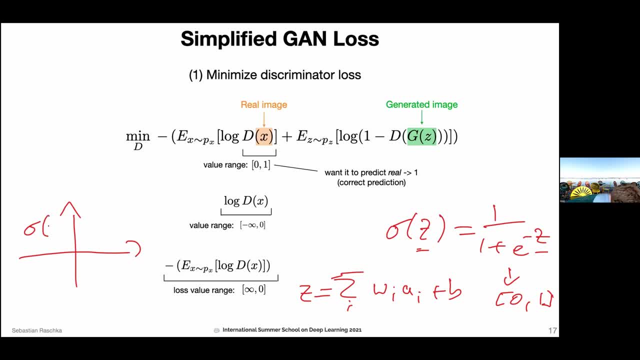 Oops, This would be like an S-shape, like an S-shaped curve, and between the value 1 and 0. And it's not a great drawing here, but there should be the center point here where it cuts the line at 0.5.. 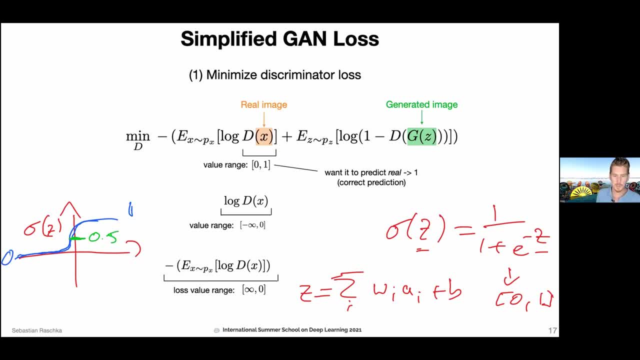 So usually we say we usually in practice use threshold function and say if this value is above 0.5, output class is 0.5.. Class table 1.. If it's below 0.5, output class table 0.. 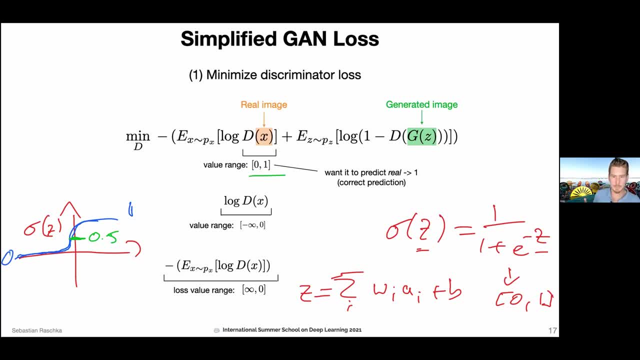 That's how we convert these values into class tables. But here for the gradient computation we don't do that. It's more like for the final step, when we compute, let's say in a classification example, or when we want to return the class tables. 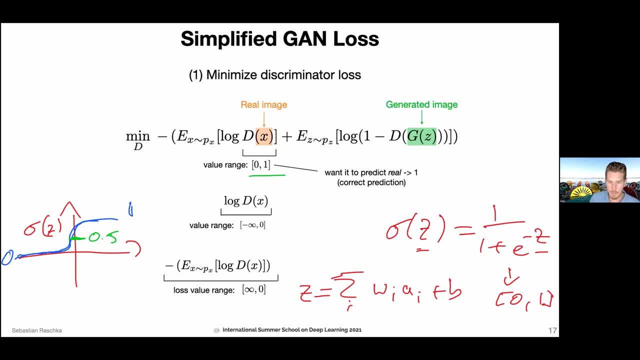 Here we are just working with these scores directly, But the same concept applies. We want the score to be close to 1 as possible. So if we want to return the class tables, we want to return the score. So, if we want to return the class tables, we want to return the score. 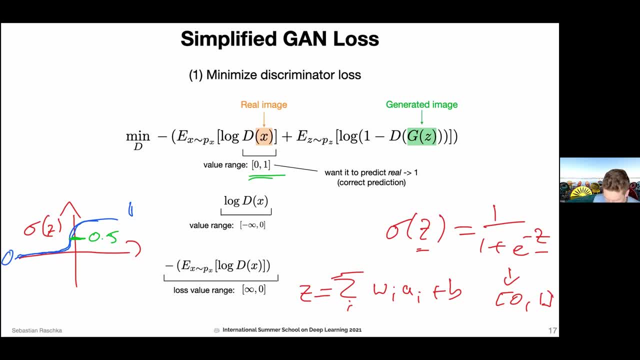 So if we want to return the score, we want to return the score. So if we have now for the real images the possible output range between 0 and 1, we add the log in front. This turns into then a minus infinity to 0 range, because the log of 0 is minus infinity. 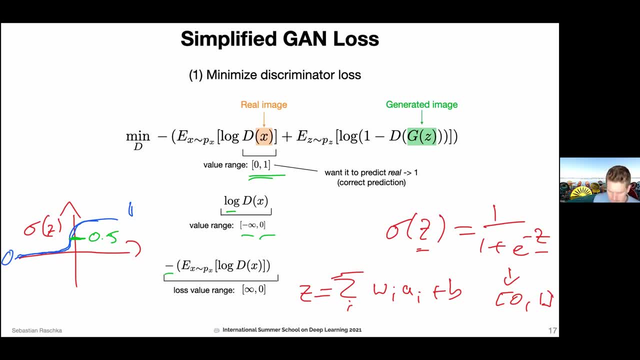 and the log of 1 is 0. And then now, when we add this minus in front, this will then turn into infinity to 0. And we want to minimize here, right? So this is a minimization problem. We want to minimize this. 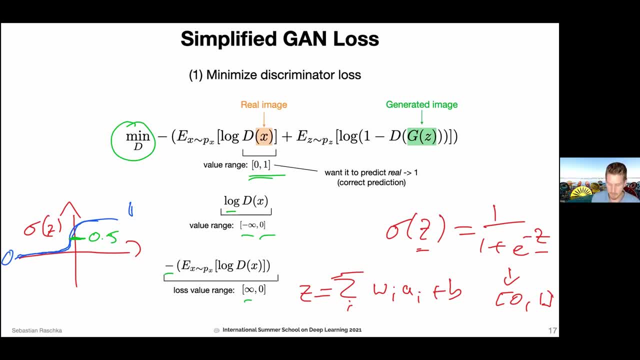 You can think of this as a loss function that we want to minimize And if we trace this back, so 0, 0, 1.. So ideally, the highest value we can get here is a 0, right? So the highest value we can get for this expression is a 0. 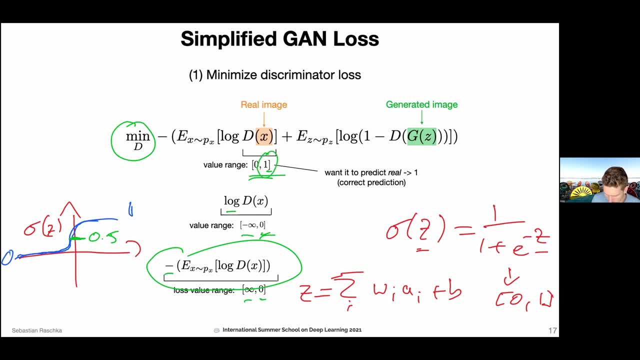 And this is achieved if we have the output label 1 here, or an output close to 1.. So yeah, so we want the discriminator to predict a 1 here. The same can do the same thing for the generated images. So for the generated images, we get the value range between 0 and 1.. 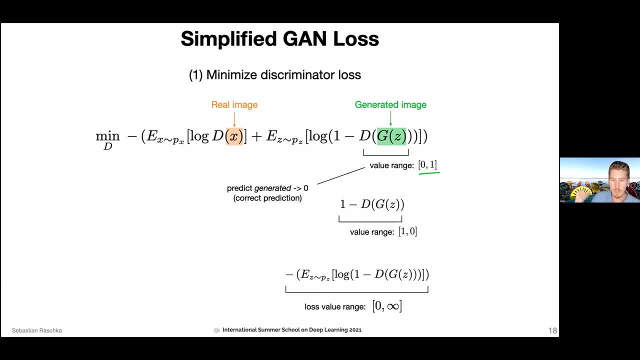 So we can do the same thing for the generated images. So for the generated images, we get the value range between 0 and 1.. And now we want to predict the class label 0, because they're not real images. they're. 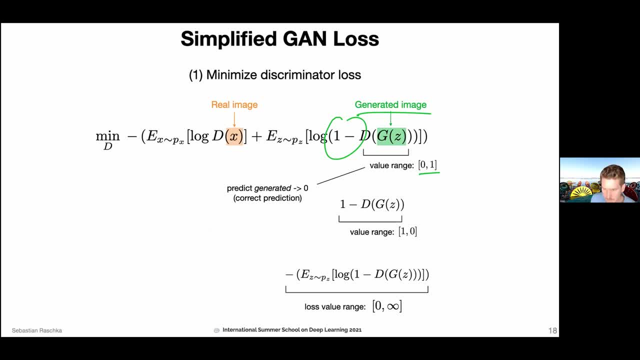 now the generated images. So that's why we have the 1 minus here in front. So the 1 minus turns the 0, 1 range into a 1, 0 range. And then, when we add this minus here in front and the lock, this turns into a 0 infinity. 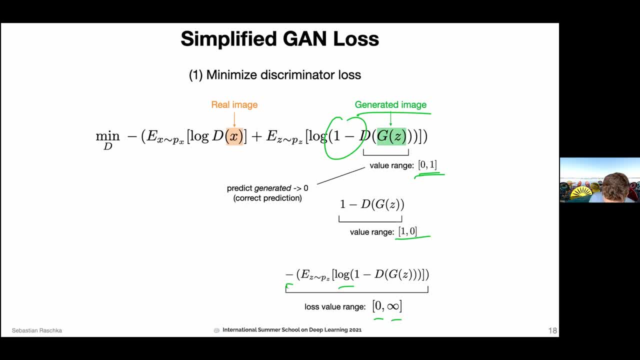 So here, in this case, this whole expression here, or the expression on the right-hand side of the plus symbol, And, of course, considering the 0 here, The minus sign, Then this has a value range between 0 and infinity and it's minimized when we have. 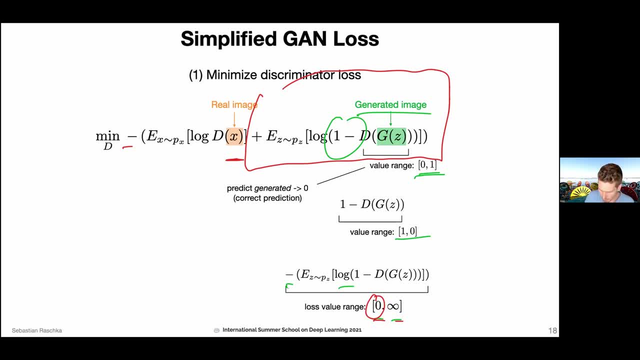 again this 0. And it's 0 when we have the output 0. If we have an output of 1, which would be very bad, very wrong- then we have an infinitely large loss, which is very bad. So this is like the setup for minimizing the discriminator. 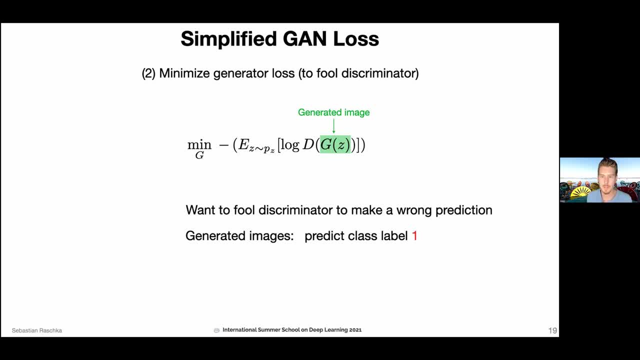 Now for the generator. we want it to fool the discriminator, So we want it to become better And so that it becomes so good that the discriminator can't tell apart what's real and what's fake. Then we have kind of achieved our goal. 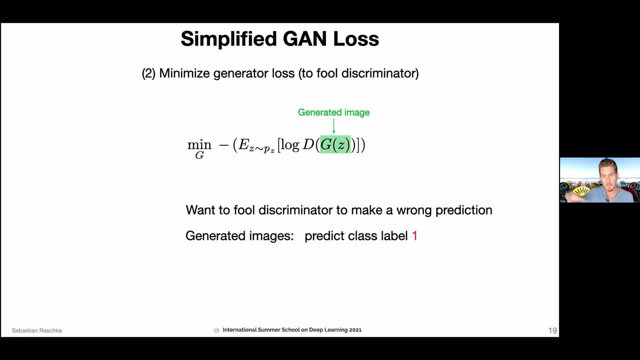 But of course, keeping in mind that the discriminator also becomes better all the time. So it's kind of like this adversarial game, But here we are training the generator to become better at fooling the discriminator. So we want, in order to fool it, or when it's fooled, we want the discriminator to predict. 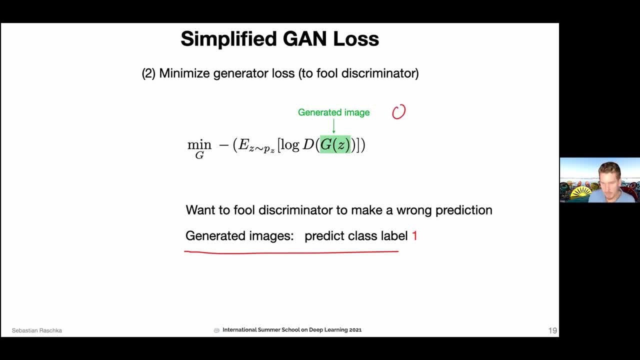 a 1 now. So it's generated. The true label is 0, but we want it to predict a 1 because we want to fool it, All right. So how do we do that? I mean we use a similar setup here. 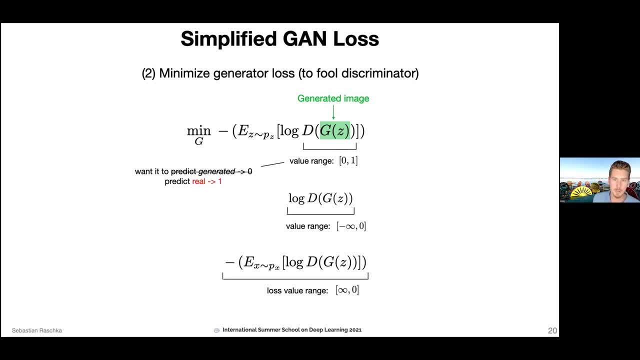 It's again a minimization problem, because it's easier to implement in PyTorch, because we can then use just stochastic gradient descent or let's say the atom optimizer, And yeah. so what we do is again, we look at this. So the d here is again still the discriminator. 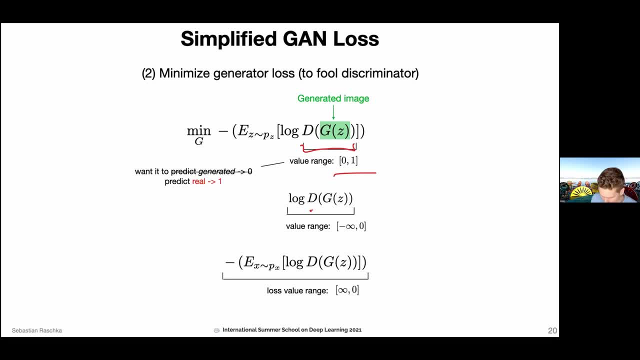 It outputs values between 0 and 1.. The log turns this into a minus infinity, So it's a minus infinity to 1 range, a 0 range. sorry, But now we are not using this 1 minus here. We are basically just dropping the 1 minus that I had earlier here. 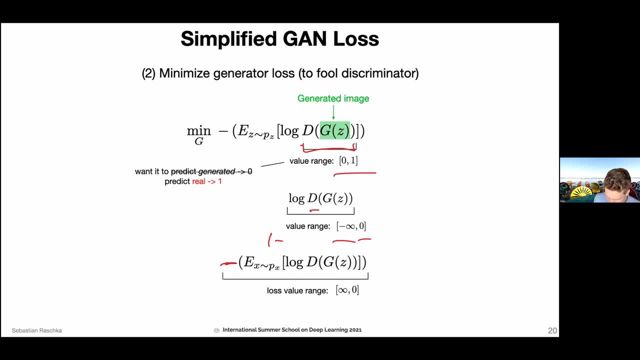 So in this case the range, if we add this minus, becomes infinity to 0. So the minus infinity turns to infinity, The 0 stays 0. So here, in this case, this is minimized, The loss function is minimized. 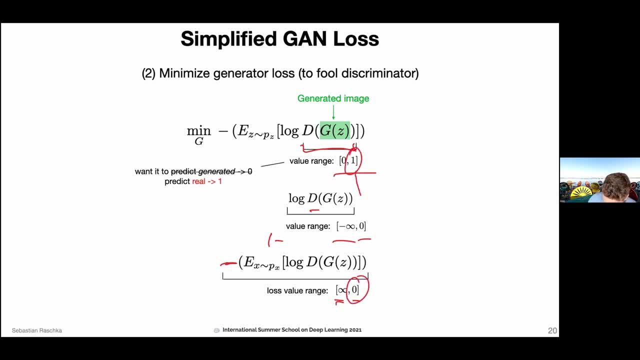 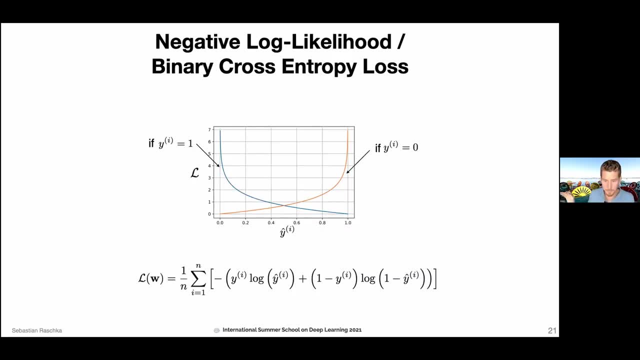 If we have a 0, this is when we predict the 1.. So if we go through here, So it would be minimized if it outputs a 1.. And yeah, this is essentially how we turn the scan objective just into a minimization. 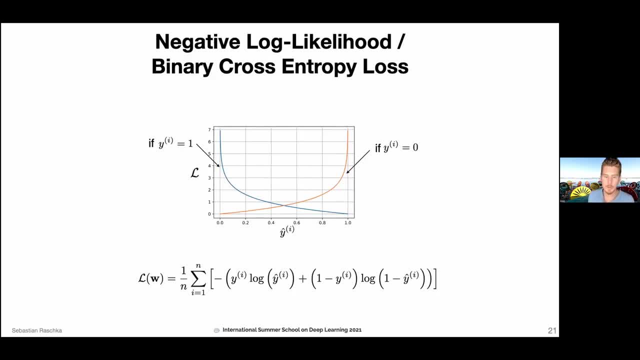 problem And if you are familiar with logistic regression, there is something called the negative log likelihood And we also call it the negative log likelihood loss And another work for that is the binary cross entropy. It's really like the negative log likelihood is more motivated from a statistics background. 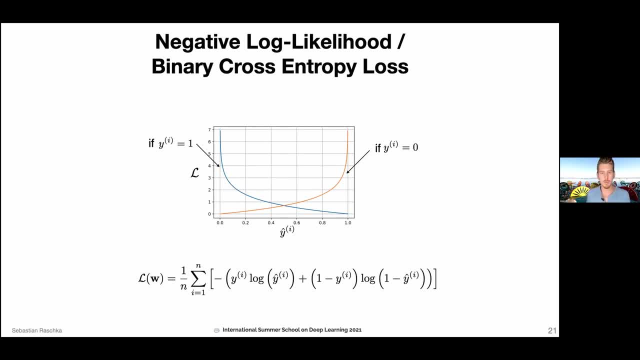 whereas the cross entropy is something motivated from information theory, But they are referring to the same thing. It's just like different fields came up with similar concepts independently and then gave it different names. So in PyTorch there's a cross entropy function that is referring to the multiple or the multi-category. 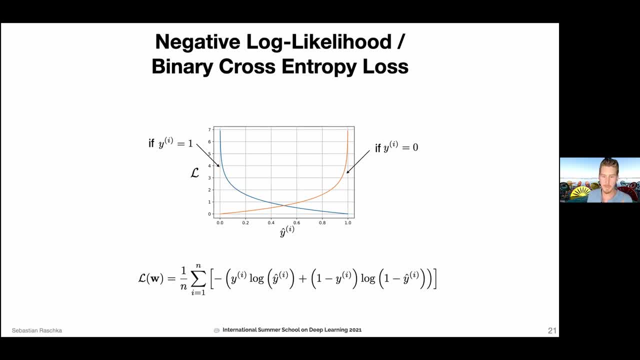 cross entropy if you have more than two class labels. But if you have only two class labels, like in the original, The original logistic regression, then you can also use the so-called binary cross entropy. So binary stands for the two class labels 0 and 1.. 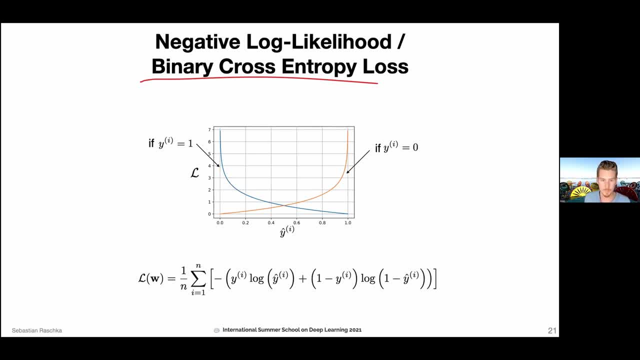 And here this plot in the center is showing the loss function, So the binary cross entropy loss function for different input values. Here this y hat, y hat i, i stands for the- let's say i's- training example, Okay, And the y axis shows you what the loss is, corresponding to the training examples. 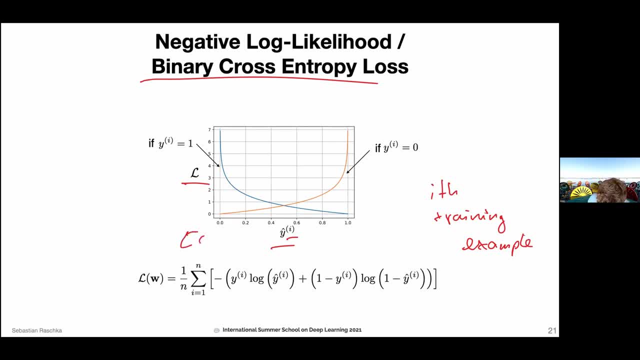 If you predict a certain value, like we said before, the values are in the 0, 1 range that we can have. And if the label the true label, why? why I? so this is the true class label? If this is one, then we look at this blue loss curve here. 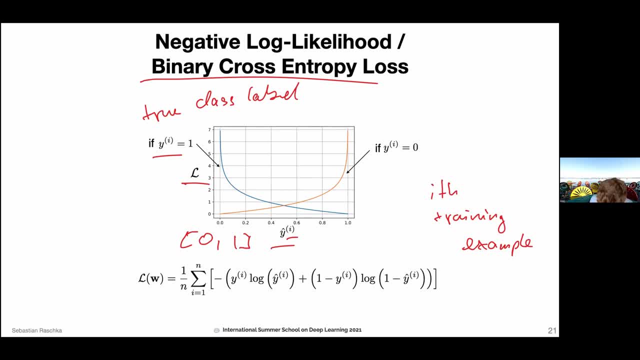 This is where the error points to. So then we we look at this one, and if it's a one, and we predict one, then the loss is zero. This is what I've shown you in the previous slide. So the loss will be zero. the slowest as it can get. 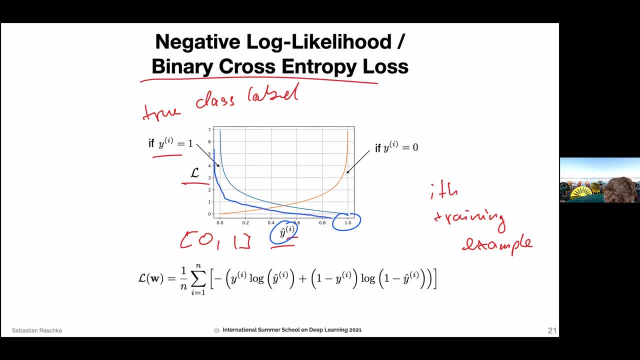 And then the more wrong we are, the exponentially higher this loss becomes. It would approach infinity here, but it would be for a very small value, I mean if we approach zero. So here I. when I plotted this, I think I used 0.01.. 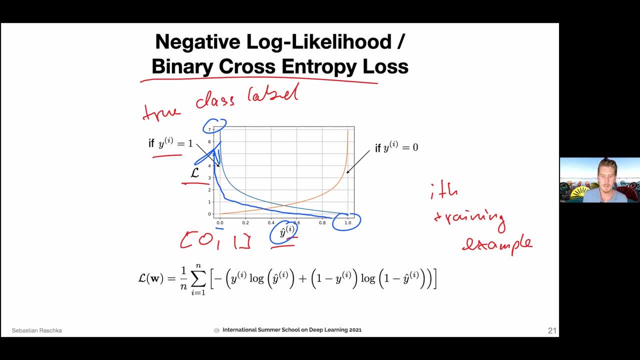 Okay, 0.01 or something, So it wouldn't crash, because I think NumPy gives you an error If you put in a lock of zero in any way. So the loss becomes higher. the more wrong we are, and the same is true here on the right. 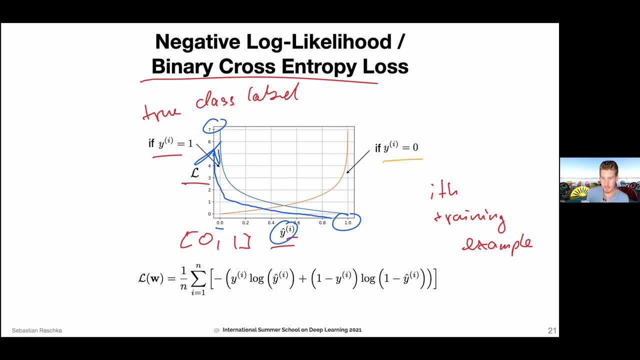 hand side. So here on the right hand side, assuming that the true class label is zero, we get a zero loss if we predict a zero. but the more wrong we are, the more. the farther we are away from the zero, the higher the loss becomes. 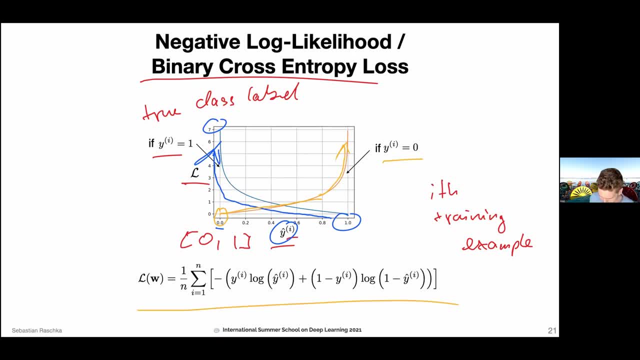 And we, yeah, we can express this And the following equation: So this loss function I'm showing you in the plot can express this in the equation here at the bottom, And this is the binary cross entropy loss. So it's this empirical, empirical one, because we also don't look at the expectation. 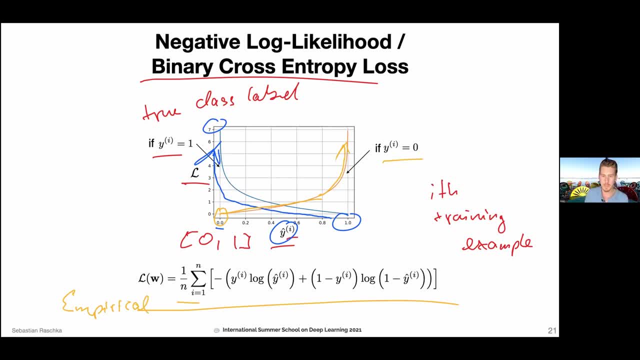 We really? you look at the discrete case where we have a fixed size training set with N training examples. What could be your batch size? If you compute the loss only on a mini batch, then this would be the N would be your batch. 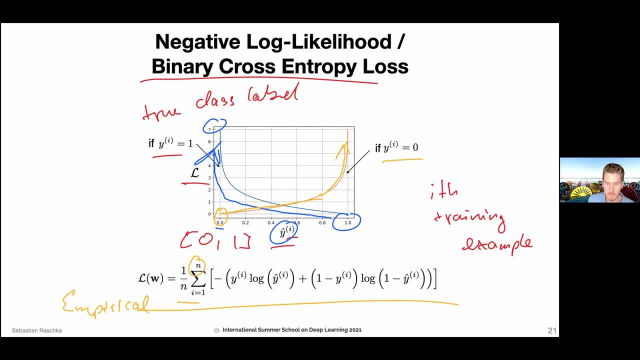 size. And yeah, we can also turn this equation into two sub equations. So the plus sign here again divides the two halves. And if we now plug in the true class table, let's say we first start with class table one, then this one here becomes one. 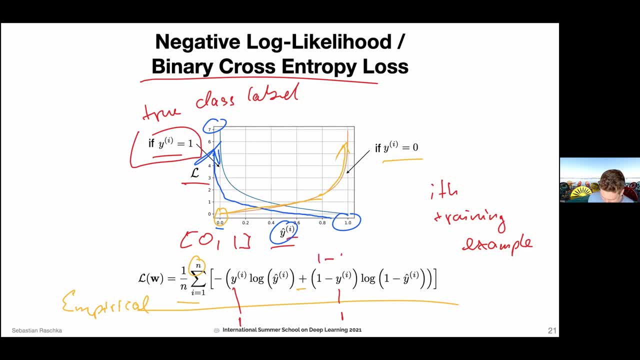 This one becomes also one, but you can already see: one minus one becomes zero, right? So then this whole thing here becomes zero, and zero times something is zero. So so this Cancels. If the classable is one, the classable is one. we are only looking on the left, at the 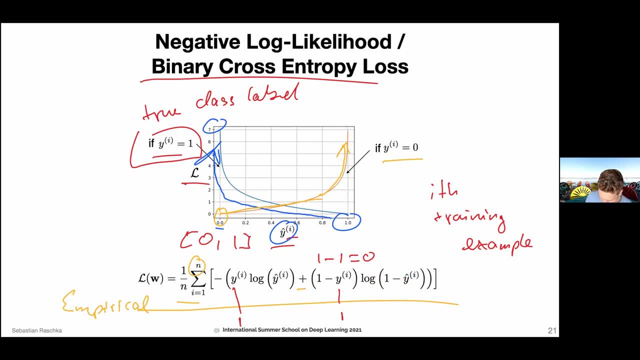 left-hand side. vice versa, If the classable is a different color, if the classable is zero, then we have one minus zero. It stays one. on this side, though, The Y I is zero because it's what we assuming. we are given a classable zero. 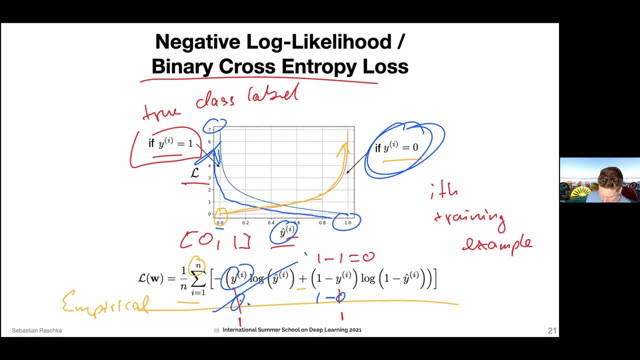 Then we have zero times something, So this cancels, and then we only focusing on the right-hand side, which is then this one becomes One, comes in block one minus Y hand, And this is the binary cross entropy that is implemented in PyTorch and TensorFlow, and 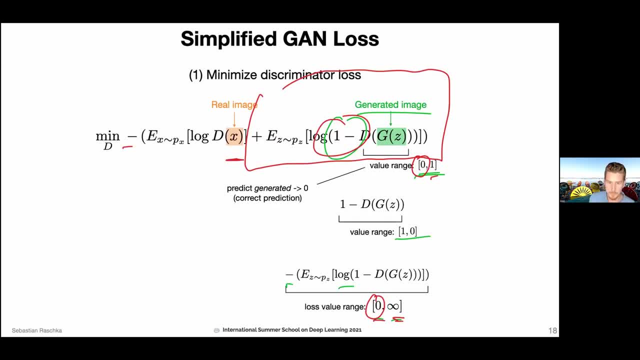 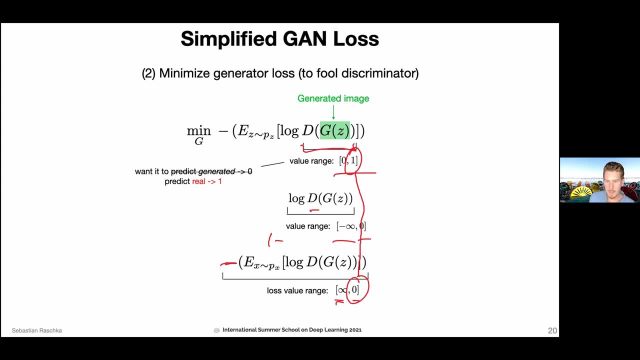 so forth. And now, if I go back a few slides, this is exactly this setup that we have. here the log one minus something And here this log of the discriminator. So you can see what we have in the GAN objective can be easily implemented using this binary. 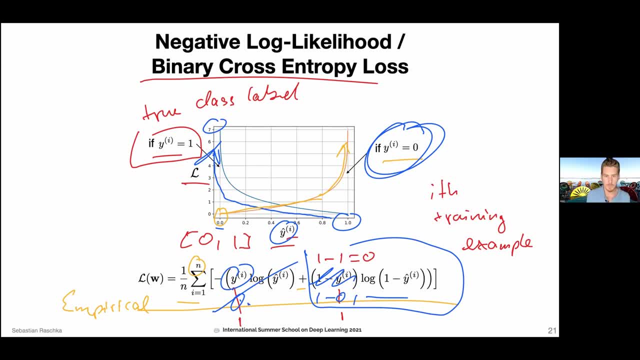 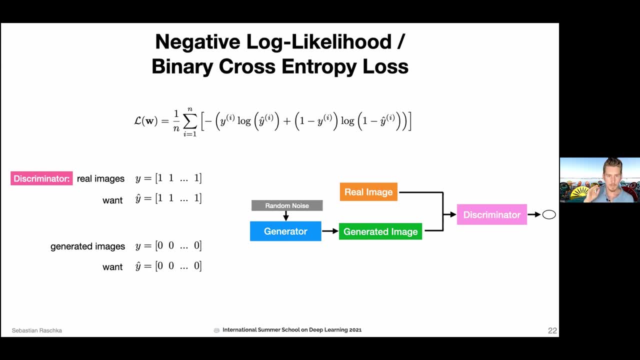 cross entropy loss. So we don't have to write a new loss function, We can just reuse what's already there in PyTorch and TensorFlow. Okay, Yeah, So then now coming back to the GAN context. So when we want to implement this, now again same as before, we use the classable one for 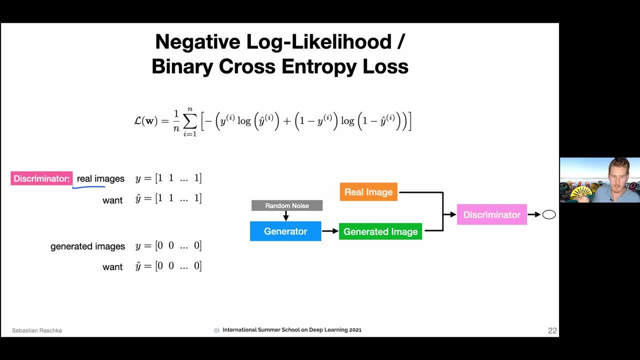 the real images. So we have a bunch of real images in the training set and we just create a vector consisting of ones And we want the discriminator then to predict for these also ones and for the generated images. we create a vector of zeros and we want the discriminator to predict these zeros. 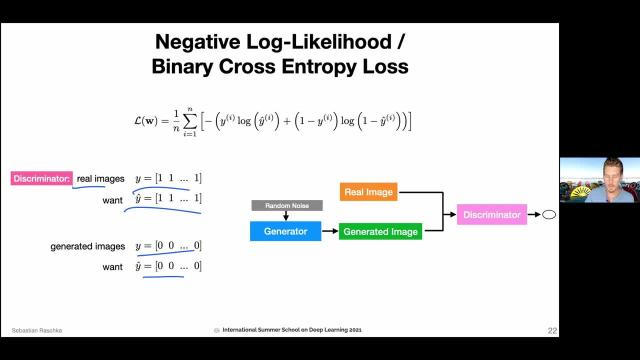 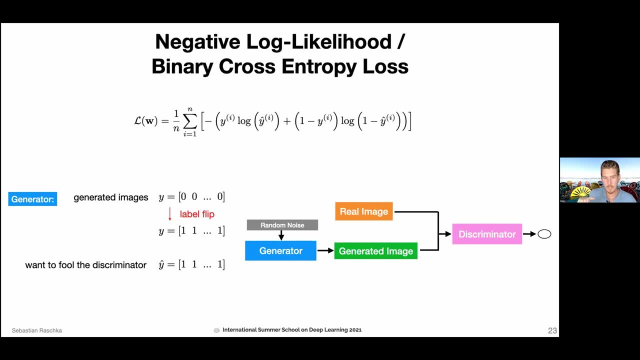 using this binary cross entropy. All right, So, and for the generator, there's a little trick. So what we do is we just, in order to fool it, we flip the class tables. So we have, I mean, we have created these before, right. 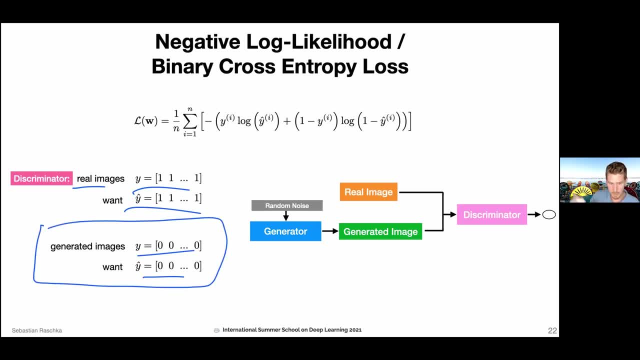 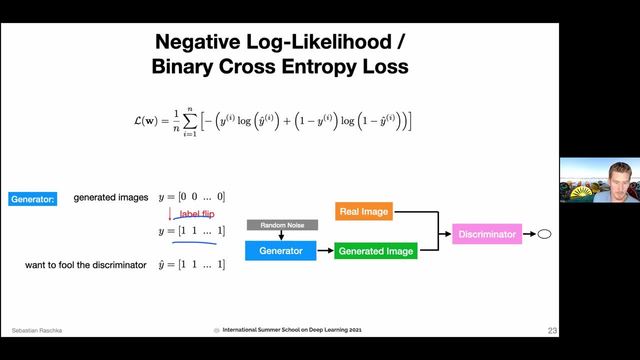 So here we have created the vector of zeros for the generated images. Now we just flip them. So we flip these class tables to classical one and then train the discriminator on that. So it learns, kind of it learns to predict. the wrong Thing for training the generator. 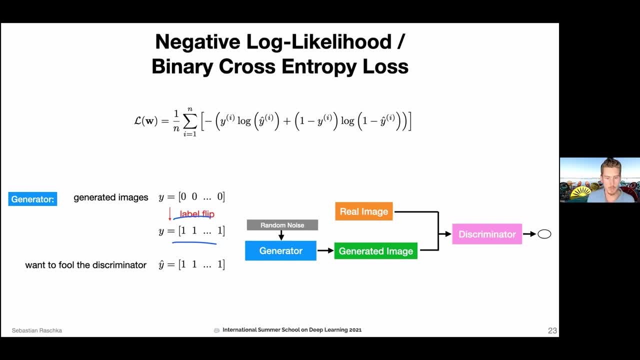 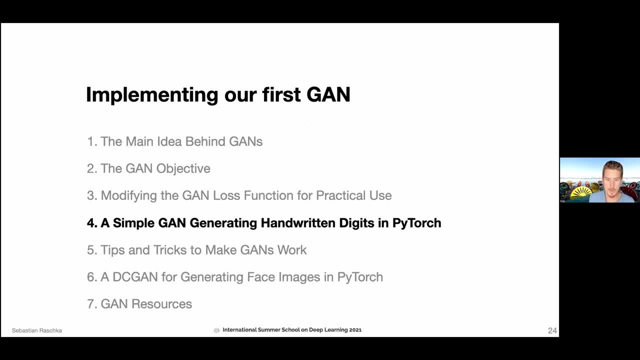 Okay, So this is exactly like before. this is just how we would then implement it in code. So I have prepared a code example, like just implementing these concepts that we have talked about, but, of course, PyTorch, also TensorFlow- they are involving a lot of code. 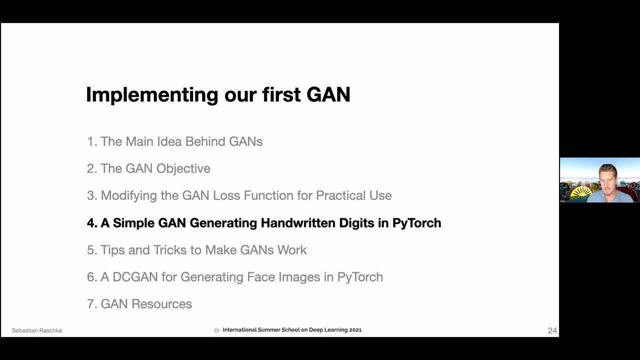 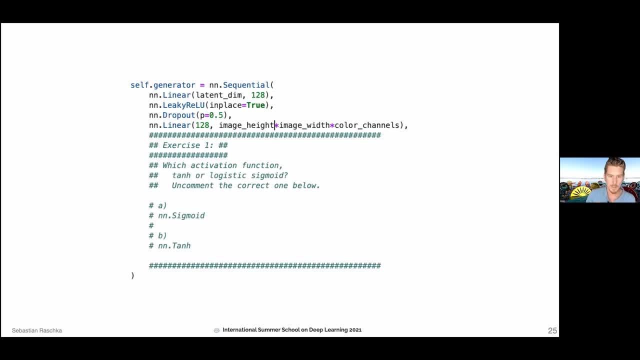 So it can be hard to find, let's say, the needle of the haystack, the parts we are looking at. So I will walk with you together through the code example and then I have a few exercises, So I will just show it to you very briefly, but they will be in the code. 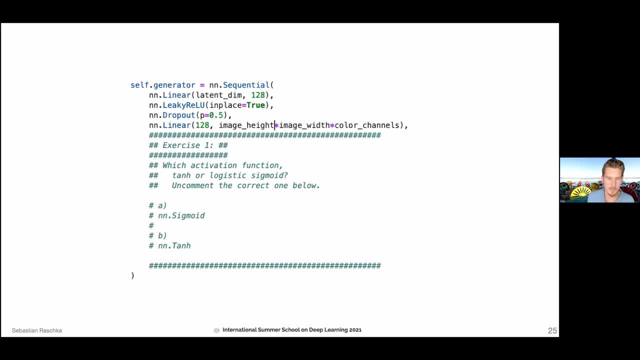 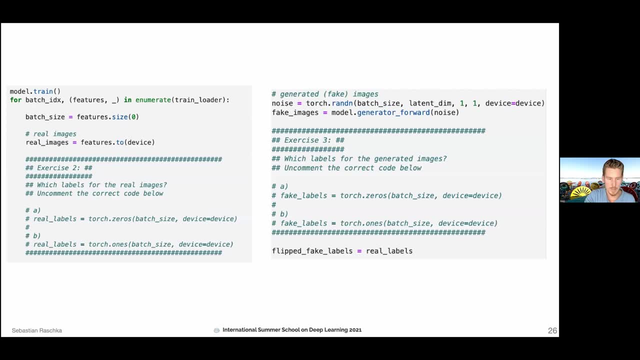 So you have the like 15 minutes to think about the solution here, And so there's exercise one, two and three. they are just comments, And your task would be essentially to, instead of writing code from scratch, to uncomment the correct one, whether it's A or B. And I thought it might be simpler because if you 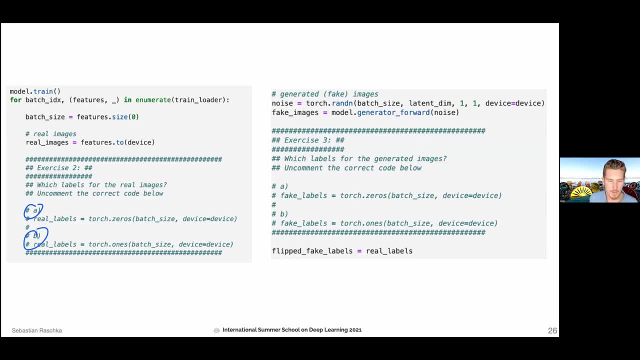 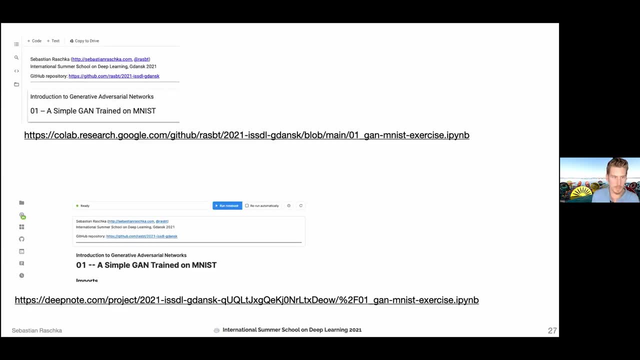 have not used PyTorch extensively before. I think writing PyTorch code can be a little daunting, So I wanted to give you a little help and a little template here. Okay, So the code example can be found. I uploaded it both to Colab, Google Colab and Deepnode. 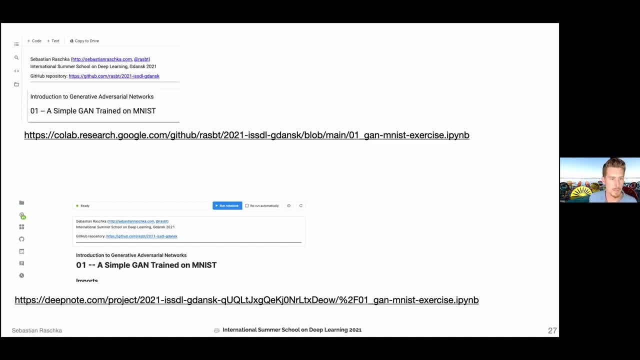 which is the same thing as Google Colab. but just in case one of the two doesn't work, you have the other one, And I should probably post these links also in the Slack channel and here in Zoom so that you can just click on it and it should open. 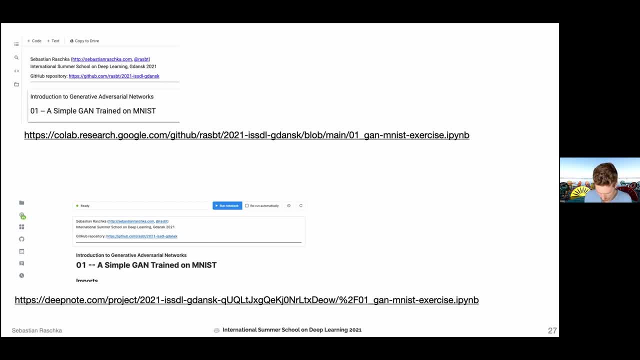 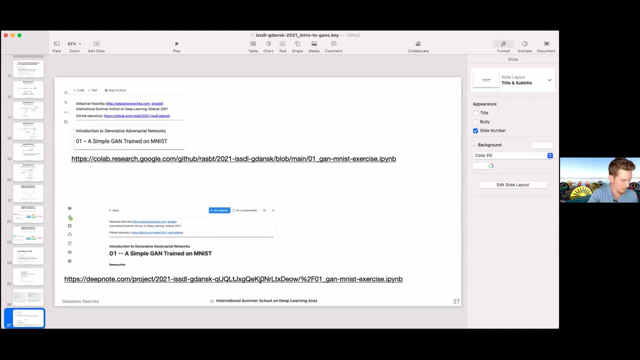 So maybe let me just do this right now. I think let's see. Okay, One second. Okay, We'll just copy these links. Let me share them in Zoom, because I am assuming everyone has it open. Well, I'm actually not sure how to open the chat window, because I don't want to accidentally. 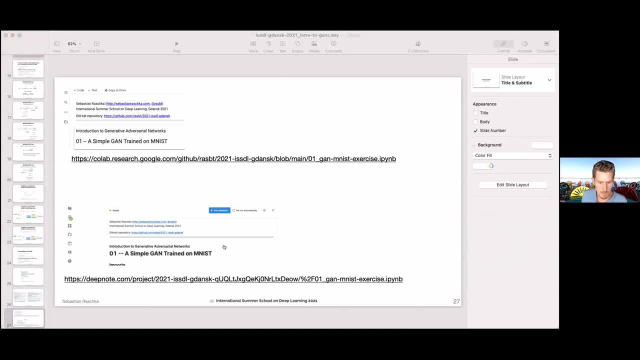 close this here. Let me share this in Slack. Okay, Great, Great, Okay, Thank you for that. So let's see. Okay, So I'm gonna show you in the Q&A. I will just go back to the Q&A session just to handle. 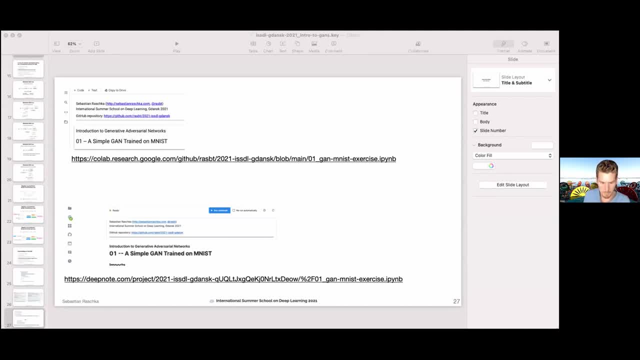 all the questions I have. Okay, So let's see how this works. One second Okay. So let's see One second Okay. So now I am doing a little compilation video. One second, One second Okay. 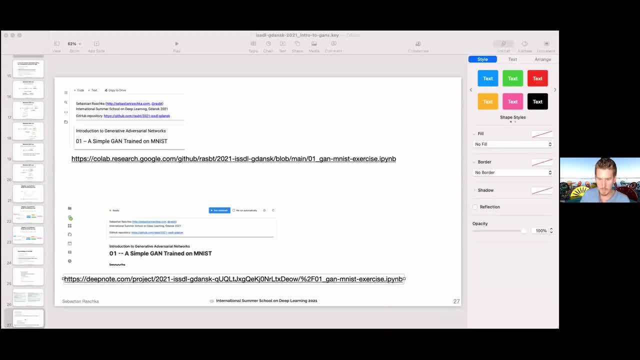 Let me just go ahead and let's continue with the discussion. So yeah, your exercise would be now to look at the code and then try to answer some. try to answer the questions, or I'm coming with the right code, but I can walk you through the. 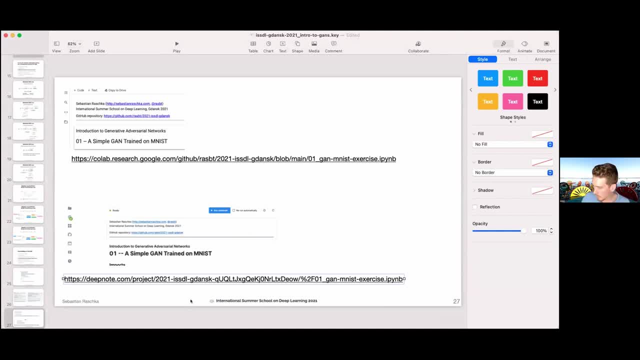 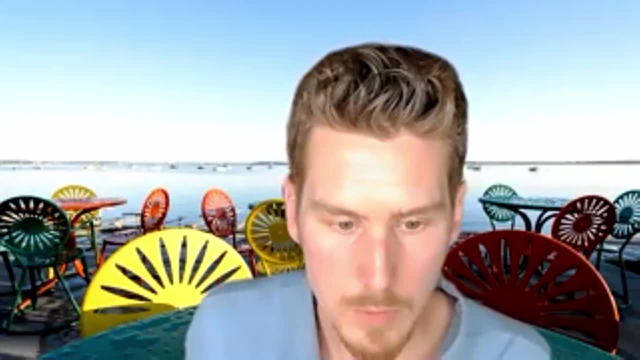 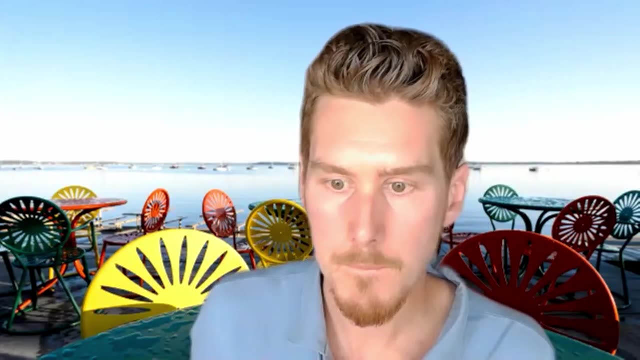 code example. let's say 10 minutes and then you have 15 minutes to do the code example. so let me also open this notebook now. you have to change my screen sharing to my web browser now. I think this should be it. can you see this? um at all. 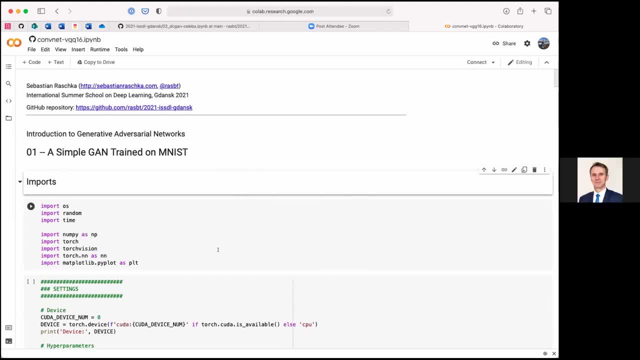 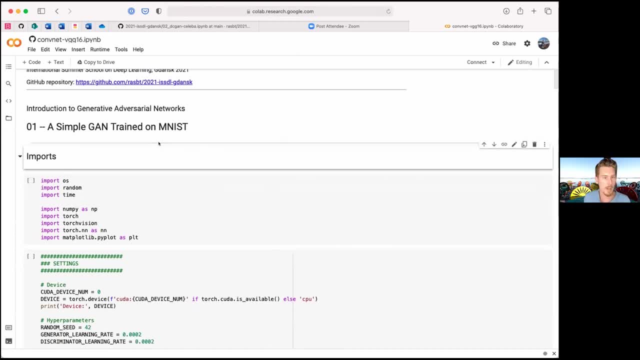 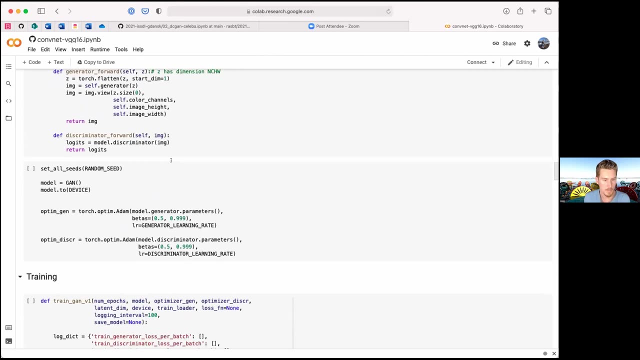 we can see the notebook. perfect, okay, so this is a very long notebook because there's a lot of boilerplate code required, um for loading the data set. so if I just scroll through this you can see there are a lot of things to it. so, um, lots of code. this is just for observing the training. 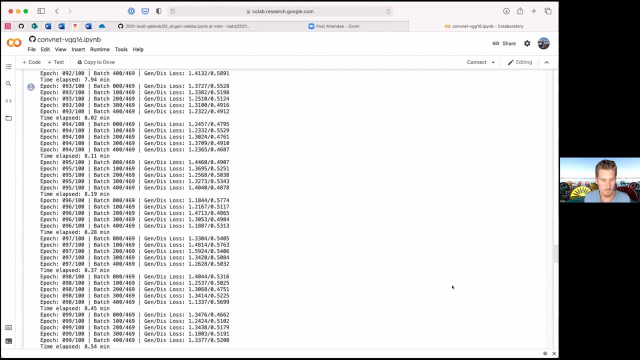 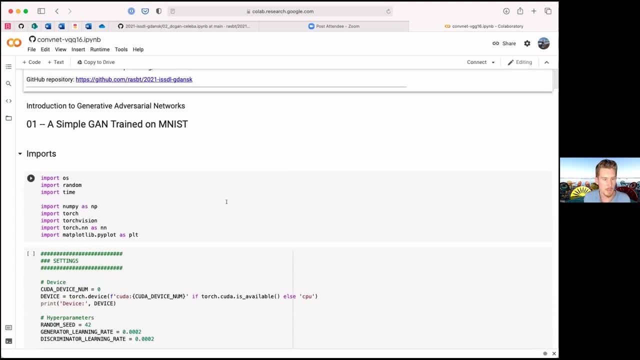 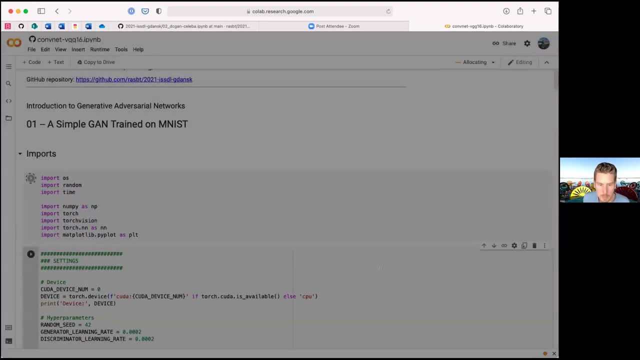 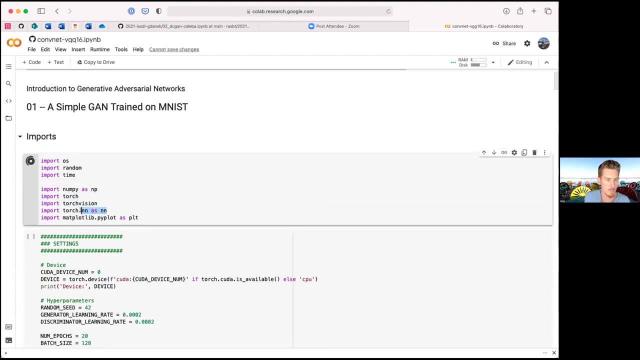 and then in the end, evaluating the results. so starting at the top, um, starting at the top. so here this would be importing just some um libraries we will we are using- oh okay, I do confirm so- just importing some libraries we are using, like torch vision, torch um. here this is just a shortcut- matplotlib for plotting and numpy for some other things, and 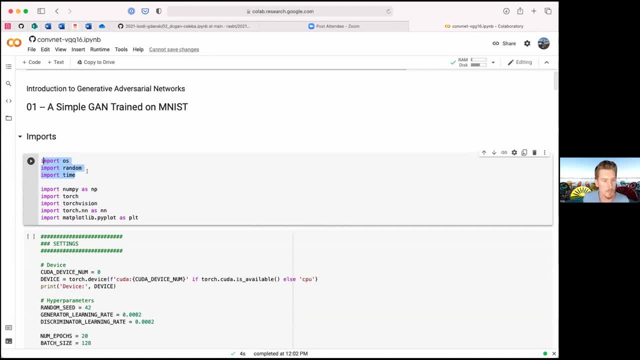 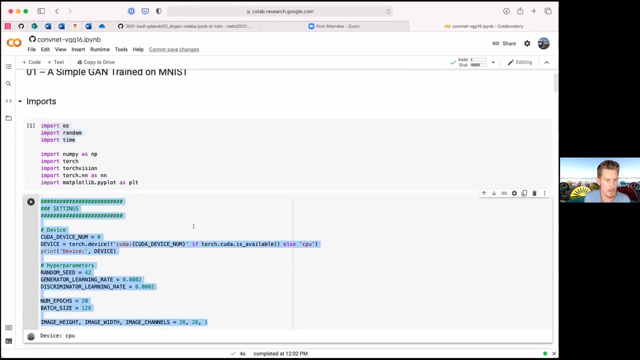 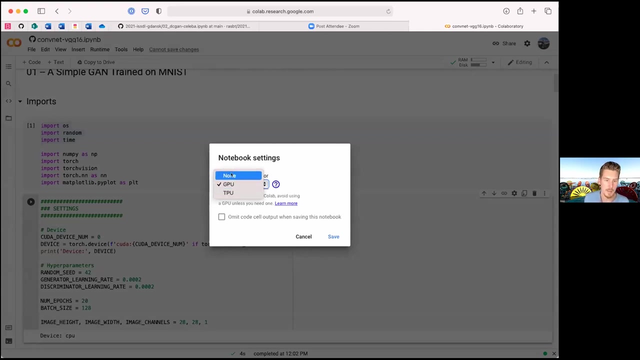 these are python standard library, um things, okay, and here are just some general settings so you can run this code either on the cpu or the gpu. so if you are using google collab, you can go to runtime, change runtime type and then select cpu. actually you can't select cpu anymore. interesting gpu or tpu, I think. none means cpu. okay, so gpu will be a. 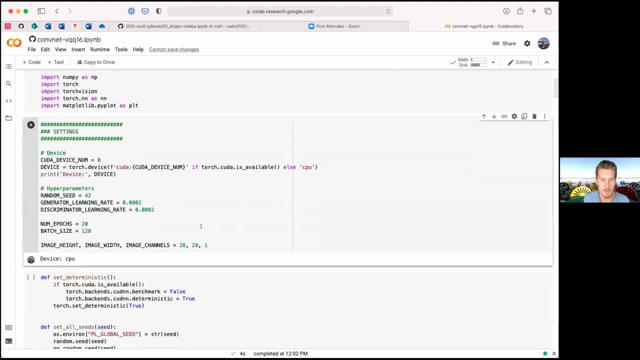 little bit faster, of course. um, yeah, so then some hyper parameters. of course, the random seed, it's maybe something you shouldn't tune as hyper parameter, but, um, the learning rates of the discrete and the generator are, for example, hyper parameters, something you have to tune to find a good one so that the network runs well. 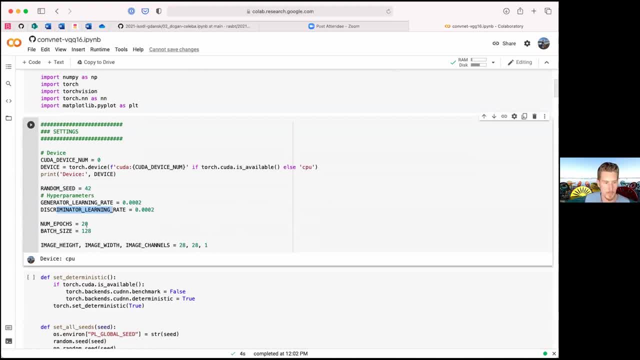 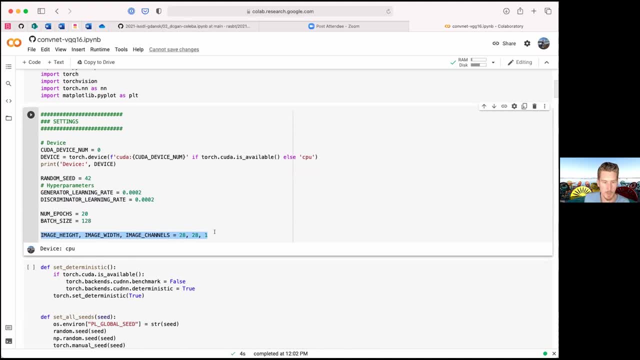 it's the same concept as with a regular convolutional network: the number of epochs and the batch size and then also the image dimensions. it's just some general settings here. um, we are working with the MNIST data set, so they are 28 times 28 dimensional and there's only one color channel. 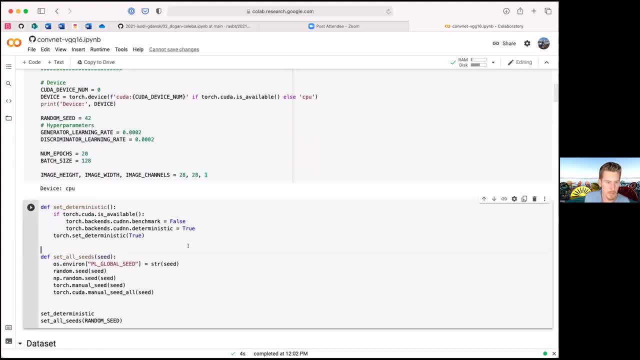 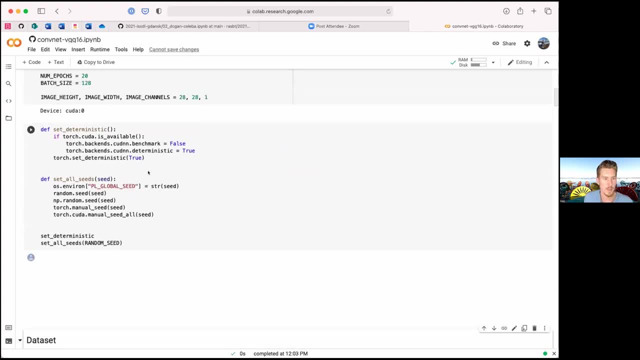 because they are grayscale images here. these are some functions I've used in the last few years personally like to use- um, okay, I should probably execute them before I can execute that. so these are just some some function I personally like to use because they make the code. 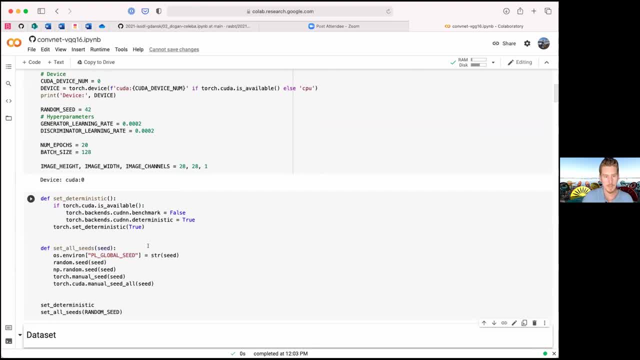 deterministic. that means if someone else runs the code they will get exactly the same results. because by default if you use the gpu, um nvidia, the cuda library, um determines based on your hardware, based on the computer, which um convolutional uh layer function is used. so there are in the library multiple ways to compute a convolution and they should give you. 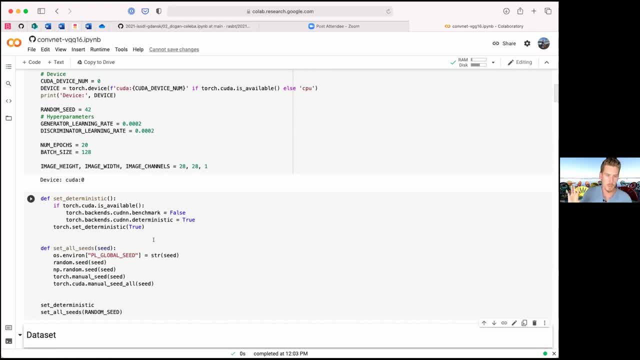 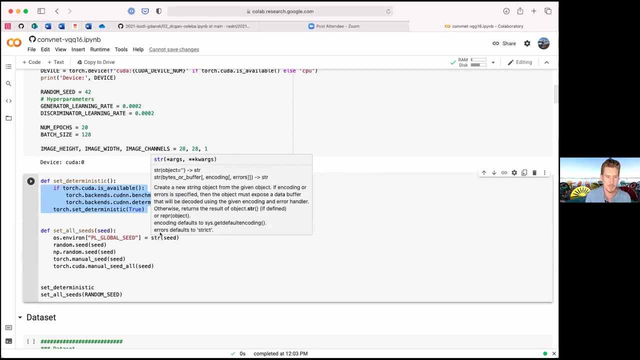 identical results, but there are some rounding errors and approximations. so on different computers you can get different results, and if you run a network over the course of training you can get vastly different results, and so I personally like to fix this so I can reproduce results. but um, it really depends on which context it's mostly if um for research I, for example, if 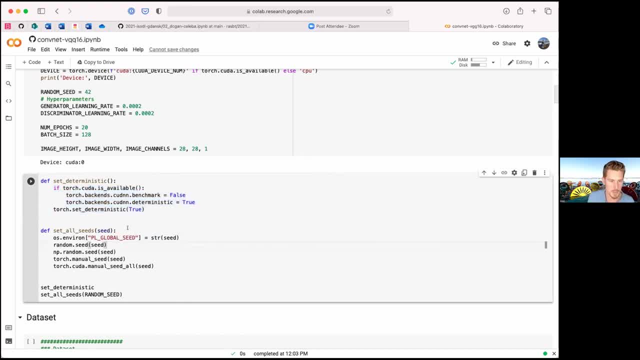 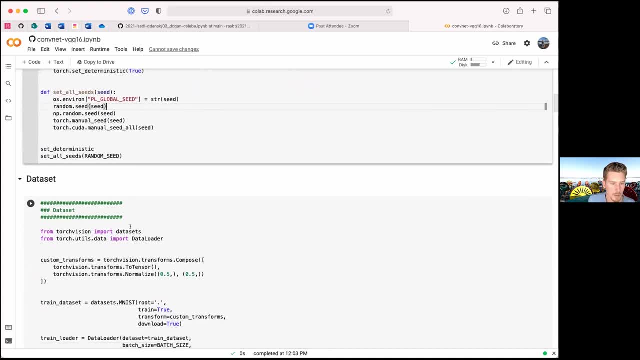 someone asks me to confirm that the code is correct, I can reproduce the same results. that's why I'm using it, but it's not super important in this context. here then we are loading the data set here, so this is the mnist data set we are working with, and 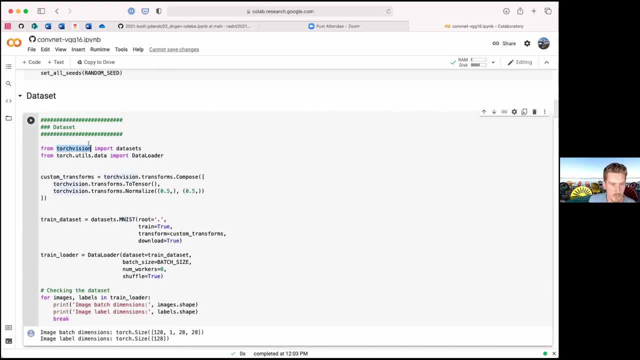 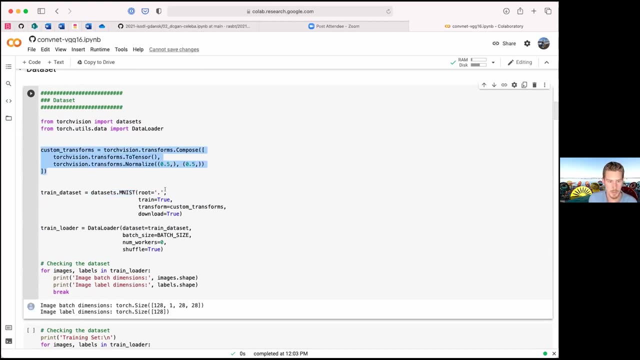 mnist is already implemented in pytorch and- sorry, in torch vision, which is a torch library or pytorch library for computer vision, and we are loading, importing these data sets here and um, we are just using it from there, and this is here a normalization. so what we do is 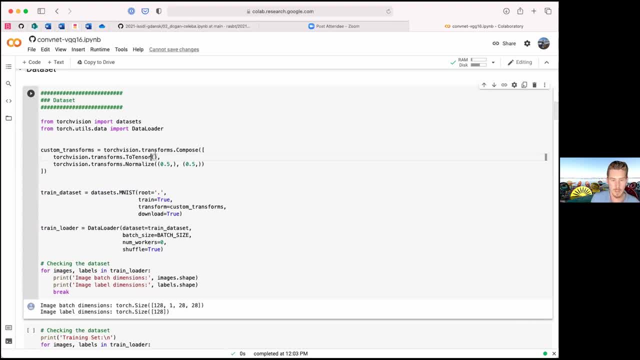 we. so what happens is it will load the images as pil python image library images, and the two tensor method converts this into pytorch tensors automatically. and in this function here what pytorch does automatically is convert everything into the zero one range. so pixel images are usually in the range between zero and 255. but this two tensor 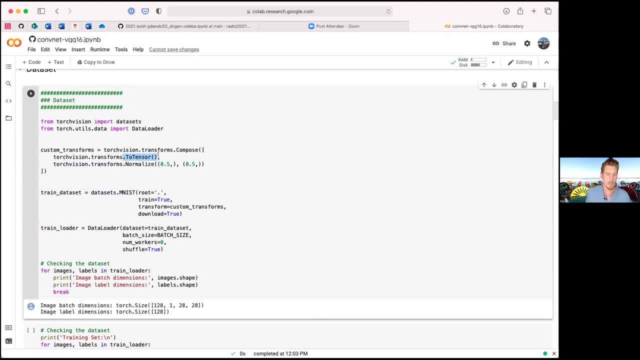 will convert it to zero and one. it can be a little better for performance optimization reasons. like we can say that the pixel value is one percent performs better when things are centered at zero. so we can achieve that by standardizing or normalizing these images. so here the first. 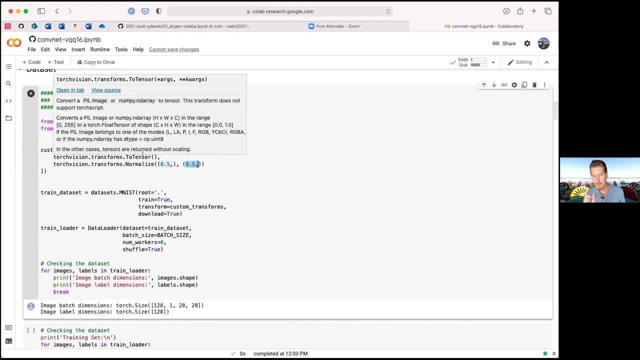 value stands for the mean and the second for the standard deviation. so if I have something in the zero one range, let's say I have a pixel value of zero, standardization would subtract the mean, so it would be one minus 0.5. can we write this down: one minus 0.5, which will become: 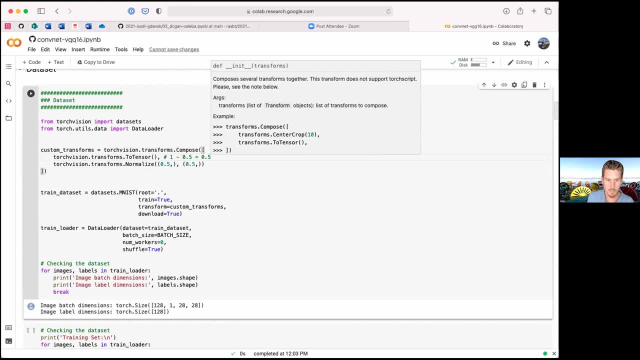 it's one minus 0.5, this will become 0.5, right, and then it's dividing by the standard deviation. so it will divide 0.5 by 0.5 and the output range would then be one. now, if I have a pixel value of, 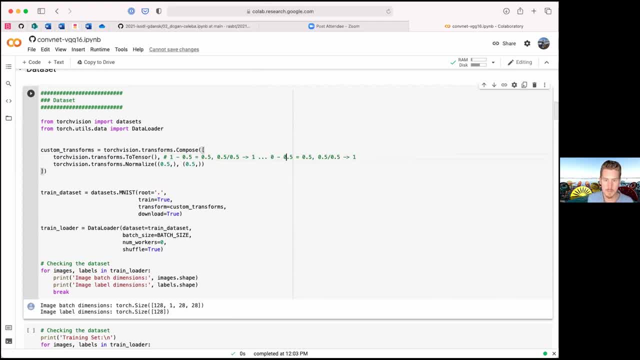 of zero. then we have zero minus 0.5, which is then minus 0.5. oops, and then minus 0.5 divided by 0.5 is minus one. so what this will do? this normalization will normalize the pixels such that they are in minus. 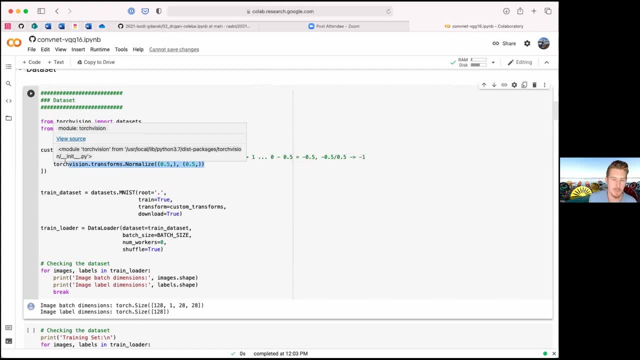 one to one range. it's very a little. maybe I'm going into too much detail, but this is like a little aspect you need to consider when implementing it. again, you have to know the pixel range, because the generator is supposed to generate images and if you want to, yeah, when we 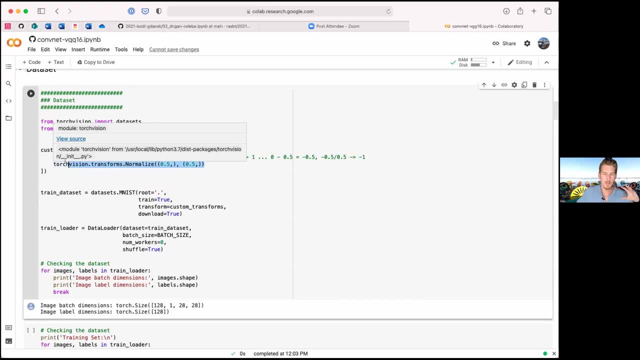 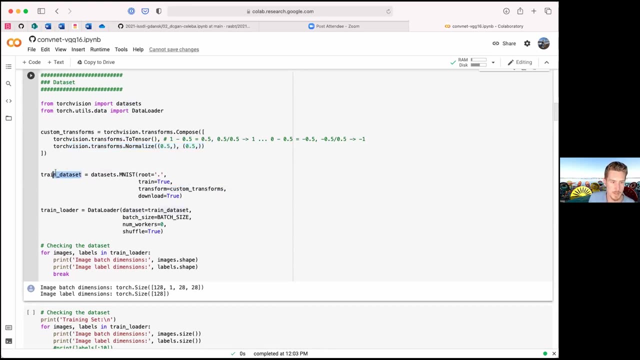 want the discriminator to make a good prediction, the training set images and the generated images should be on the same scale, right? so this is like a minor but important detail. So we are passing this custom transformation function One. also one thing to say is we're only using the training set. we are not using the test set or validation set, because 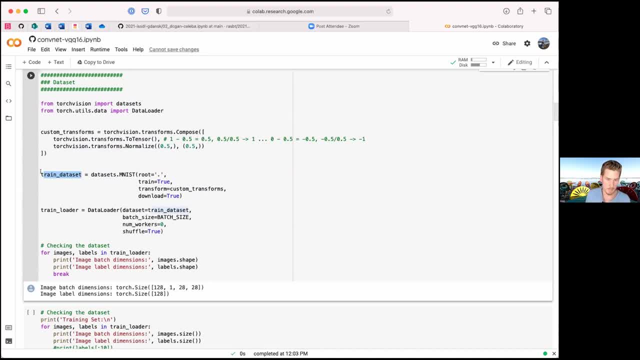 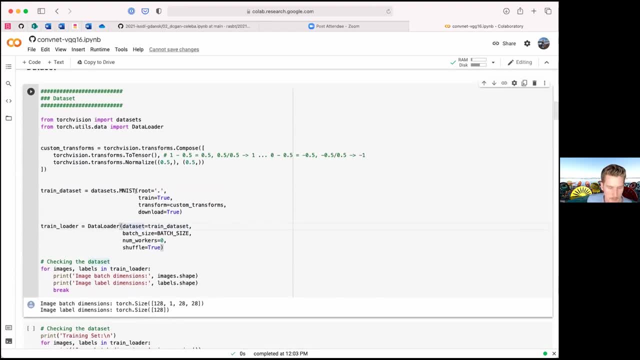 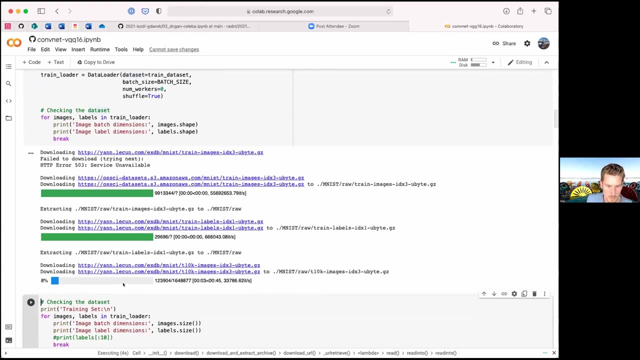 it's an unsupervised approach. here We are generating data. We don't want to classify anything in the training set. I think this might take a few minutes to run. nowadays It's made faster, I think, on how busy the server is. a lot of people are downloading the MNIST dataset, So sometimes 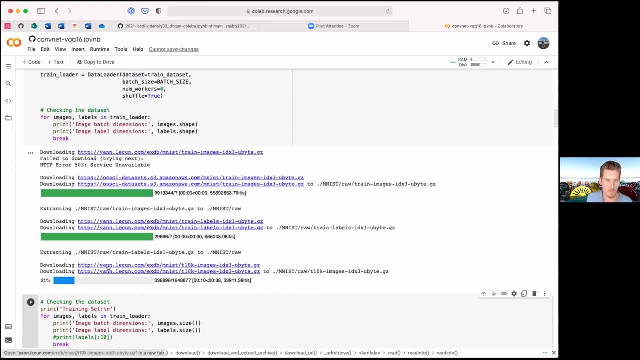 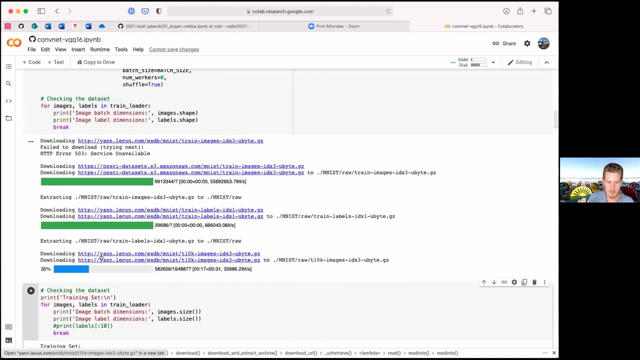 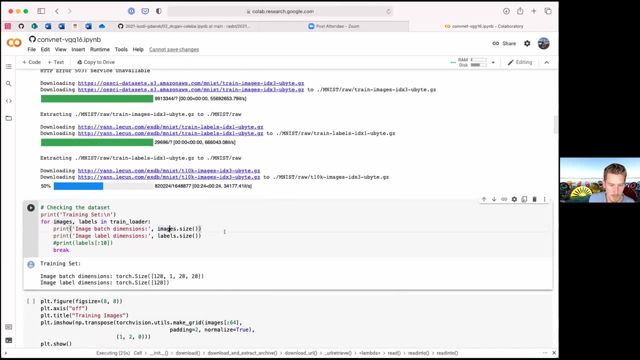 the server from, I think, Yanli Kun. his website might be a little bit slow sometimes if a lot of people download things, So Yanli Kun was the person involved in collecting the original MNIST dataset. I think it was in the 1980s And here this is just checking the dataset I like to do. 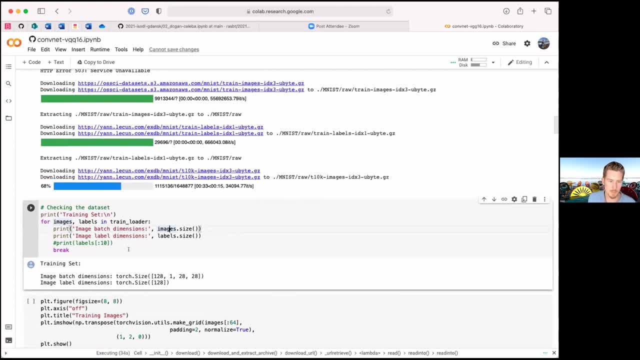 that just to make sure everything looks like as it should be. So we chose initially a batch size of 128.. And we can see when I print the size here: the batch size is 128.. There's one color channel, 28 pixels image height and 28 pixels image width, And there are the corresponding class tables. 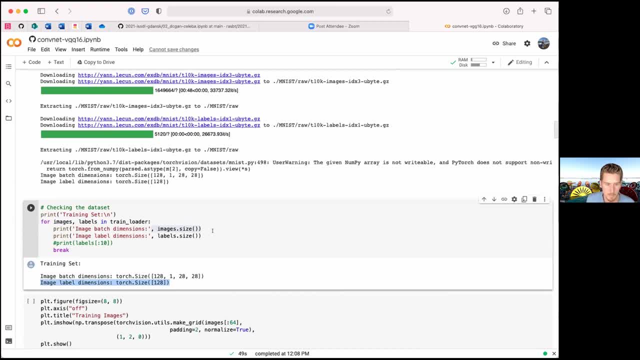 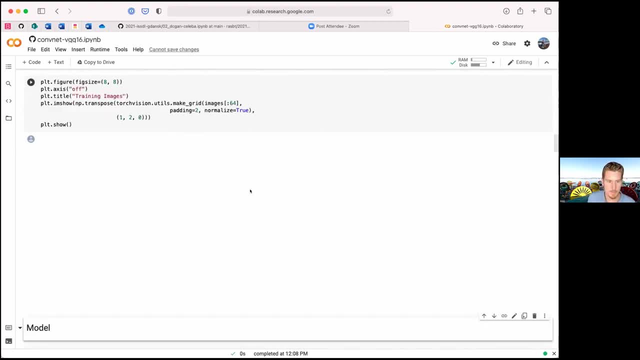 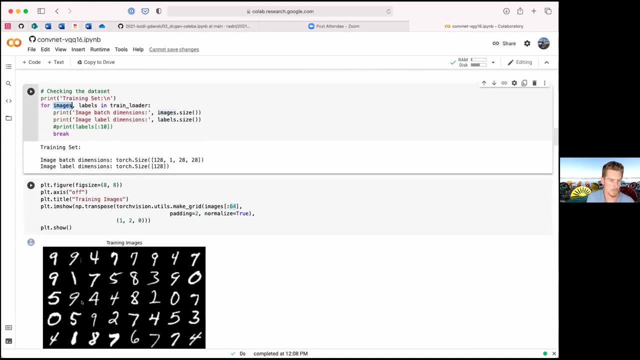 but we are not using class tables. I just printed them here, but we don't use class tables for GANs. He, I'm just showing you a random selection of 64 images from the first batch, So from this first batch here I loaded, So just to take a look at how they look like. And here's our main GAN now. 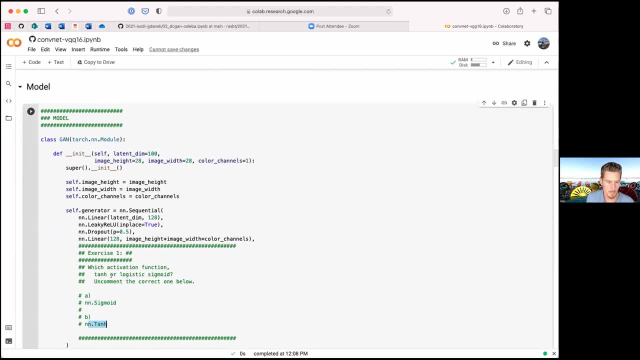 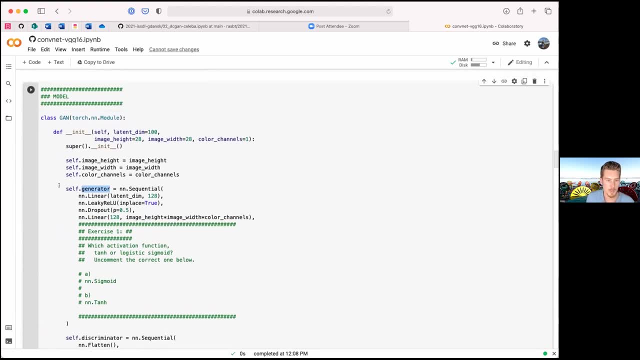 So this is our GAN. There will be an exercise for you whether we use sigmoid or 10H here for the generator, And so how this is organized is I organized it into two sub-networks. This is using Torch and NModule to make a neural network, And then we have a generator here. 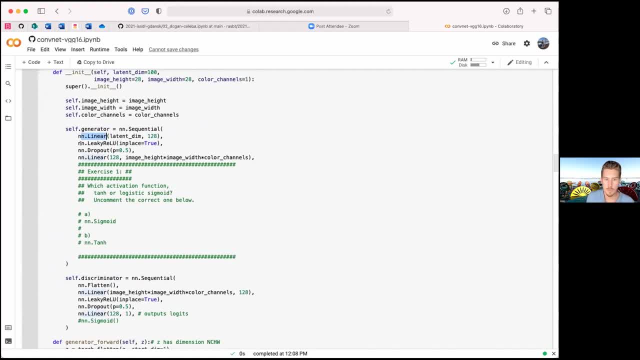 And then we have a segmented layer and a discriminator. So there are several layers. a fully connected layer- It's called linear in PyTorch, A liquid ReLU. This is like a ReLU function but with a small slope in the negative range I'm using also drop out, And that's about. 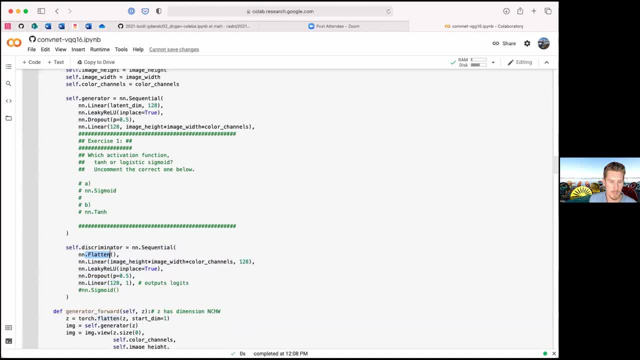 it, And I'm doing the same thing here for the discriminator. There's a flatten here because the discriminator receives an image of MNIST but a fully connected layer, a vector. so i'm just reshaping the 20 or the 1 times 28 times 28 image into a 784 dimensional. 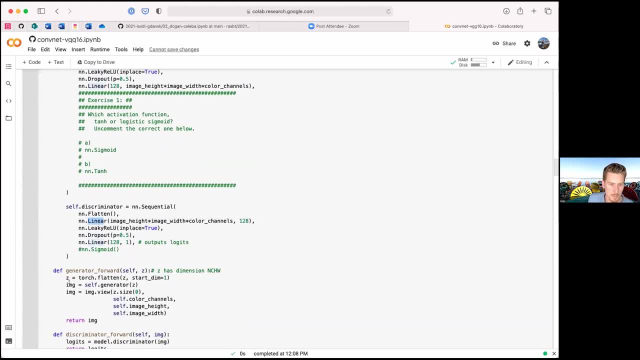 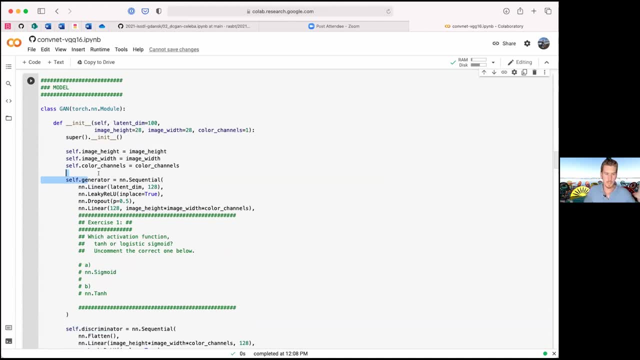 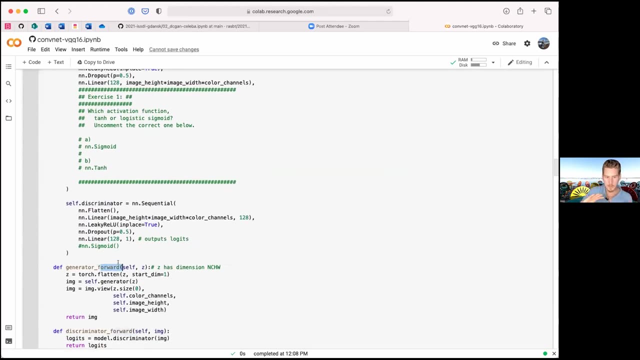 vector, essentially so, and for the generator. so i here and here i define these networks. so here i'm just saying what layers we want and what the parameters are, and here, in the forward method, these are the instructions or functions to execute that code. so these are essentially executing it. 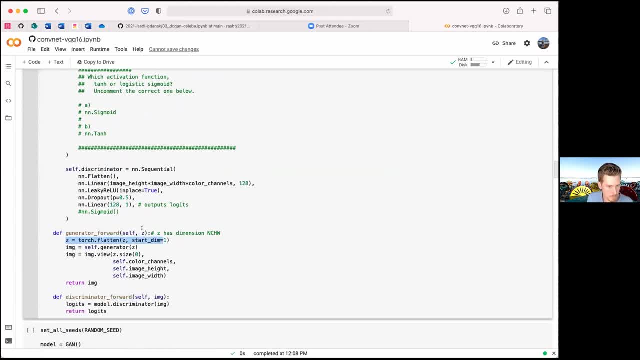 so here how we executed this: we flatten the input, so we have z, z. i made a novelty to myself. it has the dimension nchw. so n stands for batch size, c is for color channels, h is for the height and w is for the width. so it's just like this. it's a matrix, a tensor, a four-dimensional tensor. 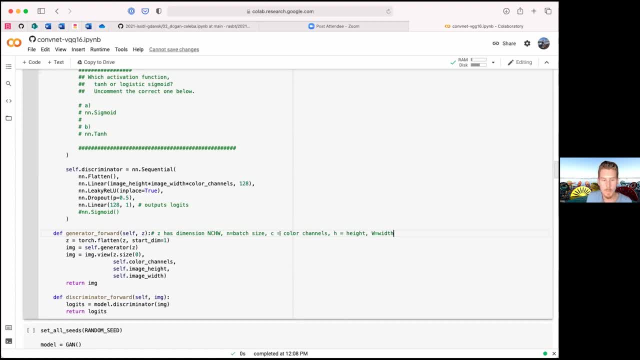 um of n times c, times h, times w, and this is because i implemented this gam dc again for the face images which i will show you later, and i have the same training function. i just wanted to reuse as much code as possible. this is why um, the training function, will feed this one an image, not a vector. 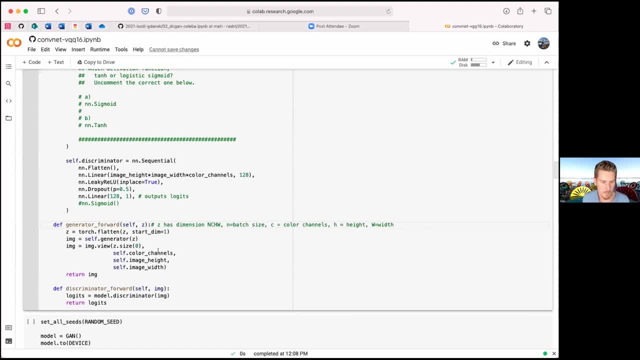 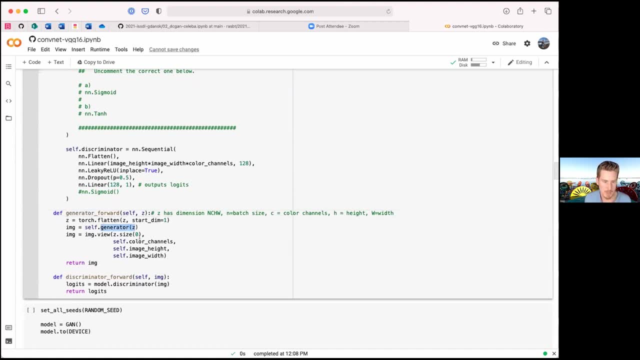 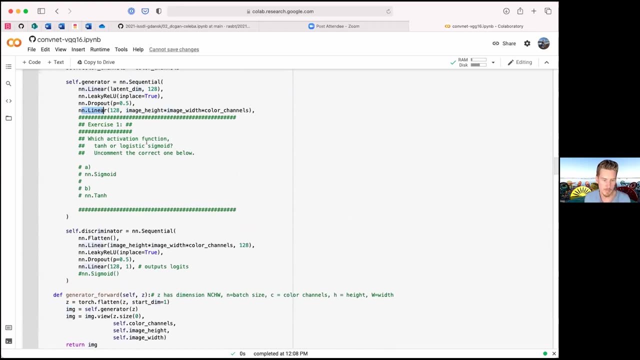 but yeah, we will see that later. why? why that is? so don't worry about these details at this point. and what happens is then the generator receives this noise vector z outputs this image and then the image- because this is the fully connected layer- is a vector and we are just reshaping it again to get 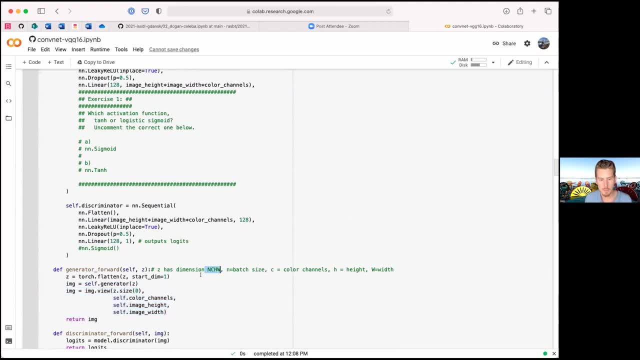 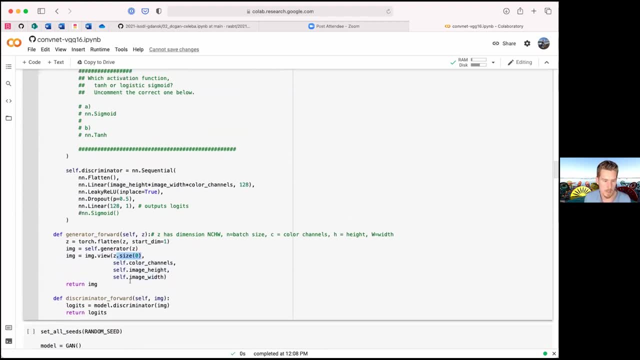 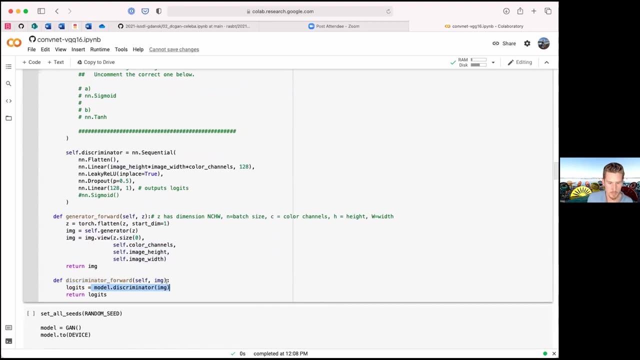 back an image in this nchw format. so color channels, height and width, and then z, zero size, zero is the batch size. now here is the discriminator forward method. so the discriminator forward method is the um, just running the discriminator and it outputs the logits. so the logits are. 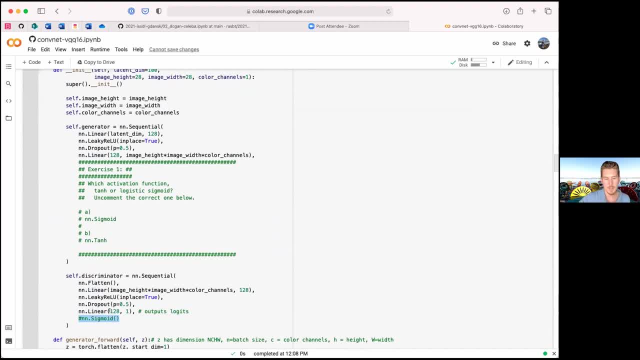 here on the outputs. so it should be a sigmoid function because, like we said, it outputs the zero and one or the range. the output range should be between zero and one. i removed that. i uncommented this because that's how the loss function pytorch works. so there's a loss function cross entropy. 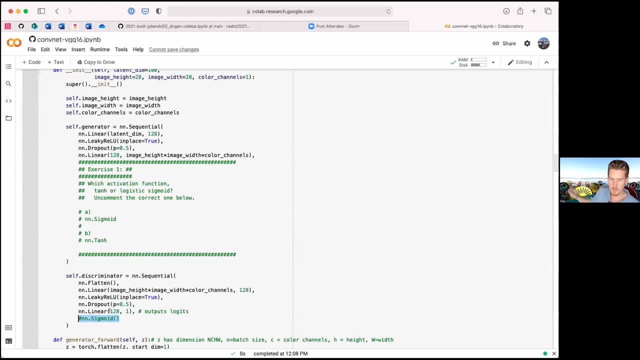 and a loss function called binary cross entropy with logits. so this one expects- or both of them expect- logits instead of the sigmoid, and this is just for um stability reasons. it's to um stabilize when you compute the gradients, like for numerical stability. there is also a function. so there's um a function and l l. i think it's called an l loss or something. 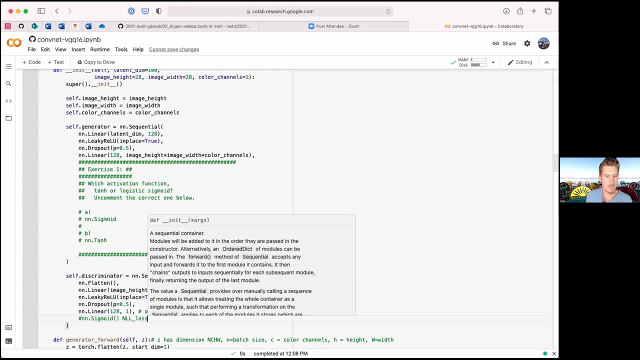 like that and l could be like this in smaller case letters. it stands for negative log, likelihood loss, the binary cross entropy, but this one would expect the probabilities, the sigmoid, so it's just like a minor, minor implementation detail. so the binary cross entropy conceptually works with these. 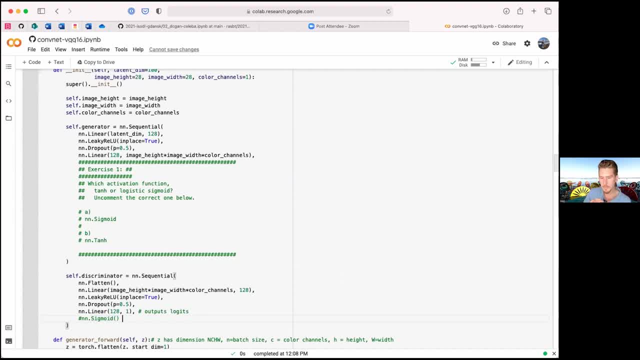 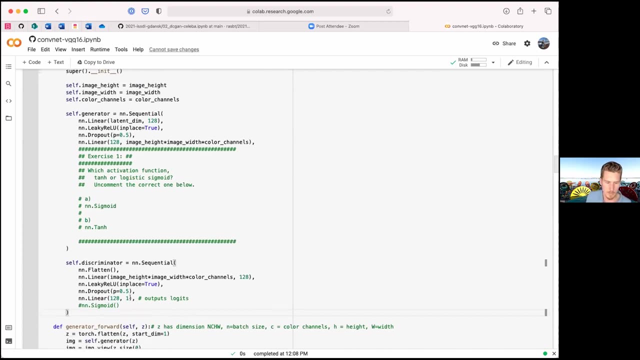 probabilities. but the way it's implemented in pytorch is you provide it with the logits for numerical stability and internally so the function, the loss function itself, will do the sigmoid for you. so if we would call sigmoid here, it would basically call sigmoid twice, which is what we don't want. 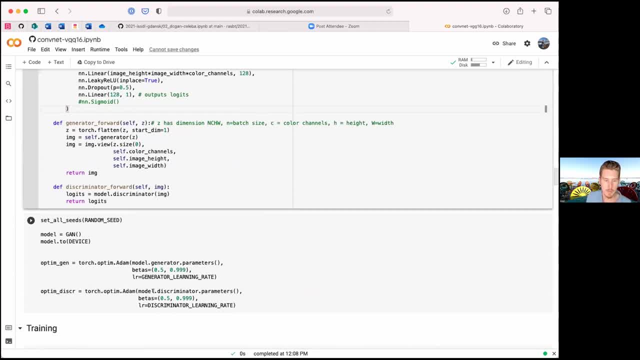 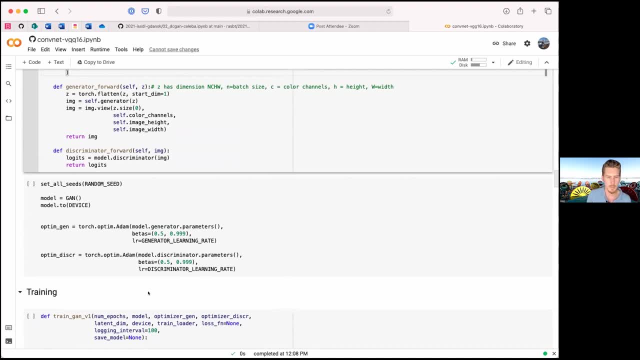 or don't need, because then the gradients would be a little bit small, because the gradient i think, uh, in sigmoid, if it should be the largest gradient we can get, i think it's 0.25. so if you have 0.25 times 0.25, it would be unnecessarily making the gradient small. 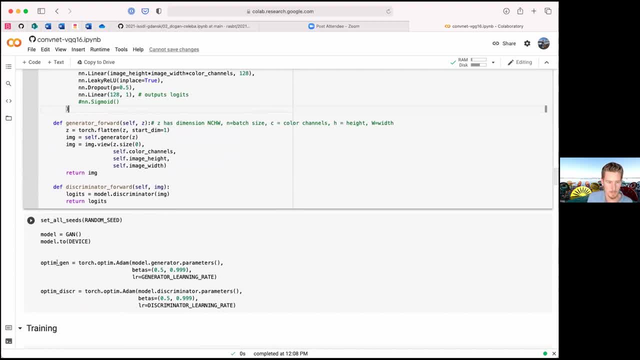 all right. so this is our model and now we define some optimizers. and this is the tricky part i mentioned before, where we have to be careful that we want to freeze the networks when we train the other network. so if we train the generator, we want to freeze the discriminator. 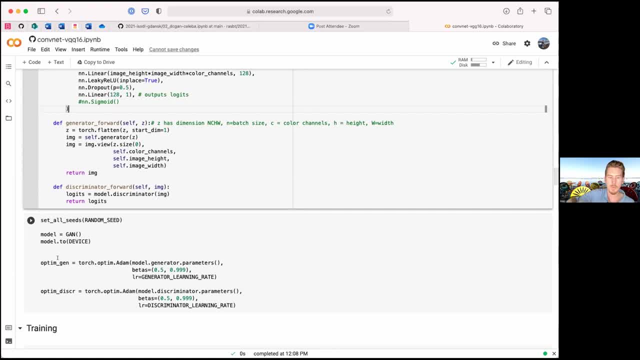 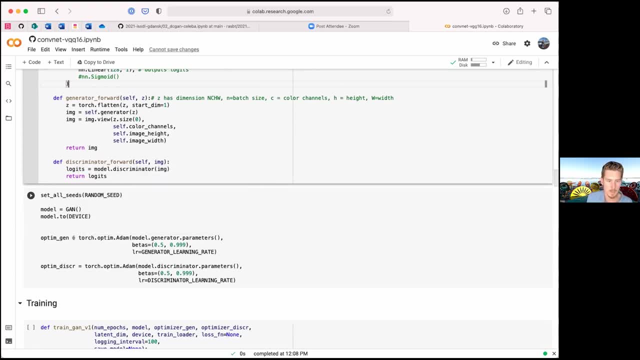 and which we train the discriminator on the generated images. we want to freeze the generator. in practice this is very simple. in pytorch we just use two distinct optimizers. so we will use one optimizer for the generator and we only give it the generator parameters here and then we have an optimizer for the discriminator and we only give it the discriminator parameters. 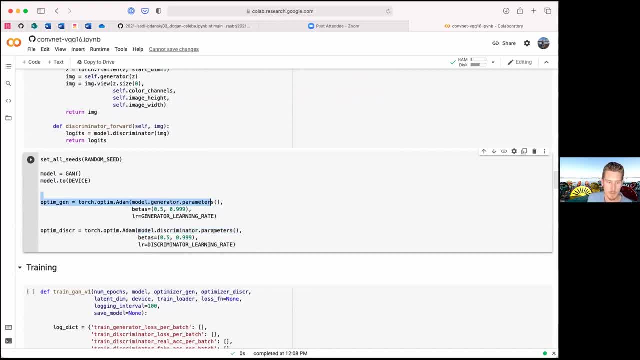 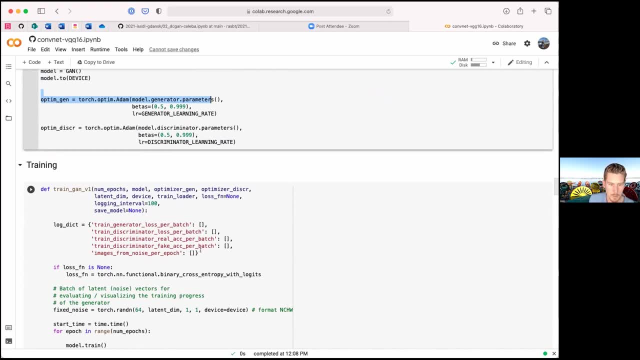 one is only updating the discriminator and this one is only updating the generator. And then here I have my training function. It has a lot of things going on, but many of those are just for logging so that we can visualize the loss later and look at the results. 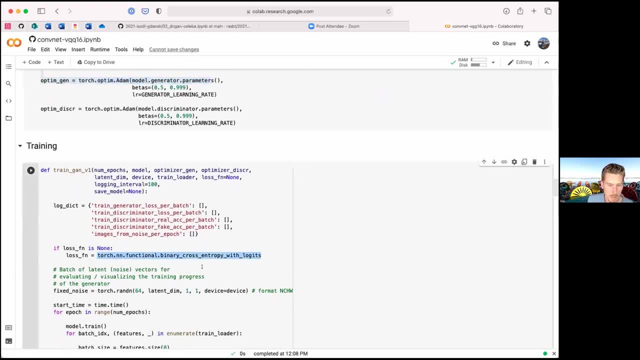 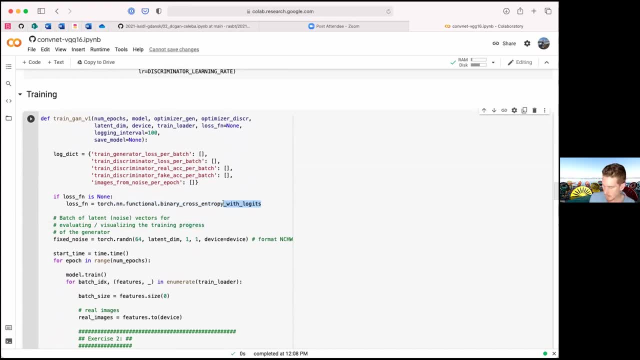 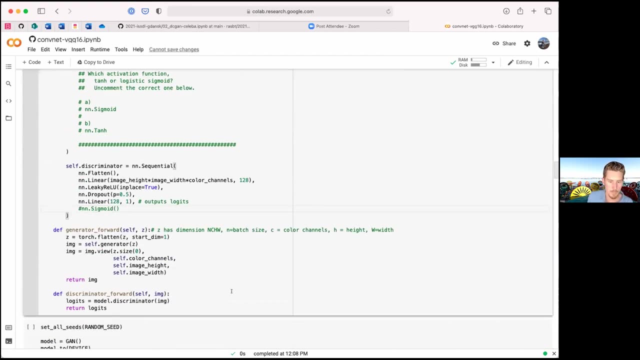 So here we are using the binary cross entropy with logits loss function, And this one expects the logits. There's also binary cross entropy, which would then work with the sigmoid here, But for numerical stability it's recommended to use this one. Here we have our fixed noise. 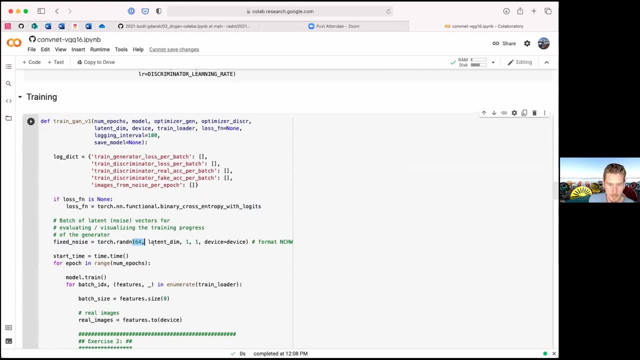 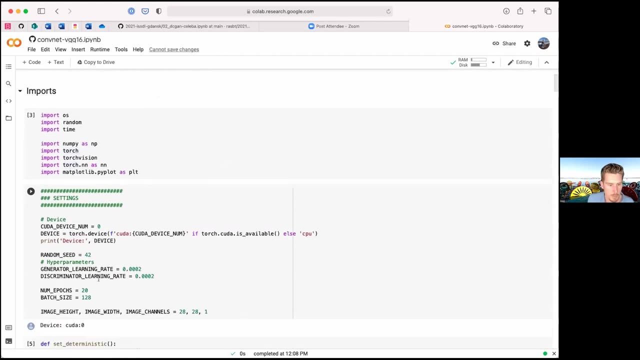 It's a 64 dimensional vector that is then reshaped into 64.. Oh, sorry, 64 is the batch size. 64 dimensional, sorry. 64 vectors of the dimension latent dim, And I think I set this to if I go to the very top. I didn't set it somewhere here. 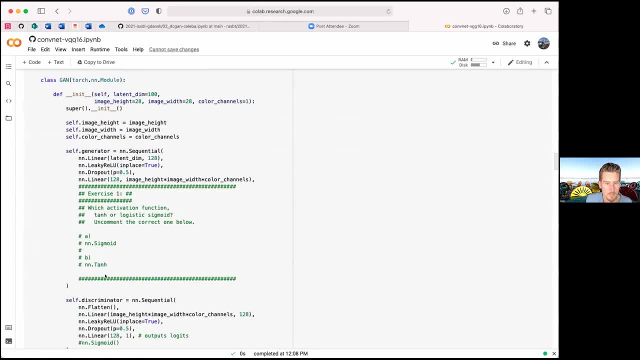 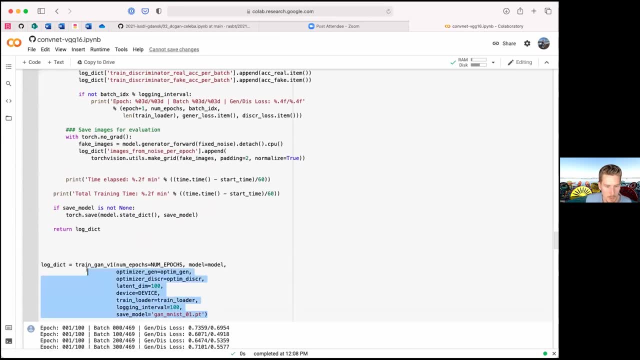 It should be. maybe I said it later. when I call the function, Scroll down. So I'm defining the function and then I'm actually calling, I'm calling the function. So yeah, I will set this to 100, but it's again a hyper parameter. It's something to experiment with to see what 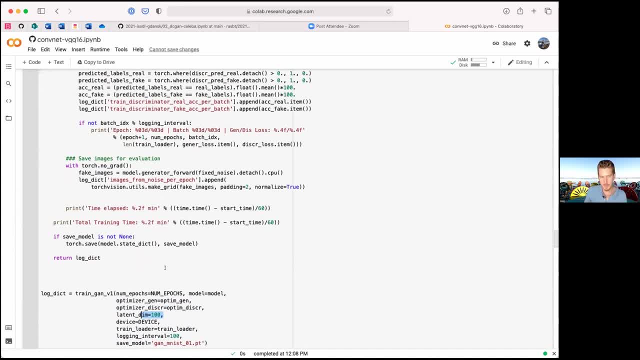 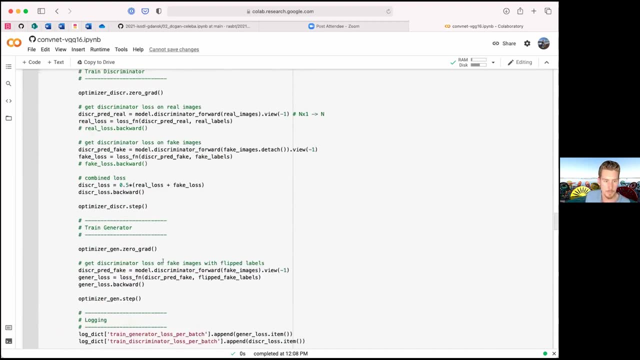 works well. Usually, the more complex the images, the more layers you need, And also some of the. sometimes you want a larger latent dimension to start from, but usually 100 is a good number, So we are also later going to use 100 for the face images. Okay, So going back to where? 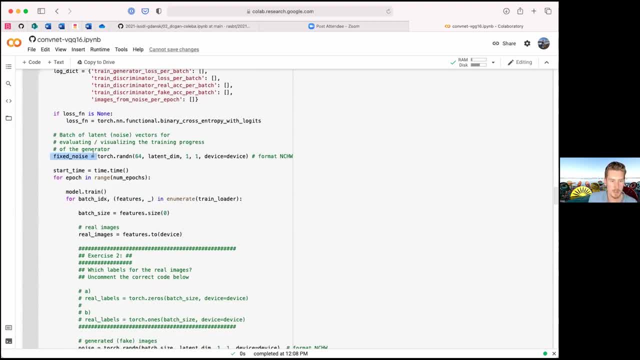 I stopped, Okay, So now this is all fixed noise and I'm using this fixed noise to evaluate the results during training, because in this training function I have a sub function that looks at the generated images for every 10 minutes In epochs, And then, using this fixed noise, we start from the same noise and it's easier. 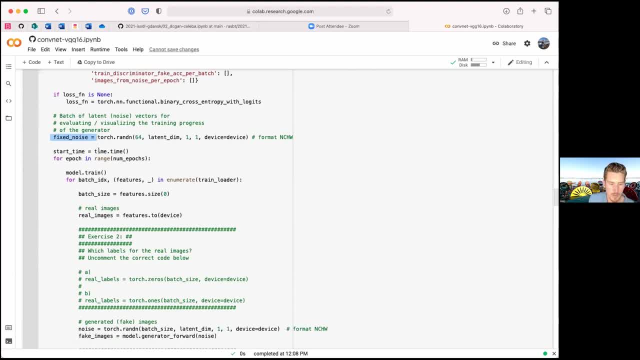 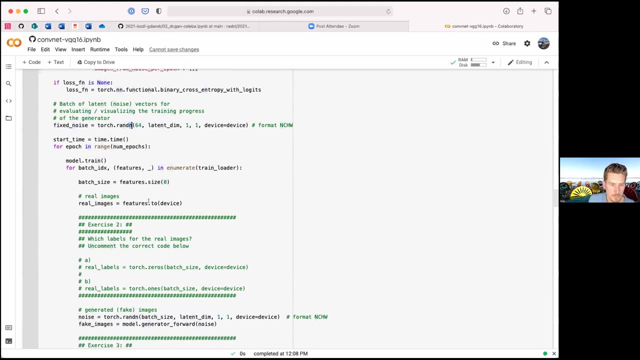 to compare how much progress the GAN makes. But then during training we actually use new noise, So it's a new noise. I should say rent N is a random normal distribution. So I think the N should stand for normal distribution. You could also consider a uniform distribution. 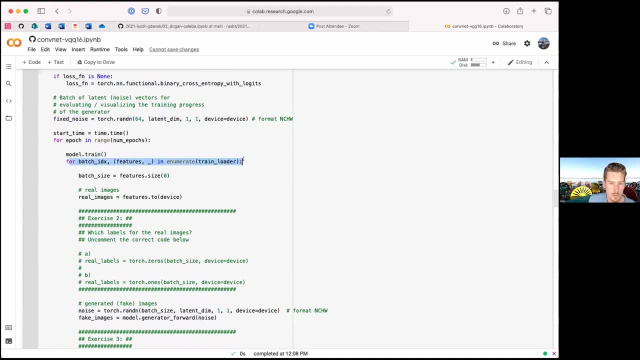 So that would be another exercise. So here this is the training loop, where we are iterating through the training data set And then we are initializing, putting the real images onto the GPU. If you train this on a CPU, then this is a kind of redundant: the two device. So the two device would just put it on the 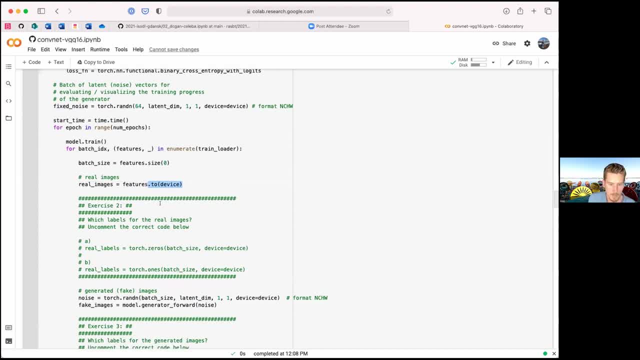 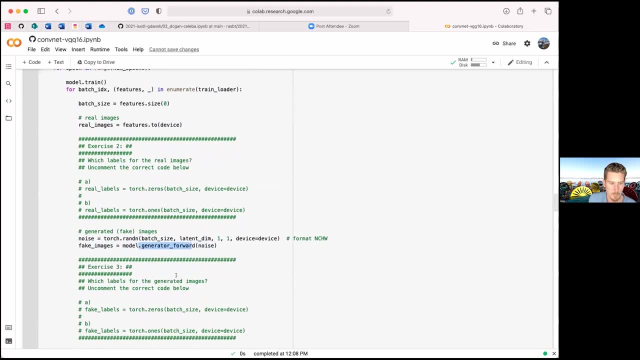 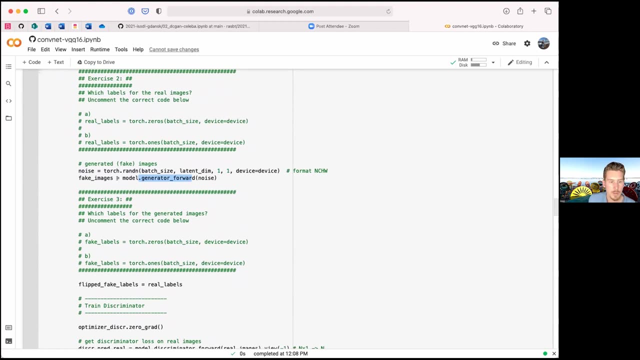 device that we chose, either the CPU or the GPU- And yeah, then we have the noise, We have the fake images which come from the generator. here And in this step we are first. what are we training? We're training the discorator first. Okay, So we get the fake images And 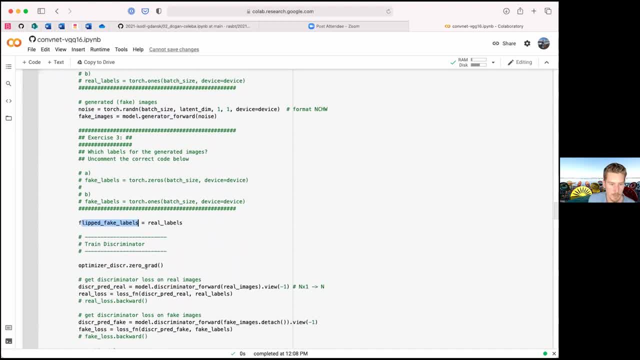 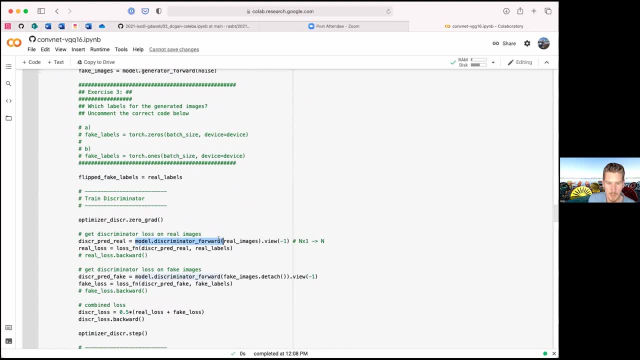 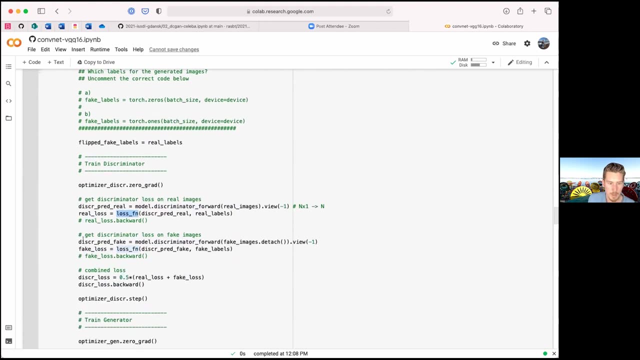 then we are training the discriminator first. So we call the forward method that we defined on the real images, compute the loss with all binary cross entropy loss, And then we do the same thing with the generated images- Here I'm using fake images, detach. And this is so that we don't use the gradient, because 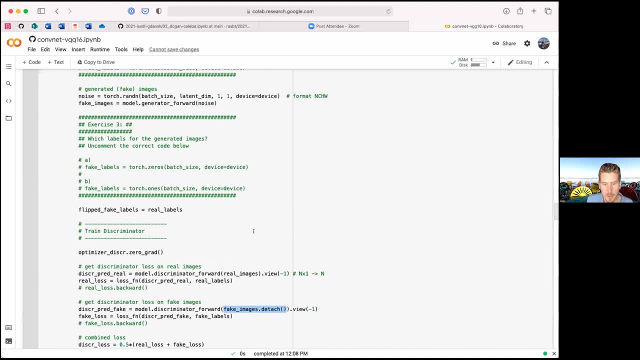 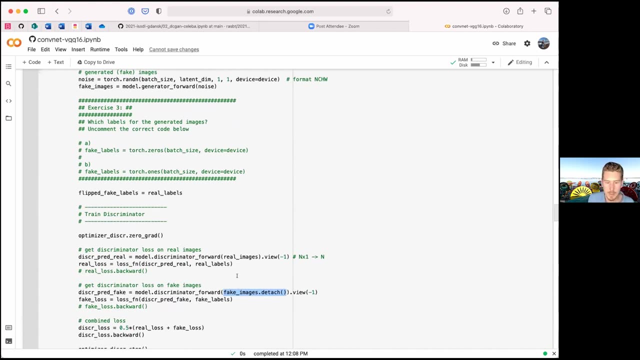 otherwise it would also up the update the generator or not update it, but compute the gradients right. So we don't need that, or we don't want that, because then the computation graph becomes unnecessarily complex. So we are only using the fake images, as is. So this will really this step temporarily. 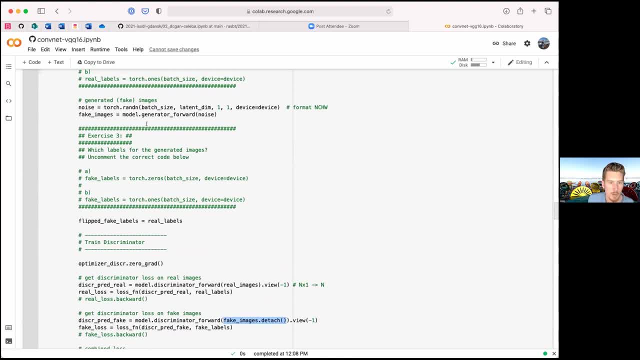 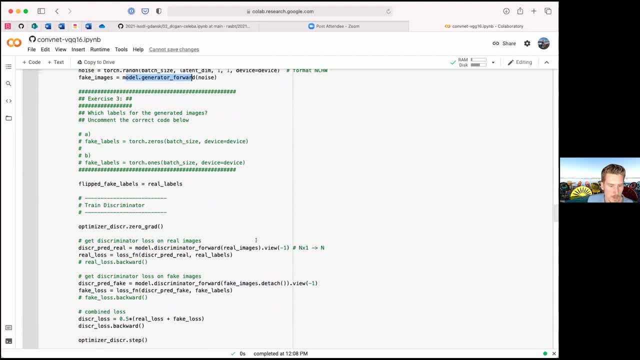 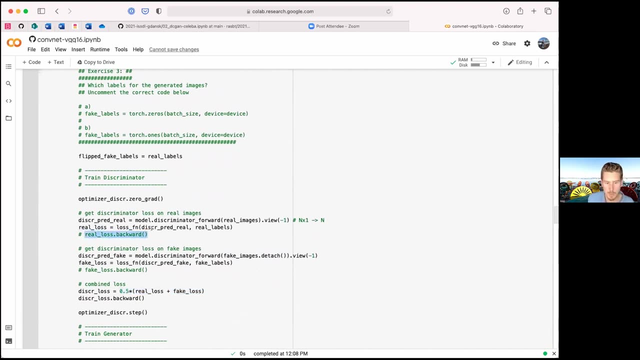 will decouple the fake images from the generator, So it's like a decoupling step, just that they are like the regular images. Yeah, and then here I just combined. I mean you can- you probably have seen that before- backward will run the computation graph backward to. 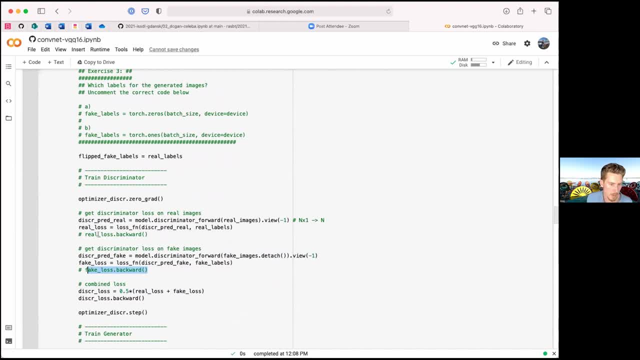 compute the gradients. We can do this in two steps separately, for the real loss, the loss on real images and the loss on fake images, or we can just put them together, because the sum rule in calculus would compute them separately anyway, and then we only have to. 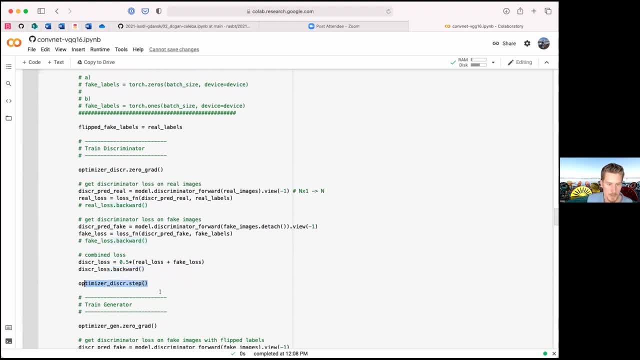 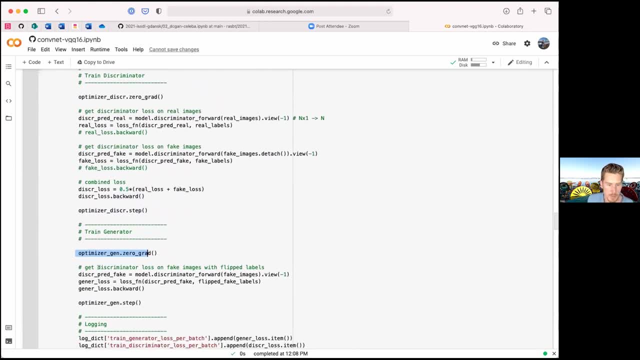 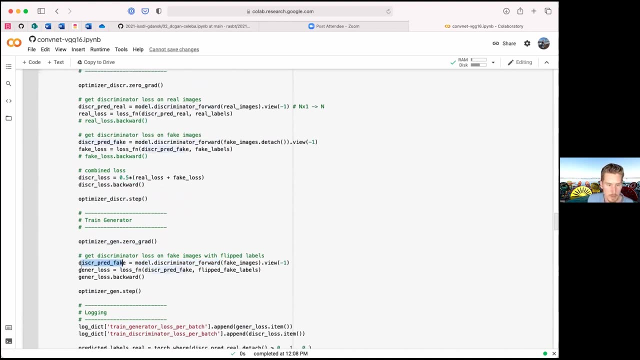 call backward once And then we update the discriminator. Next we will update the generator. So we have a very similar approach. We call the discriminator forward to predict the images here. Then we call the generator loss, compute the generator loss on the fake images and the flip fake. 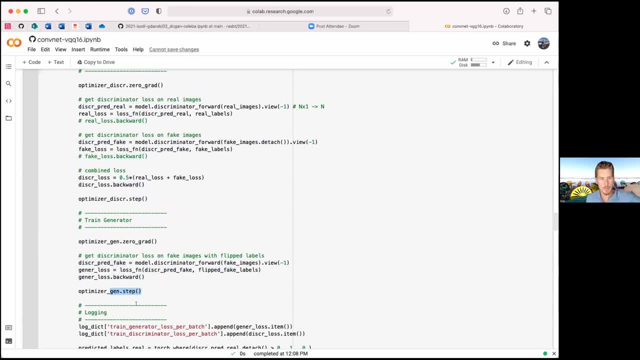 images, call backward and update. So there's a lot of stuff going on and we only have- yeah, not that much time, So in that way it might be a little bit overwhelming, but I hope the exercises are pretty straightforward, So I will give you 15 minutes for these little 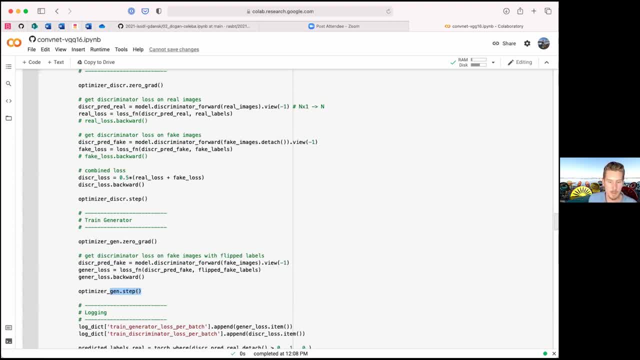 three exercises In this process. you can also maybe look a little bit at the code and let's say until, let's say, 12 minutes. So then in my time at 1230, I can in the last 15 minutes. 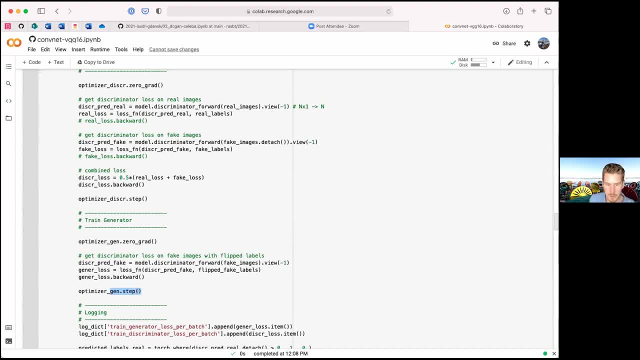 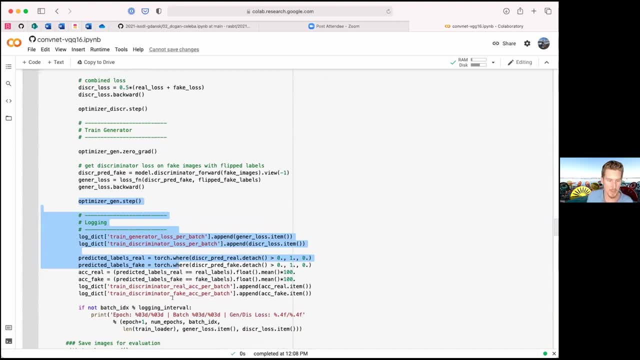 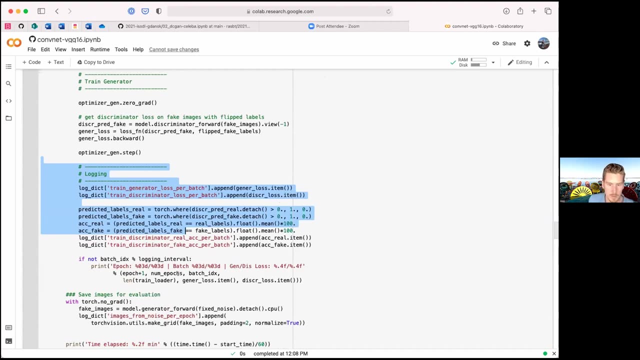 talk a little bit about the face images and also the GAN resources. So the remaining code, before I let you work on it, the remaining code here is only like for logging purposes. it's computing or saving certain things and computing the loss so that we can plot this here. So I'm just, this is only for visualization, so that I can see. 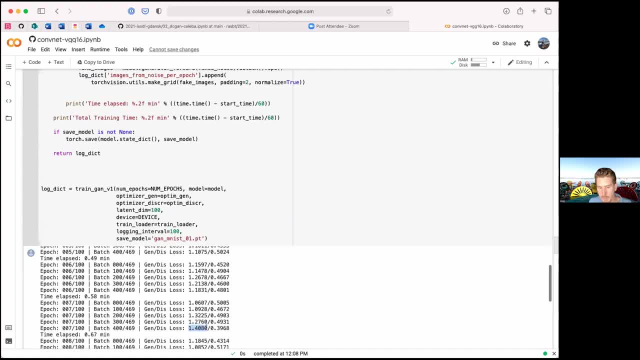 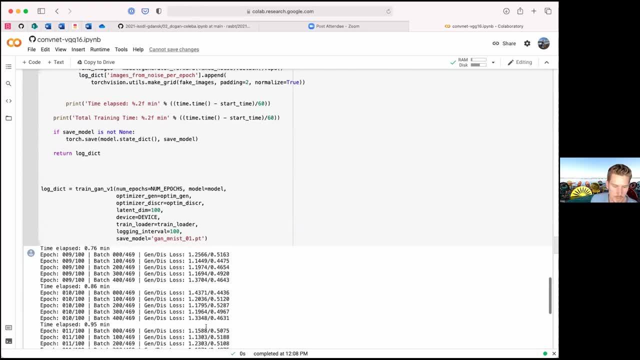 during training what's going on here, because sometimes these numbers become very large or very, very small, or they become NAN. So there's some error then, and it just helps me to bring training to see what's going on, because it might take a while. You probably don't need 100 epochs by the 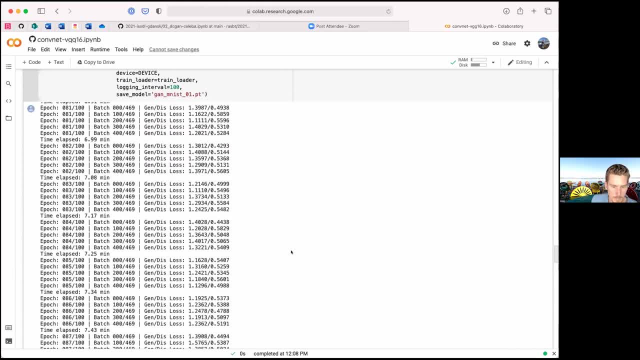 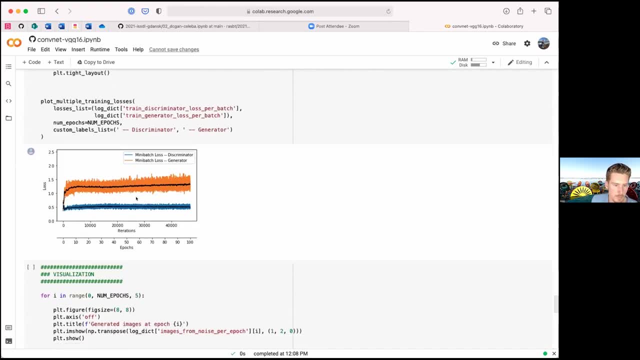 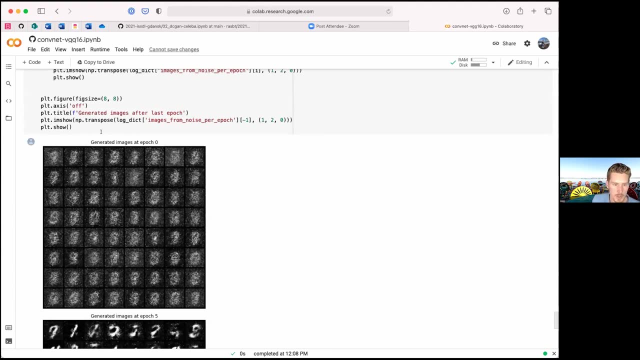 way, it's a little bit excessive. Okay, I'll go down. and this is then a plotting function. So this is how the losses would look like if you solve the exercises correctly. And then here are the generated images. So it starts really really very random. So this is at epoch zero, so very random outputs, And you can see at: 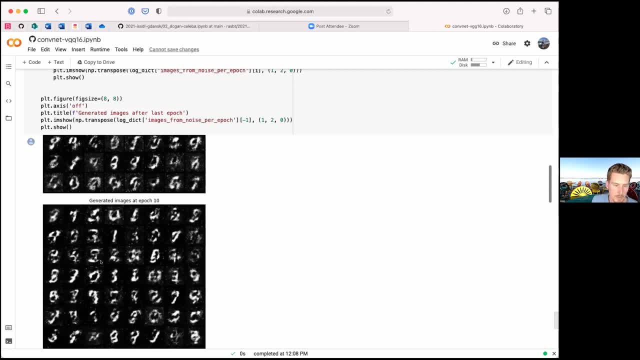 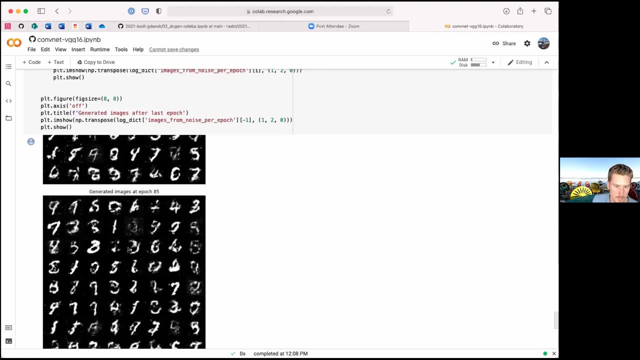 epoch five, it already improved a little bit. Then at epoch 10, it looks a little bit better, even better, And after, let's say, after the last epoch, they kind of- I mean not all of them, but some of them- look like: 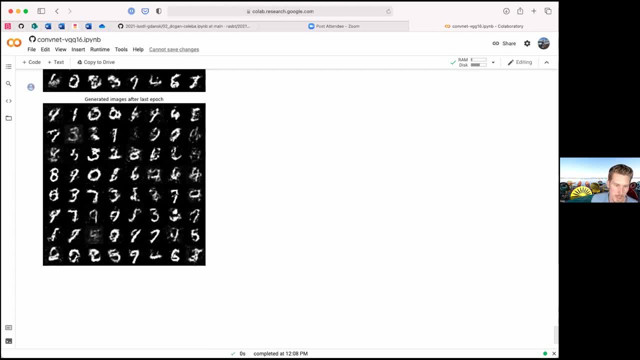 real handwritten digits. So here kind of like a seven, this is like a nine, a zero, an eight. Of course there's a lot of outputs that don't look well. If you look at the original GAN paper, the results actually look better there. but the original author also mentioned in a talk once: 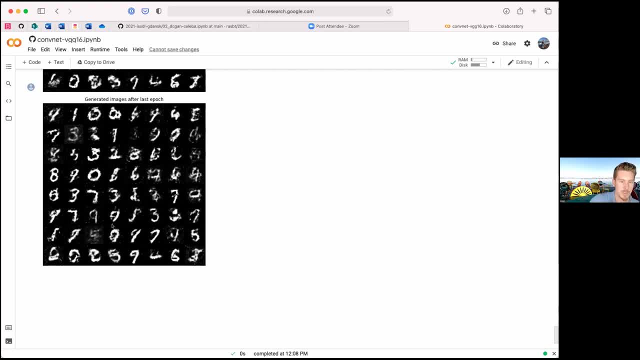 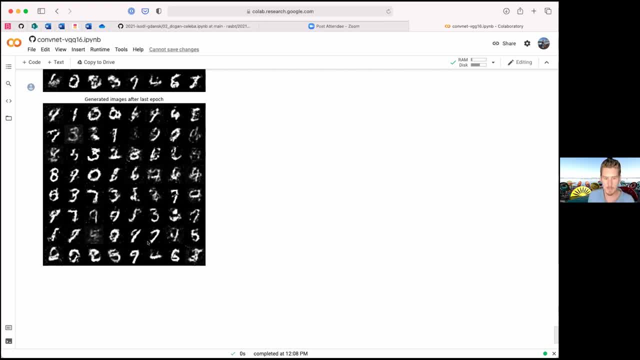 But of course we could get way better results with more sophisticated GAN methods. But again, this is like the simple GAN with the fully connected layers, just to for introduction, to become familiar with the loss function. All right, Then I would say I will give. 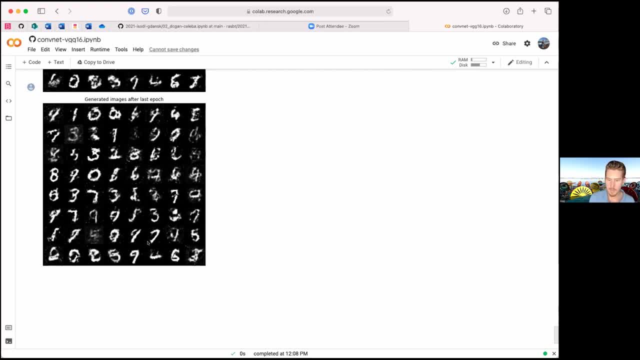 you 12 minutes to work on this and then I will be back and talk more about the DC GAN. All right, Thank you so much for joining us today. We'll see you next time, Thank you, Thank you, Thank you. 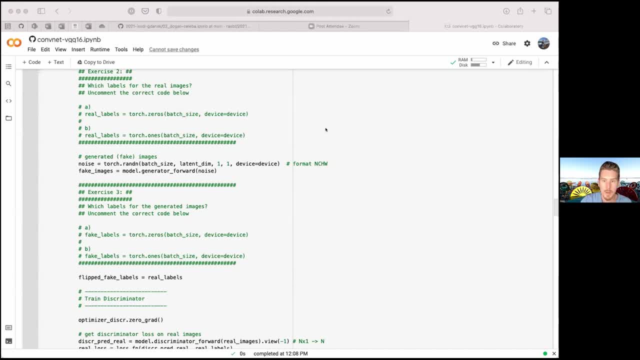 regarding to overfitting, There was another question about why only real images are used for training the discriminator, So why not? when I read the question correctly, it's about asking why not mixing the real and the fake images, And I will get to that in a moment. So 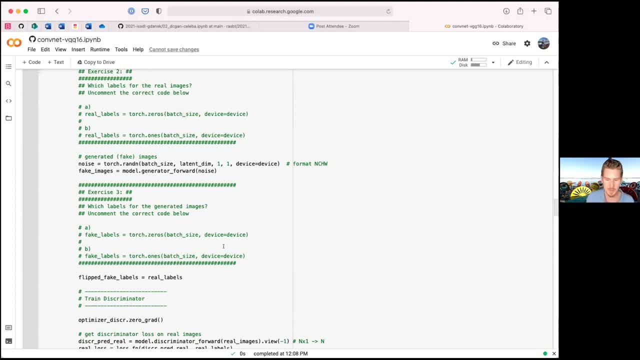 that is a very good point. It has something to do with batch normalization. I will talk a little bit about that, Yeah, So in the remaining- I think- 15 minutes, let me just tell you the solutions, of course, and then talk a little bit about some tips and tricks. 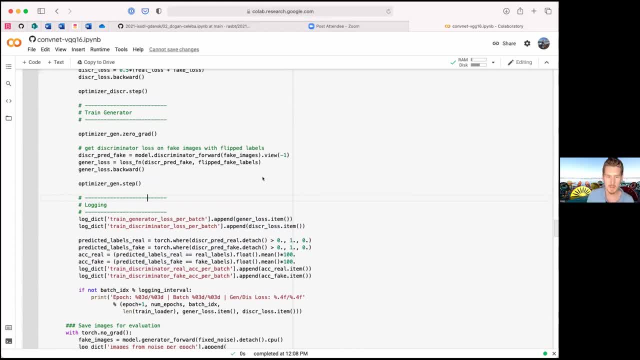 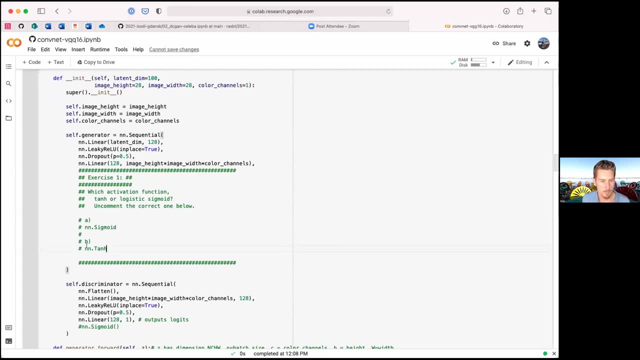 the face images part, which will be very quick, and then maybe some further resources for you to learn more about the recent developments in the GAN field. Okay, So scrolling up here, exercise one. So here the solution should be 10H, And this is because this is why I spent so much. 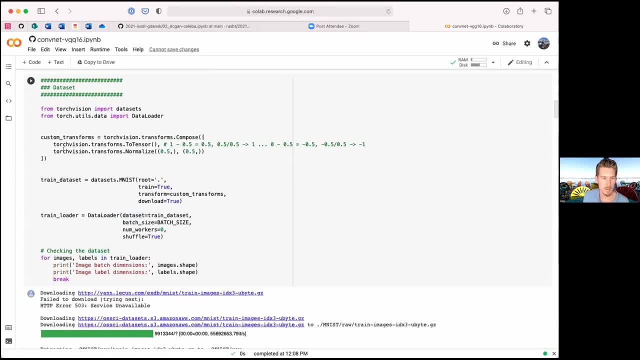 time on explaining the data loading. This is because we have this line of code in here which normalizes the images. Okay, So this is why I spent so much time on explaining the data loading. This is because we have this line of code in here which normalizes the images. 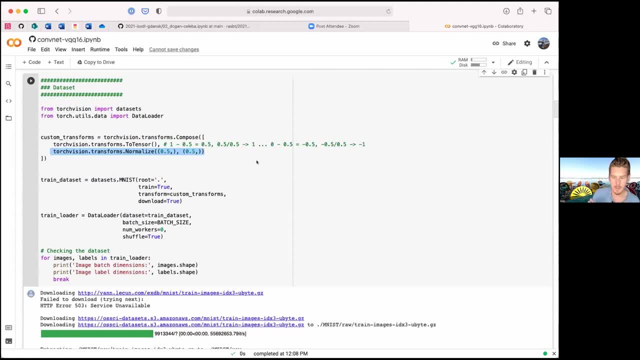 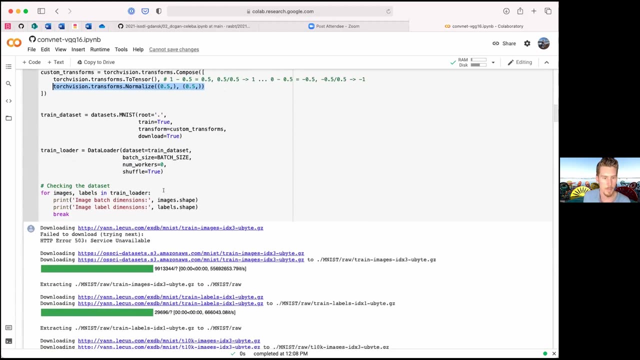 such that the pixels are between minus one and one, and with a 10H function we match this output range. If I remove this part, then we could use the sigmoid function in the generator, But with this line of code here, the highlighted one, we want to use the 10H function And, yeah, the other. 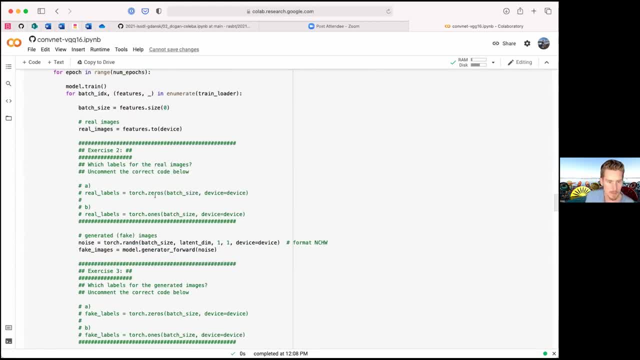 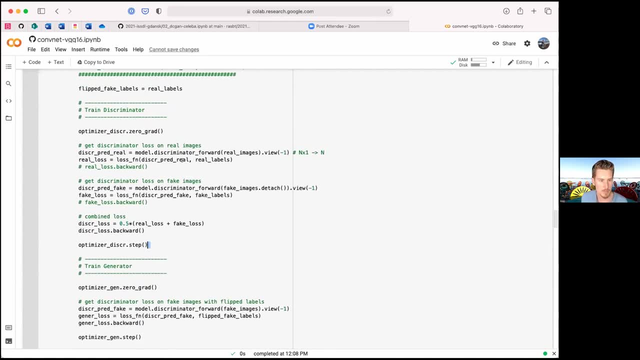 exercises were, I would say, rather simple. You could maybe read them up from the slides. even So, for real images, we use- oops. I did a jump. For the real images, we would use the ones here, So we would, oops. 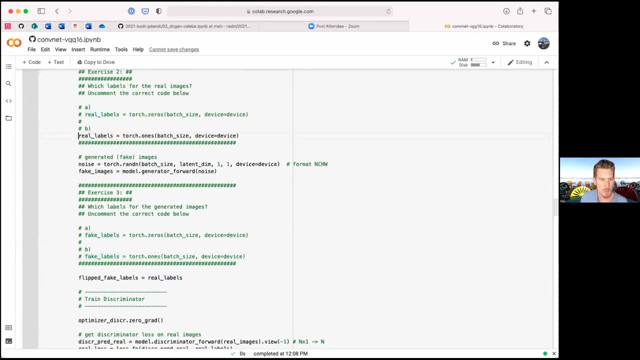 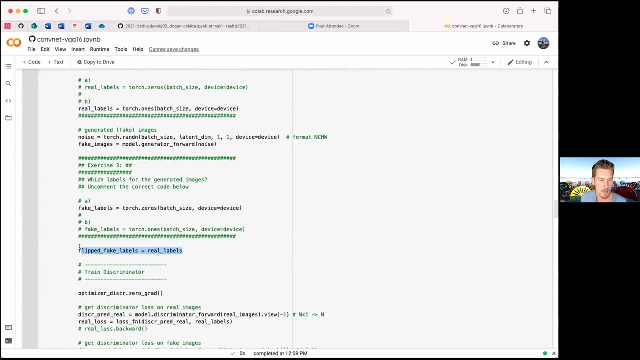 why is it fake? Okay, it jumped here for some reason. For real images, we would use the ones, And for the fake images we would use the zeros. And then for the flipped ones, the flipped fake images would also be the ones then, By the way, I uploaded the slides to GitHub. 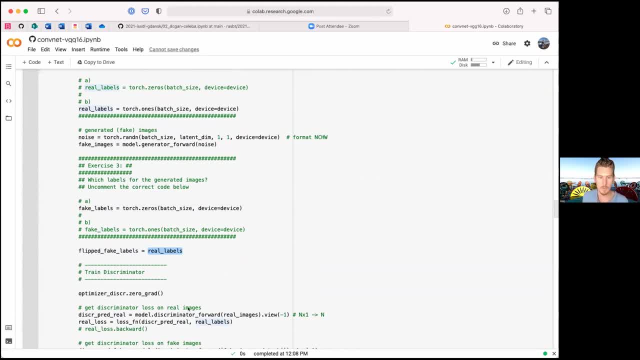 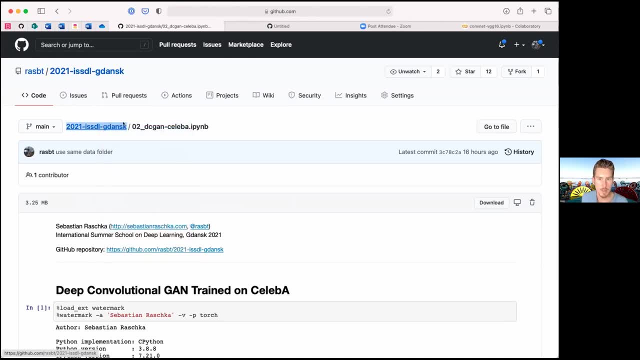 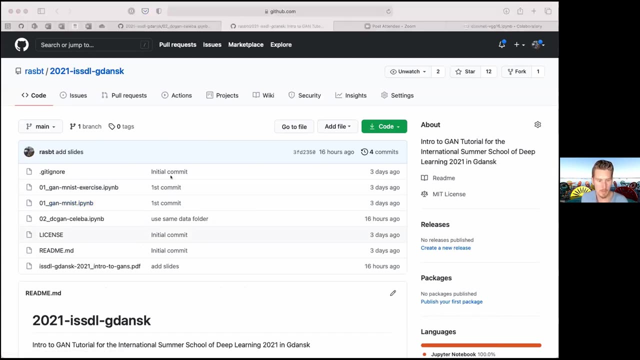 I shared a code, the link in Slack, if you want to have access to this later on, And there's also a version. if I go here, there should also be a version in here that has the solution here. this one, Okay. so moving on with the lecture then. So, oh, I skipped a little bit forward here, So 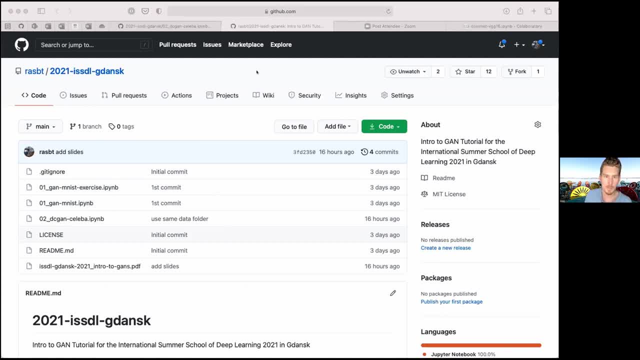 we stopped at this point where we were playing a little bit with the GAN, And here I just wanted to share a few tips and tricks with you to make GANs work in practice. So there is this nice GitHubjsoncom. 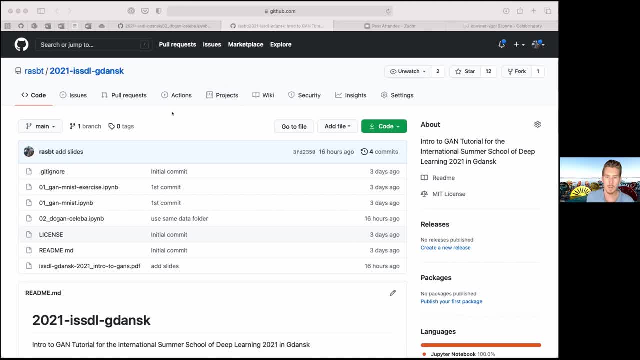 repository by Sumit Chintala, who was involved in developing the first deep convolutional GAN and also later the Wasserstein GAN. So he compiled a list of different tips and tricks. I think there are 17 or 18 tips and tricks. He says that they are maybe not super relevant in 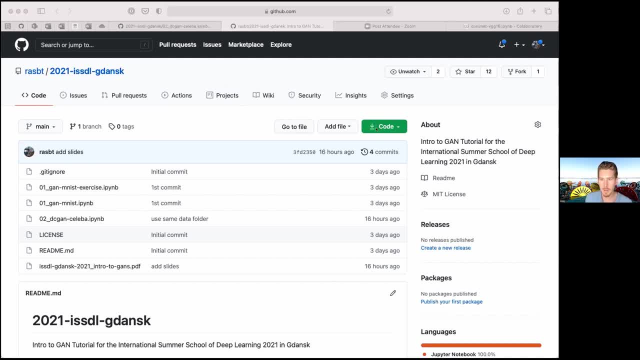 2020 anymore, or he is not sure how relevant they are. I think most of them are super relevant when it comes to the regular GAN training, but then there are some advanced GAN methods that use different tricks. So these are some of the tips and tricks that Sumit Chintala gave us. So 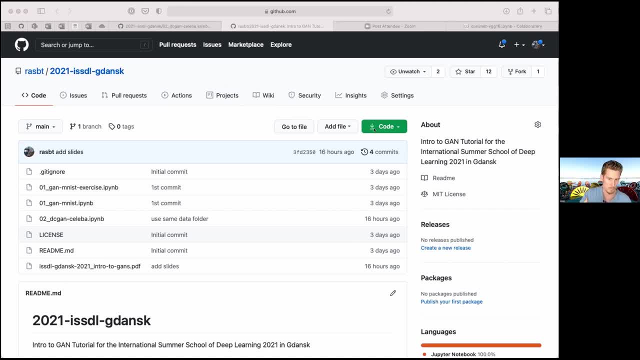 these tricks definitely apply still to all the, I would say, regular GANs. For some of the later GANs, there are additional tricks and tips that are not in this list, but you can find them in the research papers. So just going through some of those, not all of those, because we don't have 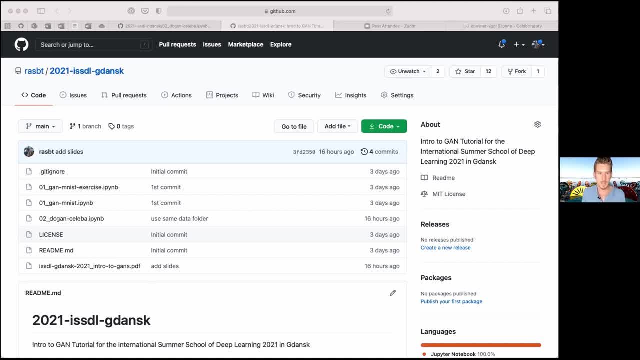 so much time, but there's also the link if you want to read through this. So one tip would be normalizing the inputs. So normalize the images between minus one and one and then use 10H as the last layer of the generator output. And yeah, this is a little bit more complicated, but yeah. 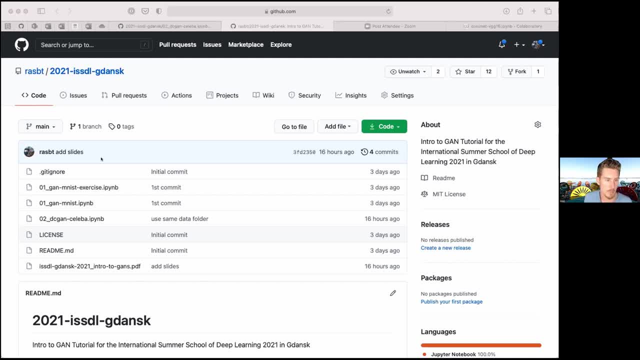 this is what we did. So we did that in the code. So we used 10H in the generator. This was one of the exercises, And here we had this normalization between minus one and one. Another trick would be the loss function. So I glanced over this detail. So in the original paper, 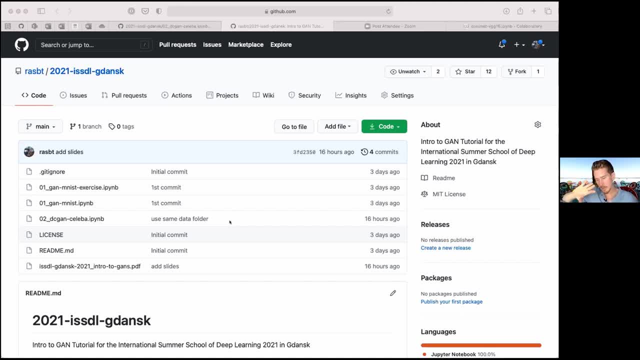 they propose the GAN objective and then they flip around the labels because otherwise the gradients would be too shallow. We really didn't discuss that in too much detail because of time constraints, But just the short version here would be: we are adhering to this. 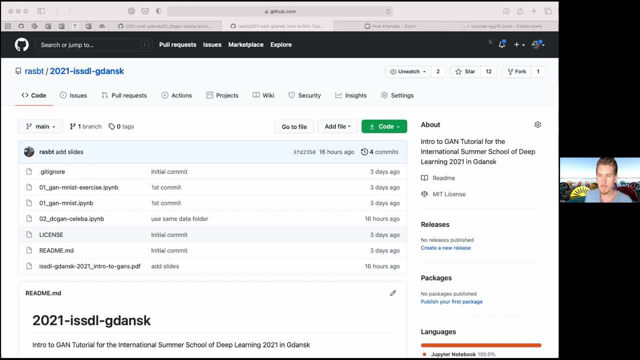 tip as well. So instead of having max lock d- we have- you can turn this into a minus min lock d. it's the same thing. And we also flip the labels when training the generator and discriminator. So this is also something we have done in code, So this is also implemented in our code examples. 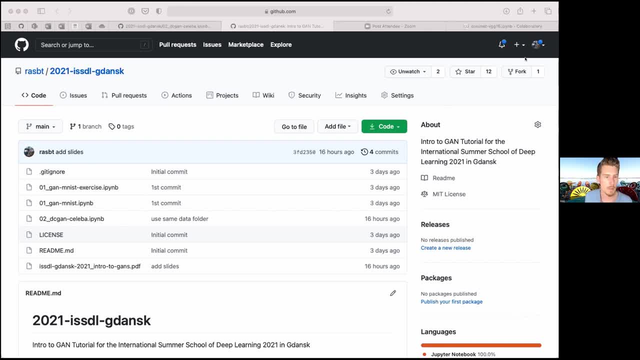 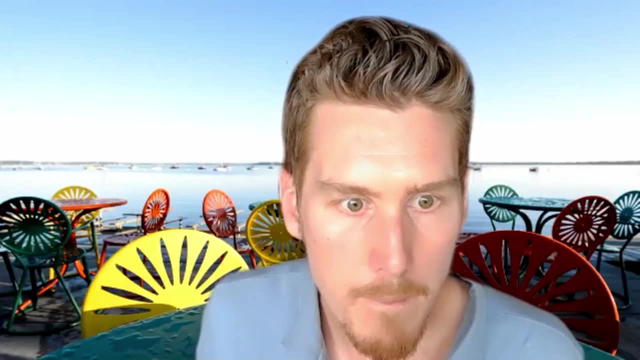 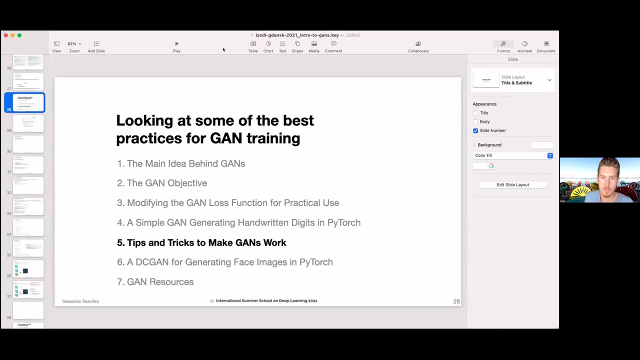 So we use: yeah, min minus lock d. basically we do not see the presentation anymore. oh sorry, i think that's because i'm still sharing the browser. thanks for noticing that. i will give that, okay, okay, okay, um, let me share the keynotes. okay, i think. no, it should work right. yes, it's okay. 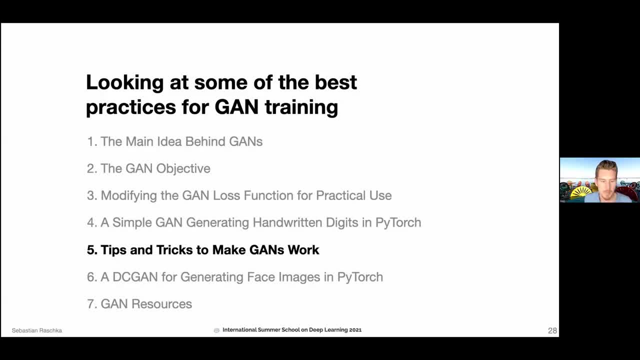 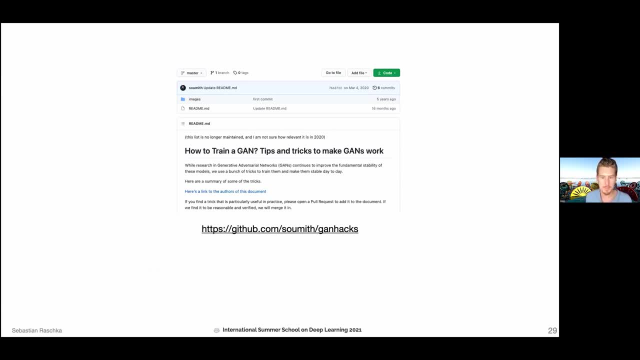 oh, sorry about that. i shared the wrong screen, okay. um, yeah, here's the link to what i mentioned before: the tips and tricks, uh, for training gans and um, yeah, what i just talked about is tip one, normalizing the inputs between minus one and one range. so this is something we did in code. 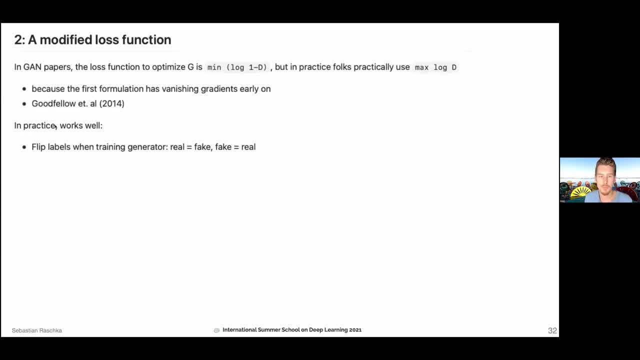 so, and then the other tip i mentioned was, uh, flipping the labels, which is also what we've done in code. so i glanced over the detail with the gradient. but i have on youtube- i can also share you with that, that with you later- a video on explaining the gradient issue. 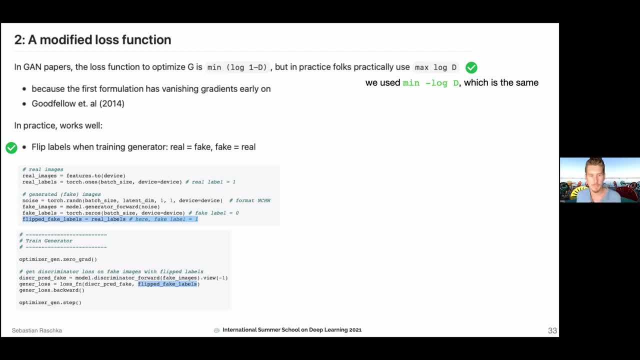 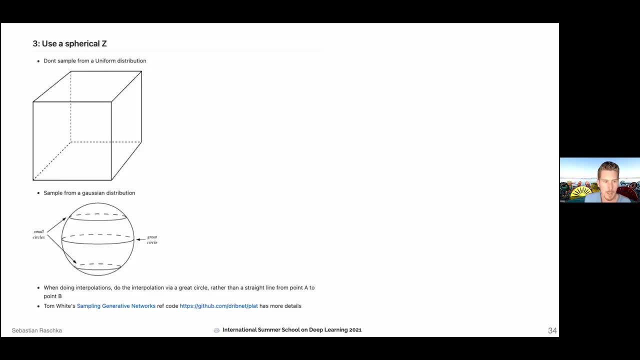 it's like a 20 minute video or something, so i unfortunately don't have time to go over this detail, but just wanted to mention um there's a reason why we flipped these labels. um, using another tip would be using a spherical z instead of a uniform distribution, so it's also in practice. 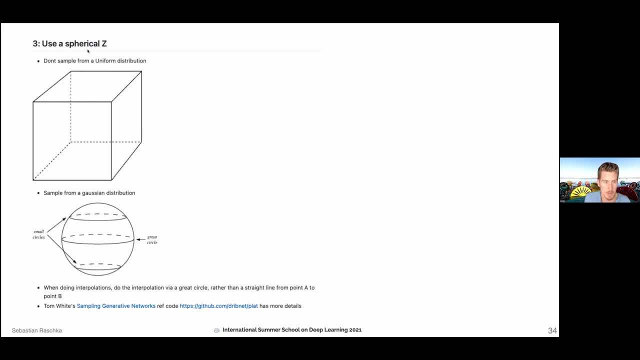 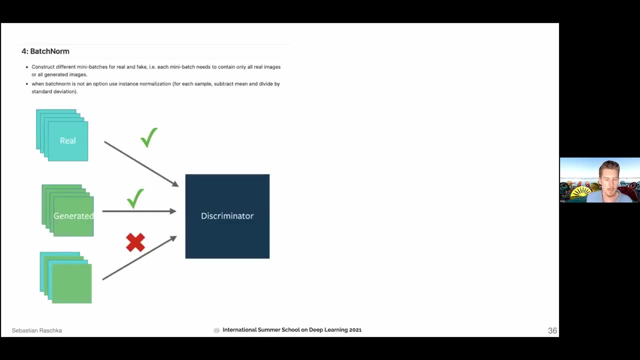 better to use a gaussian or random normal distribution, like with it, instead of the uniform distribution, and also this is a tip that we adhered in our code example. so with this, rent n sampling the noise from a normal distribution instead of a uniform one, um, and this goes back. 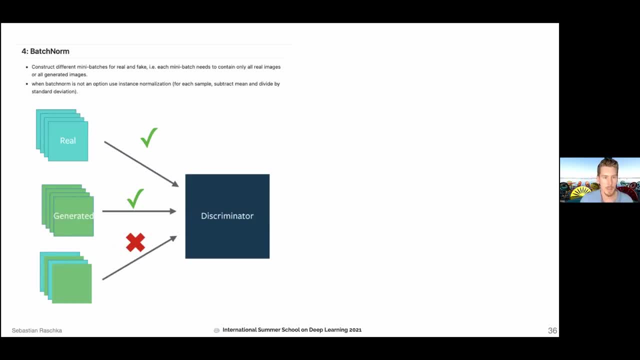 to the question that someone asked um in the chat. so why don't we mix um the real and generated images in the batch? why do we use them separately? does that have something to do with when we use batch norm? it performs better if we keep them separate, as real images and generated images. 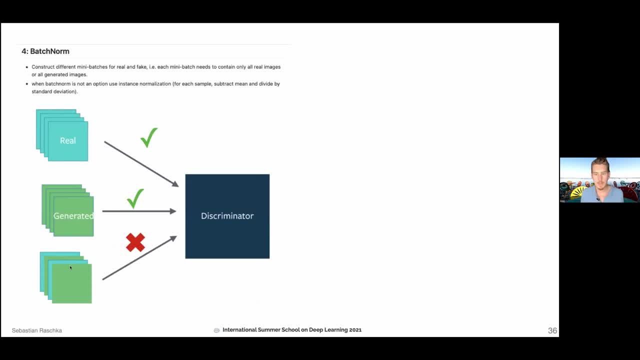 instead of mixing them. in our code example, we didn't use batch norm. we didn't use batch norm, um, but i used batch norm in the dc again, so we can take a brief look at that one, um. yeah, so there are more tips, but yeah, due to time reasons, i was thinking we would probably 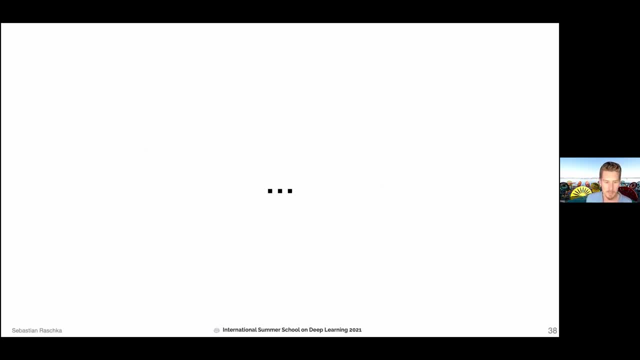 not have enough time for that, and i think this is about true. we have like 12 minutes left, i don't know. actually eight minutes, sorry. so, um, i encourage you to go to this list here and maybe, on your own time, walk through this list and see whether we implemented these. things in this way. so i think it's a good idea to do that, and i think it's a good idea to do it. okay, so i guess i think it's a good idea to do that, and i think it's a good idea to do it. 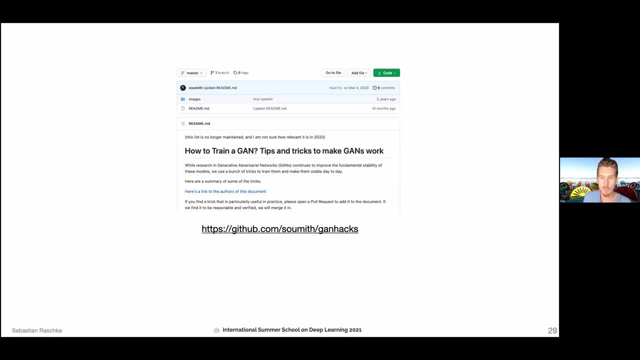 things in code, And you can also try to remove these tips and tricks, in a way like maybe not normalizing between minus one and one, and see what happens, whether it makes the results better or worse. That might be an interesting exercise. Yeah, Okay, So then? 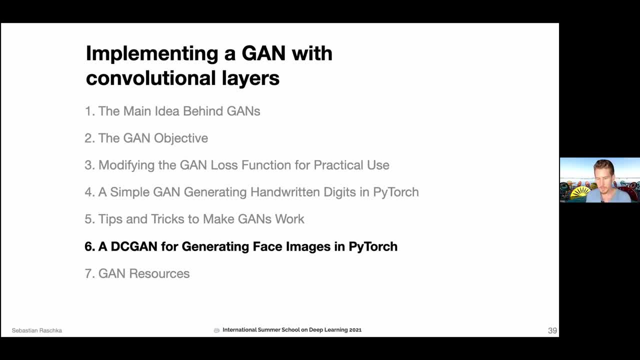 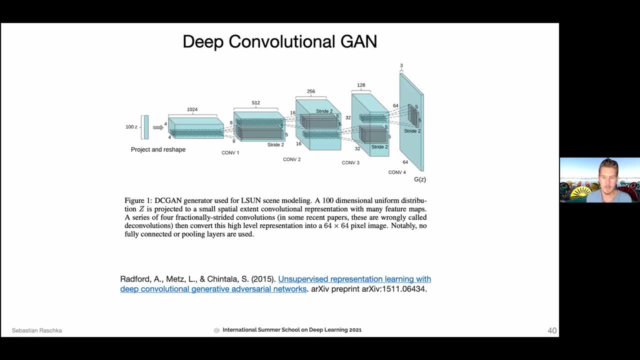 the DC again for generating the face images in PyTorch. So the real, only novelty here is that we are now replacing the fully connected layers with these convolutional layers. And yeah, it's a convolutional network. They say notably no fully connected or pooling. 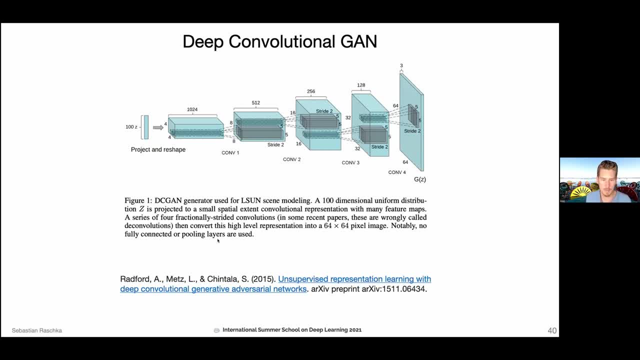 mass, just convolutional layers. And, yeah, implemented this in code, So this goes back to paper in 2015.. It's pretty old. I mean this particular architecture is pretty old, but nowadays, if you look at all the new against, they are all using convolutional layers. If 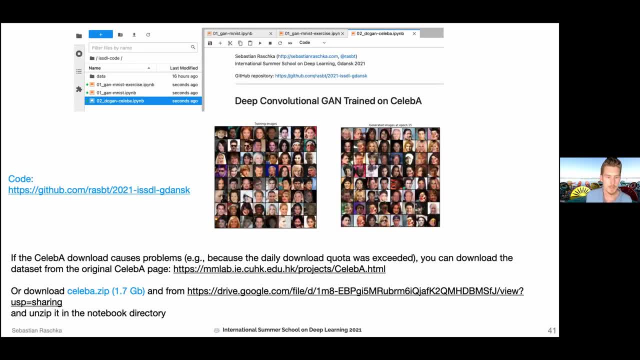 they are generating images. Okay So I have the code example, not on Google call-up, but you could upload it to Google call-up if you wanted to. Okay So, I have the code example, not on Google call-up, but you could upload it to Google call-up if you wanted to. 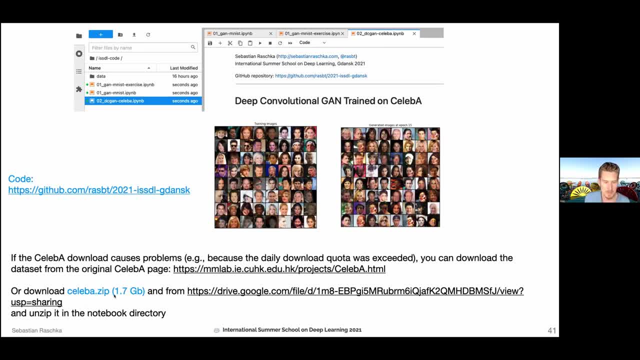 Okay, So I have the code example, not on Google call-up, but you could upload it to Google call-up if you wanted to. The problem with that is it's a large data set. It's the Syllab. A data set is 1.7 gigabytes. 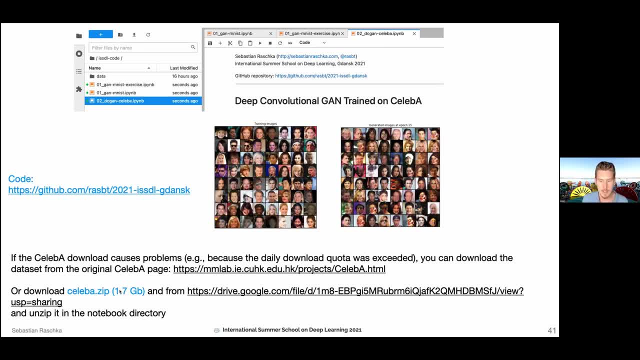 So it's something I thought we don't have time to run in this lecture, but I have the results in the notebook and on your own time, if you're interested, you can run the notebook. There is a function in Torch Vision to download the Syllab A data set similarly to the MNIST. 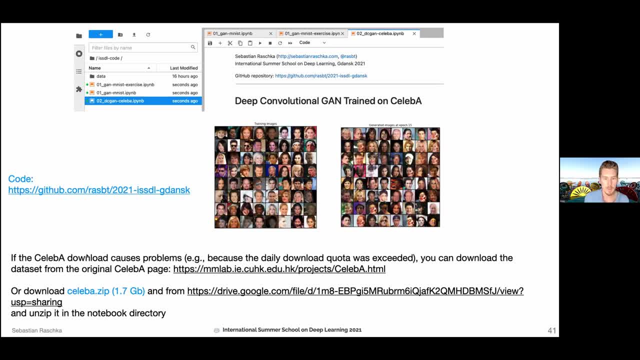 data set that we've seen before, But unfortunately every time I try that it runs out of or it complains because I think they have a quota for downloading. I think it's hosted on Google drive and then too many people download it. they exceed the quota. So you can find the. 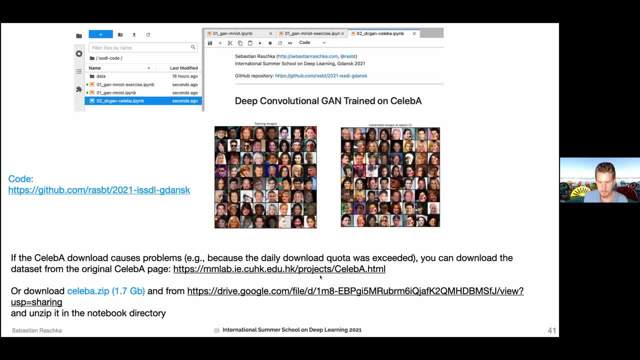 original Syllab, A data set on the original website here, where they have different download links, I think, to Dropbox, Baidu and Google drive, And I also prepared a file which has exactly the files that you need- the zip file here- and I uploaded to my Google drive. So 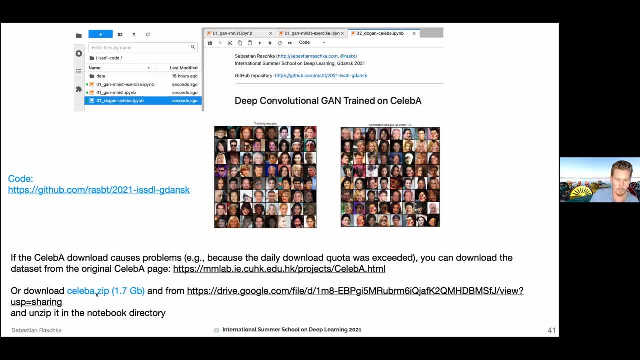 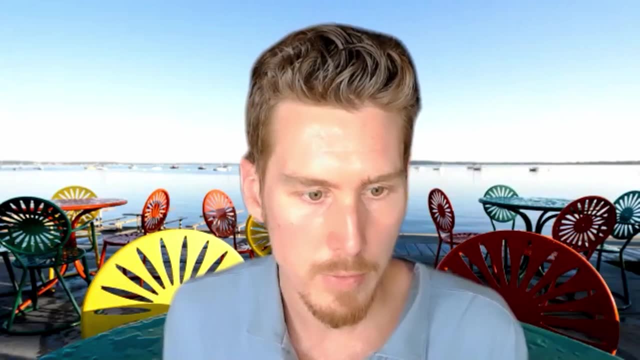 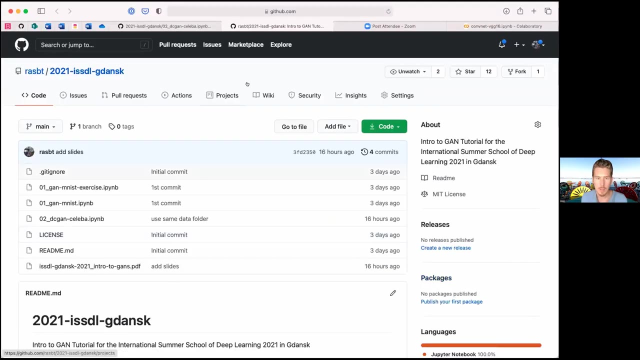 you can technically just download the Syllab Azip from this link and put it into the same directory as your notebook is. Then it should work. Okay, Let me briefly go to the notebook. share the different screen now, and then I will show you briefly the deep convolutional GAN. All right, So it will. 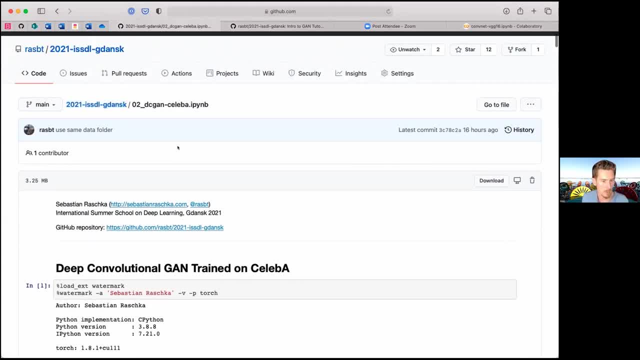 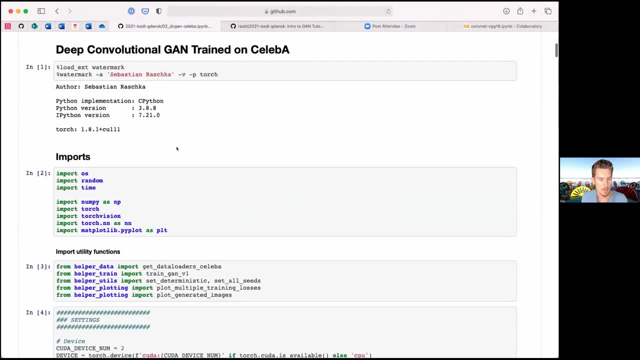 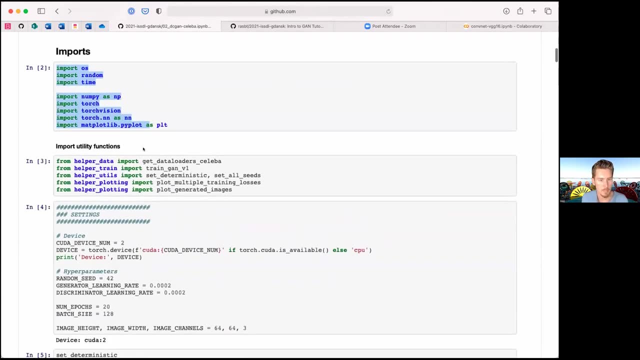 be so. this is in the GitHub repository if you want to download it and play around with that later. And what's nice about it is it's pretty straightforward, because what's cool is that, Yeah, Yeah, It's essentially all the same code, So it's: everything is the same, except now we have 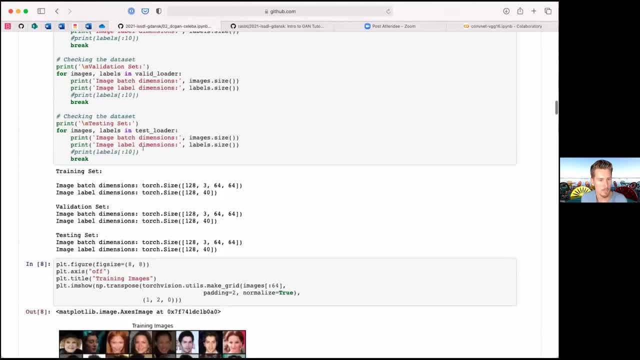 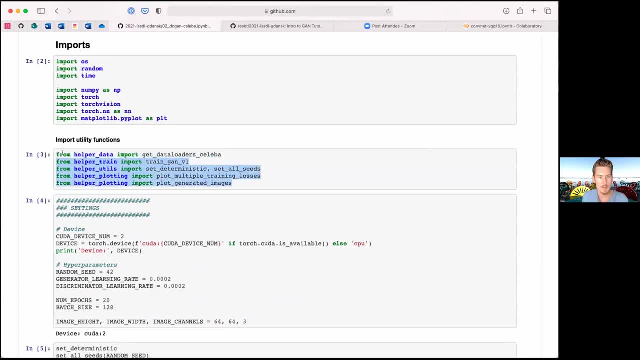 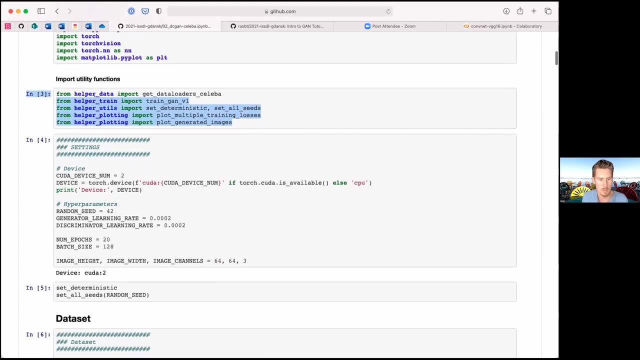 this are we here? We have the convolution networks, So let me go through this, maybe slowly. Okay, So this part. the imports are identical. This is just. you can ignore this. I had helper files before. This is probably redundant. You should ignore this or delete. 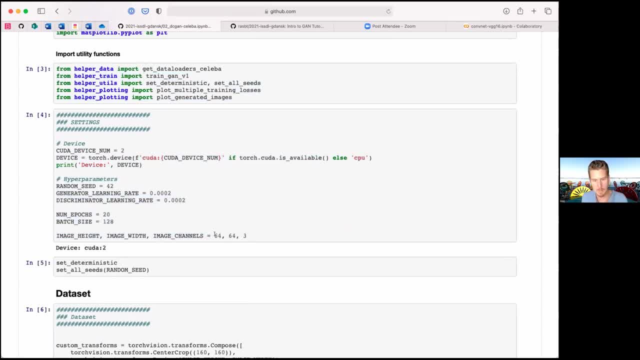 this. Here are the settings. We have 8 times 8 times 1, 28 times 28 times 1 images. We have 64 times 64 times 3, 3 color channels. We have our data loader. I implemented the function for loading this Here. we have again: 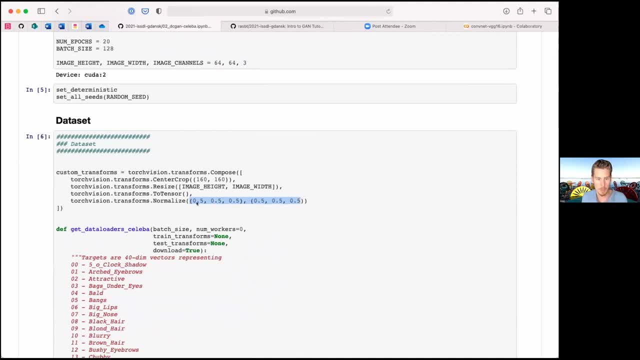 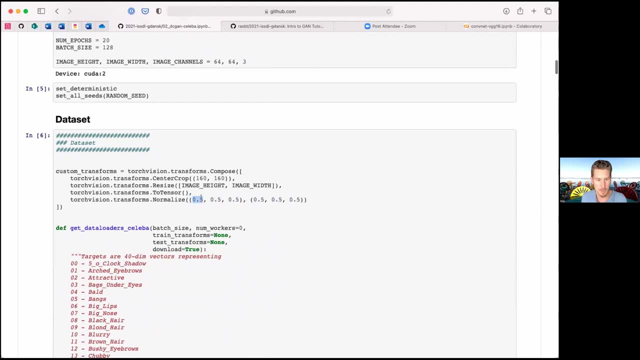 our normalization for normalizing the pixels between 0 minus 1 and 1.. Here we have three values instead of 1 because we have three color channels, So each value corresponds to one color channel. Before we only had one gray scale channel. 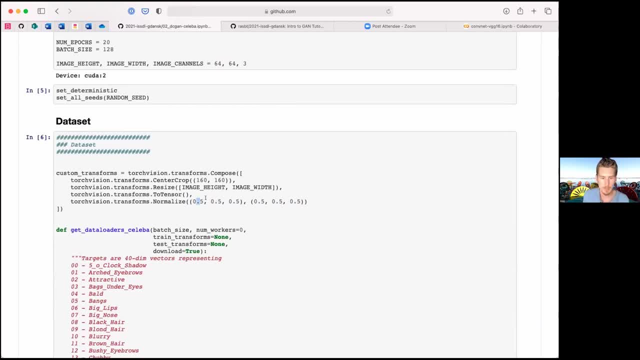 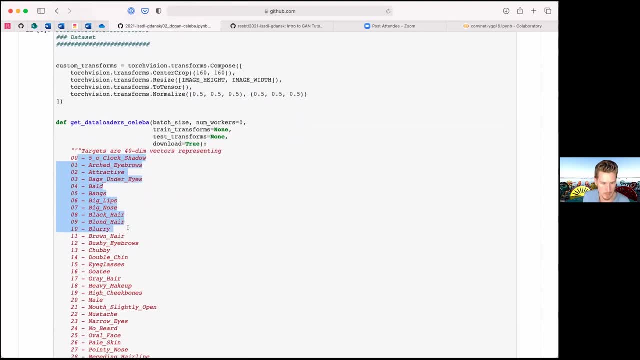 Which is why we only had a 0.5 here. Now, this is for the red channel, the green channel and the blue channel, And then the same for the standard deviations. If you're interested, this data set has a lot of class labels that you can use for different purposes. There's 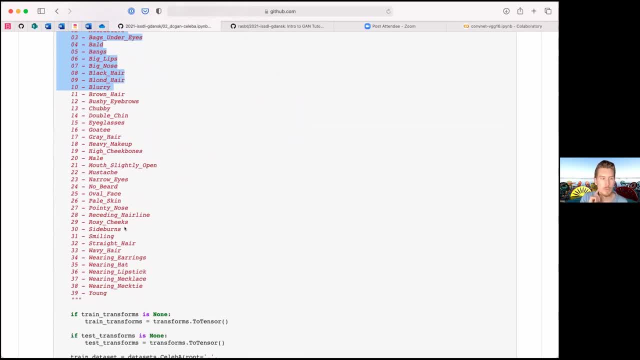 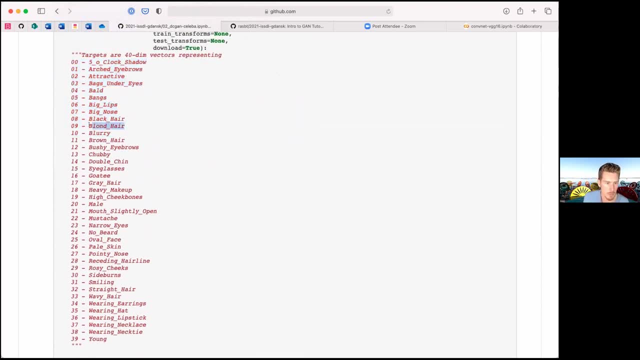 also something called a conditional GAN, which you can use to generate, let's say, images only from one class. So, for example, you can maybe train a GAN to only generate someone with a big nose, or blonde hair or eyeglasses, And then you can also generate a GAN with 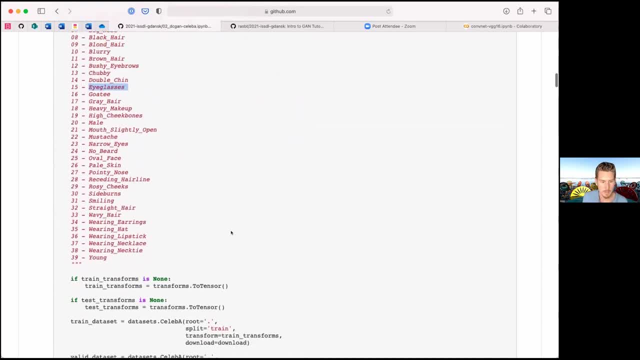 a lot of class labels that you can use for different purposes, So this is something called a conditional GAN, which you can use to generate, let's say, images only from one class. For example, you can get yourself glasses and things like that. 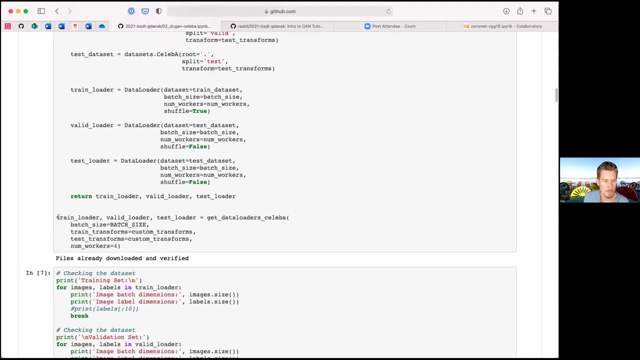 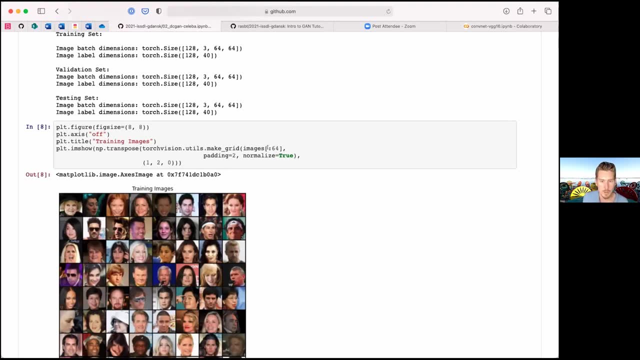 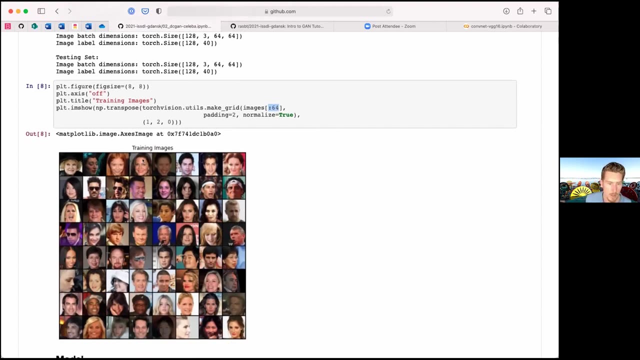 Yeah, yeah, So then we have the data loaders only using the training loader, But most of the code is really identical here. This is how the images look like. So just 64 images from the first mini batch, and Celep A stands for celebrity, So they are all celebrities. 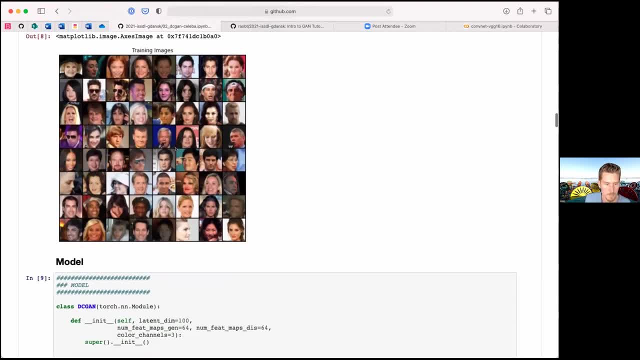 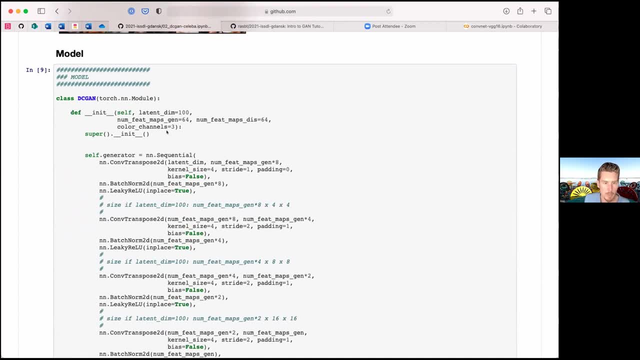 someone downloaded from Google Google image search, And this is really the main part that is different: The data set from the first batch, which is essentially how the images are rolled out from the previous code example. This is now our deep convolutional GAN. 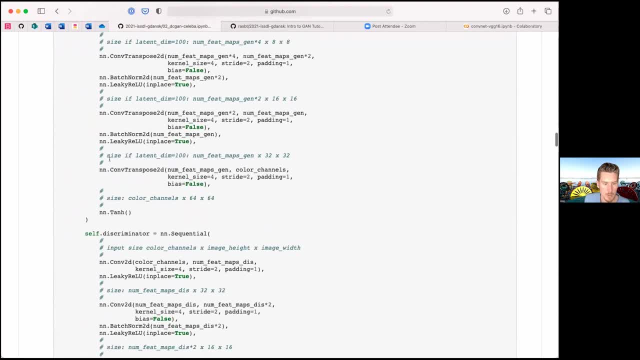 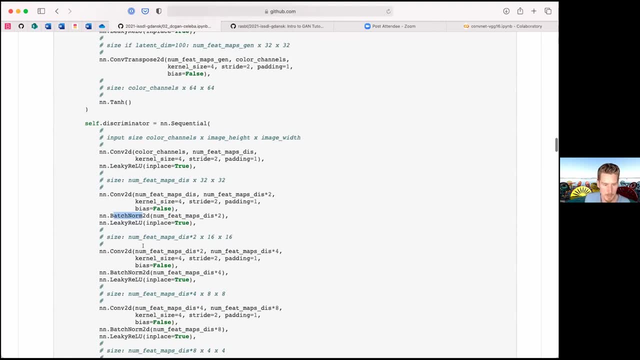 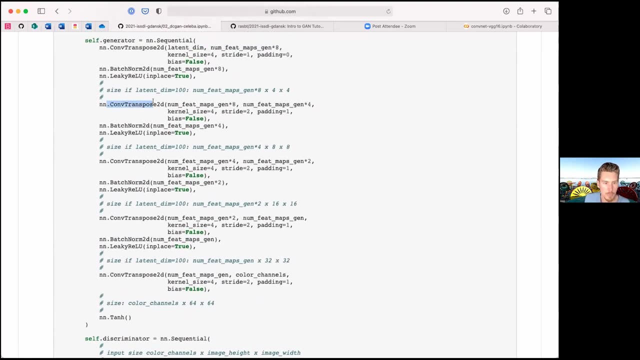 So I'm using, for the discriminator here, convolutional layers, CONF2D, Again still using Leaky ReLU. I'm also using BatchNorm because it helps with the training and you have multiple layers here, And for the generator I'm using the CONF transpose layer. 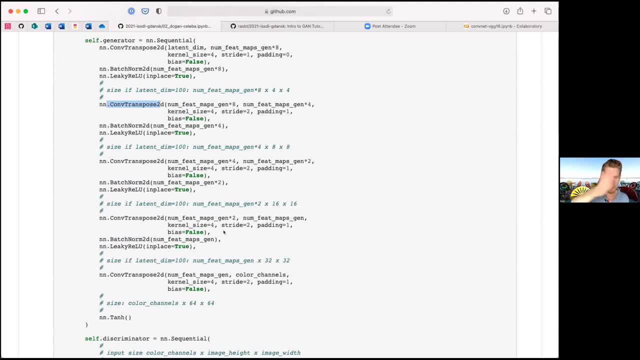 It's essentially doing the opposite of a convolution layer. instead of going from a larger image to a smaller image. If you use the large stride, it would make the image larger. It's like going backwards. almost Okay, yeah, and this is it. 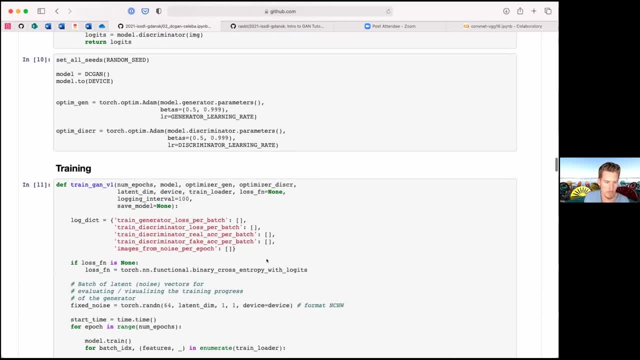 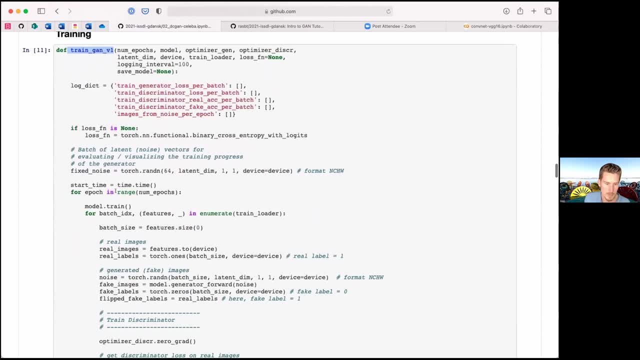 So if you run this code, it should work like before. In fact, this function here is exactly the same training function I used before. I just copy and pasted it here. So there's no change here. It's exactly the same function. 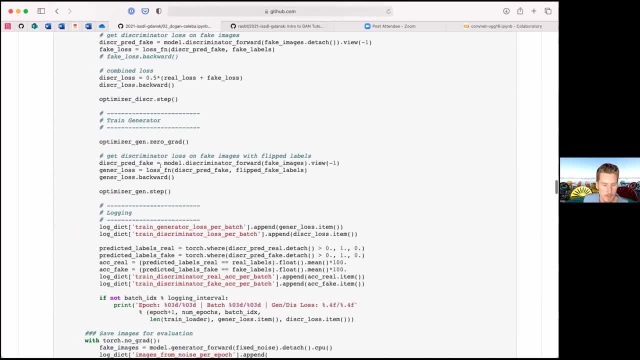 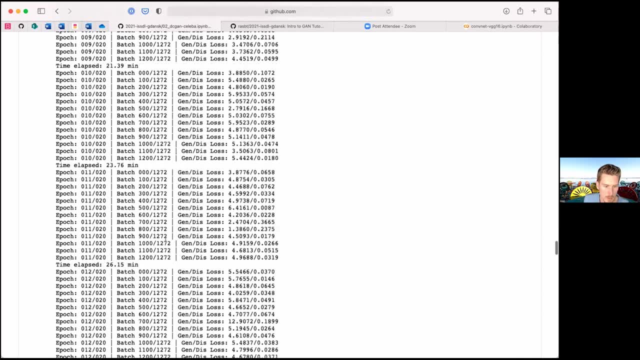 And also the solution to your exercises here with the labels. And this takes a little bit of more time. to run a project like this, It takes approximately two and a half minutes per epoch And I only trained it for 20 epochs because it took a long time, almost an hour. 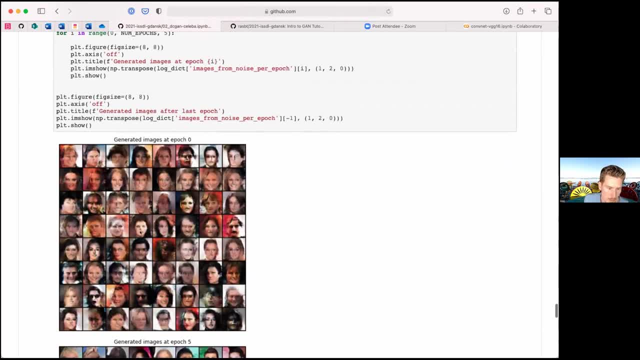 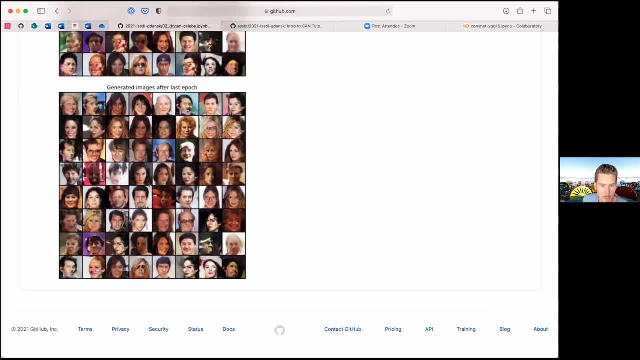 And you can see it starts with relatively bad images And then the face images become more realistic over time. So this is after the last epoch. Of course they're not perfect. It's a simple DCGAN. It's still a very simple GAN method. 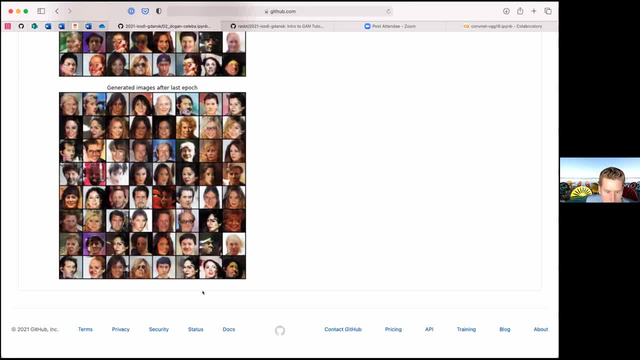 But you can see maybe this person or this person. They kind of look like almost realistic face images, So they're not too bad. So this person looks very realistic. Two minutes, OK. So I will wrap it up now. So if you are interested in GANs. 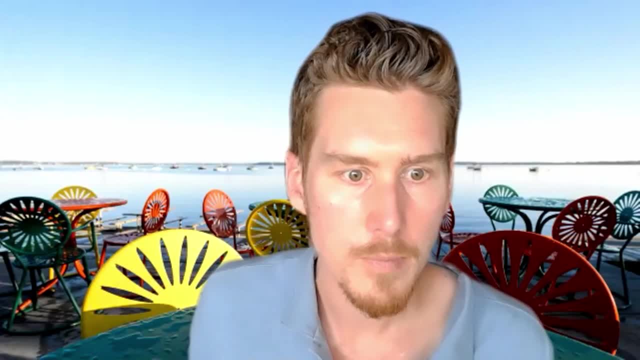 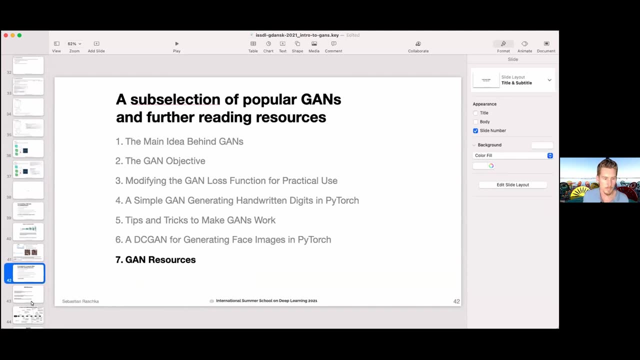 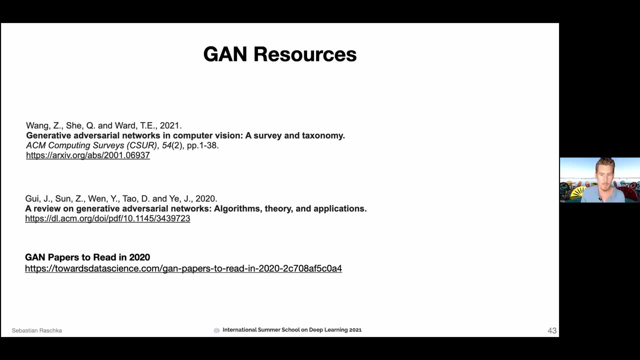 let me just one more time share my slides. If you are interested in GANs, I have some resources here for you. So full screen. So of course, there are hundreds, if not thousands, of GAN papers out there. So I would say these are. 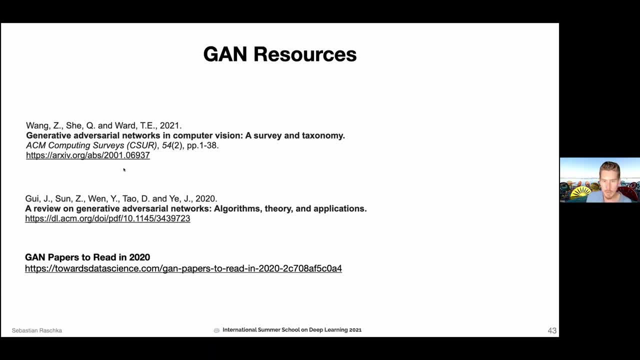 Good ones to start nowadays. They are very, very recent And one focused really on computer vision. The other one is also kind of focused on computer vision. But these are nice survey papers. They are approximately 40,, 30, 40 pages. 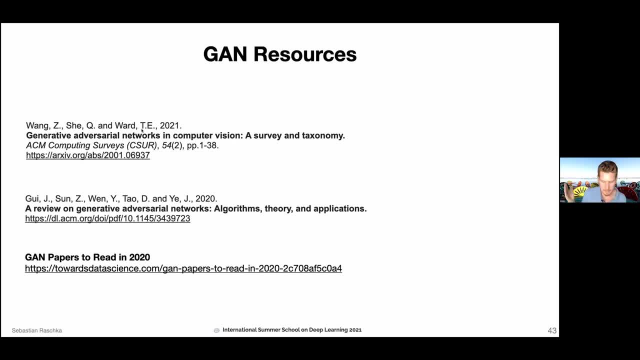 So they have a lot of information, But they are really just highlighting what are the current GANs that are currently used, And this is, I think, a nice resource if you want to learn about the cutting edge GANs. So what I gave you was an introduction. 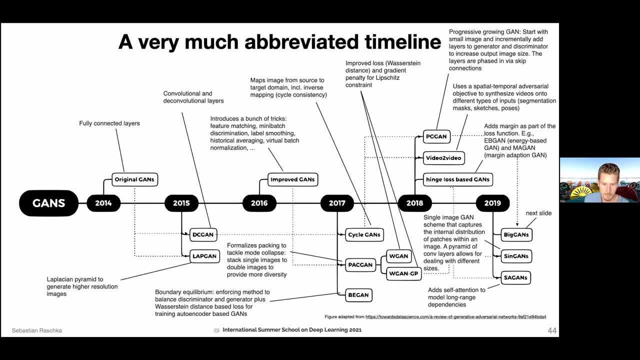 And with that you can also catch up with the latest GANs. Here is a figure I created based on a figure I found on the internet. I just annotated it with some sentences describing these methods, So this is like a selection of methods. 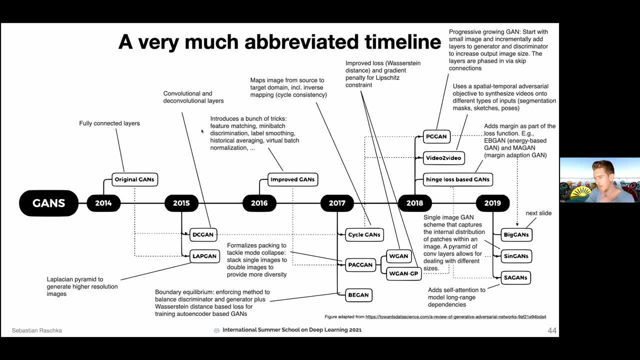 that have kind of shaped the development of GANs. Of course, there are many more influential methods. For example, this also stops in 2019.. So the alias free GAN is not on there. Style GAN is not on there. 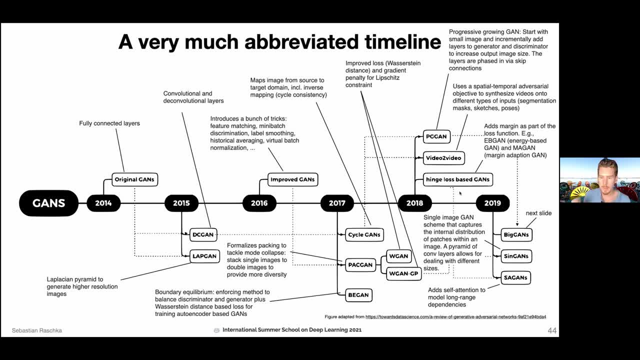 But many other important GANs are on there. In my other talk on Thursday, I will talk, for example, a method that is based on this. It's called the cycle GAN here, which is something that can be used for something called. 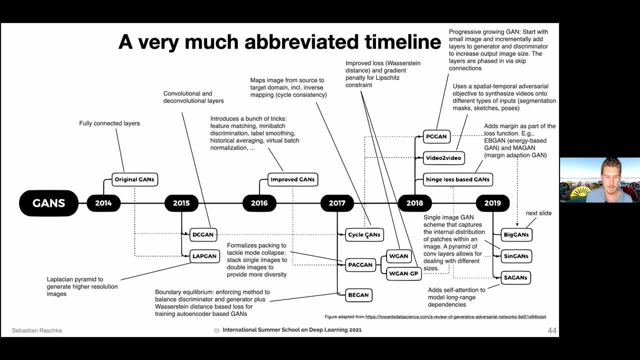 the neural style transfer. OK, so yeah, this is also if you want to learn really about the individual steps and history of GANs. this is like a good summary of different GANs maybe you want to learn about. This is the big GAN which is currently very popular. 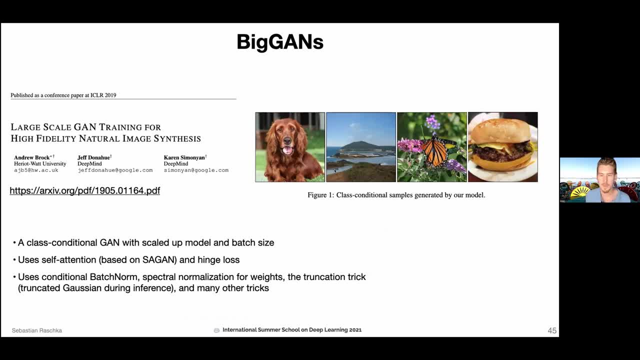 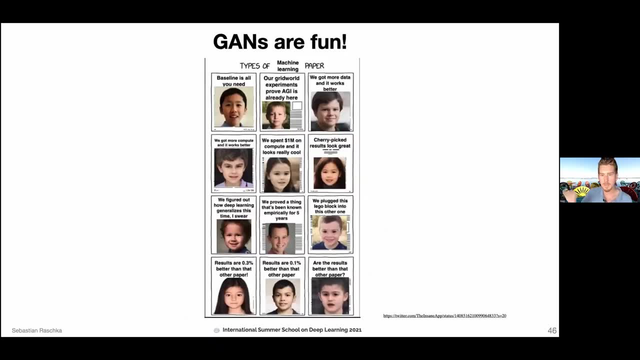 And you can see the images look super good if you compare it to what we trained. But of course this would require way more resources that we have used. OK Yeah, So with that, I just want to say GANs are fun. 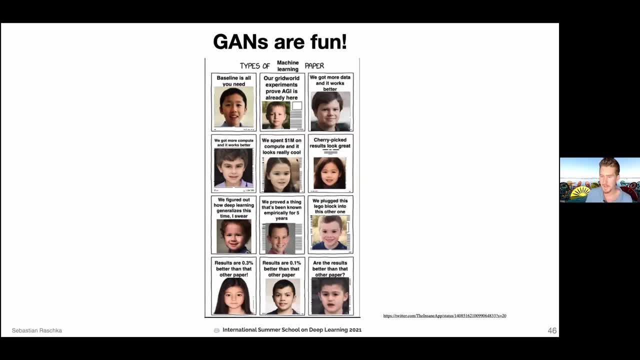 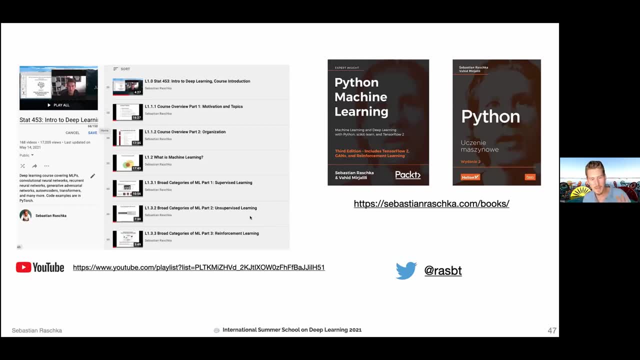 You can do lots of interesting things. So this was just a fun thing I saw the other day on Twitter And with that, yeah, just briefly. if you are also interested, I have some lectures on YouTube also, including GANs. It's actually a whole deep learning course.